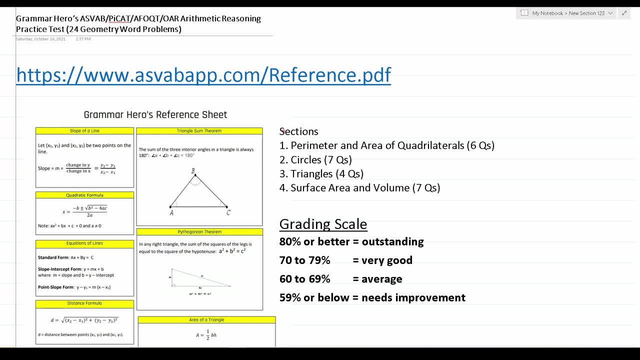 all these word problems in today's video And, as you can see, these word problems are going to be broken down into various sections. There are going to be six questions about perimeter and area of quadrilaterals. There are going to be seven questions about circles. 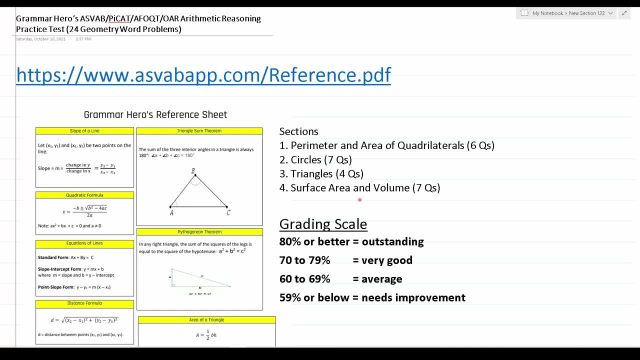 Four questions about triangles and seven questions about surface area and volume. Finally, I want to say this: typically after I post a video like this, I notice that quite a few of these paid tutors will start going through my videos and creating almost identical content. In light of the fact that that's happening, I don't encourage you to pay for tutoring whatsoever. 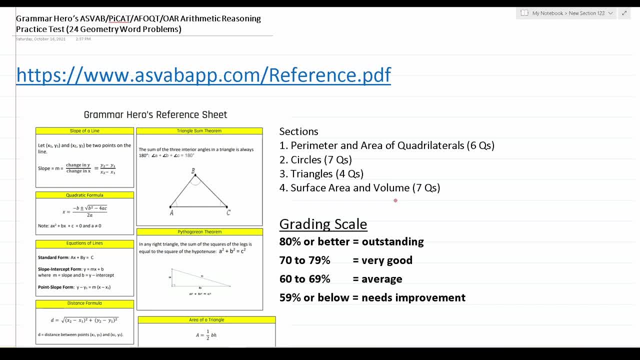 This video has almost everything you need to know about geometry to be successful on any of these standardized tests. So, with all that being said, let's go ahead and get started with today's video. All right, so this first question says if a parallelogram has 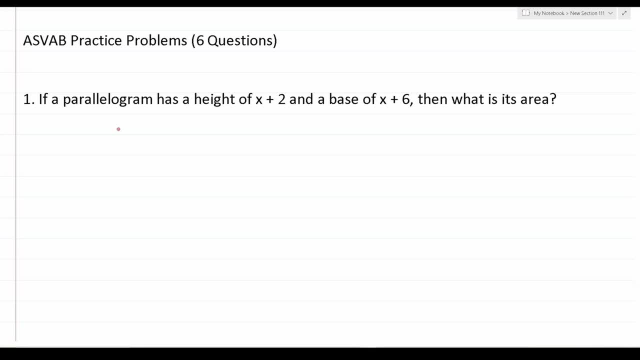 a height of x plus 2 and a base of x plus 6, then what is its area? Well, we should know that to find the area of a parallelogram, we simply multiply our base by our height and, as it happens, we were given both of those things. We were told the. 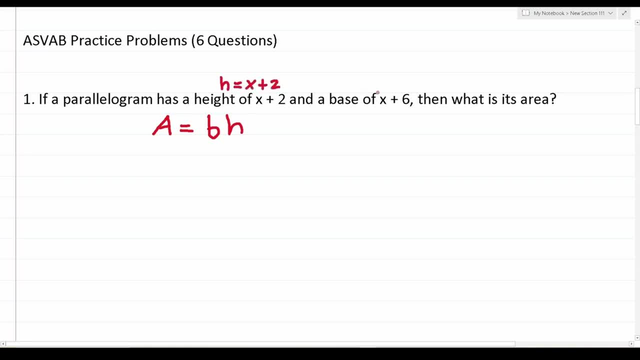 height of this parallelogram is x plus 2.. Similarly, we were told that its base was x plus 6.. So let's plug those values into our formula. accordingly, This becomes area equals again base. So this becomes x plus 6 times x plus 2, which was our height. All right, so one of the challenging 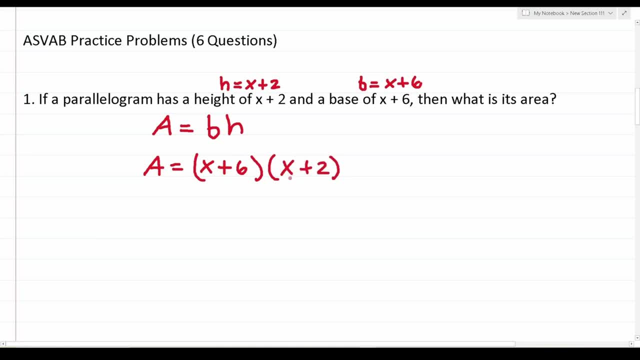 aspects of the ASVAB is it will take a lot of simple principles and combine them into one problem. So in this case, to start we had to know how to find the area of a parallelogram. but now we actually have to know how to apply the area of a parallelogram, So we have to. 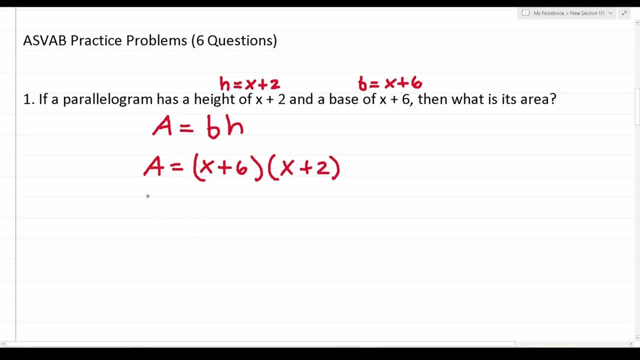 take the distributive property to multiply these two polynomials together, And what we're going to do in this case is we're going to take this x, we're going to multiply it by this term, as well as this term. Then we're going to take this 6, according to the distributive property, We're 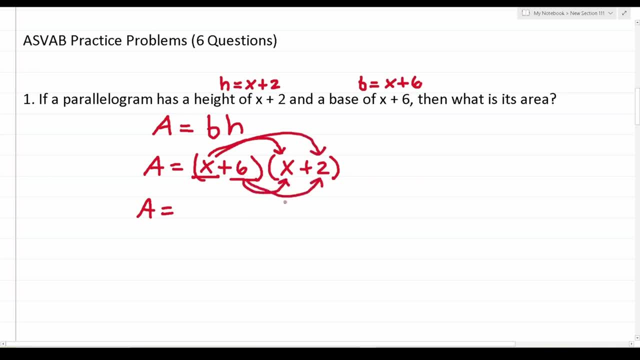 going to multiply it by this term and then this term. So let's go ahead and work on doing that. As you can see, to start we have x times x, which is going to be x squared. Then we have x times 2, which is 2x. 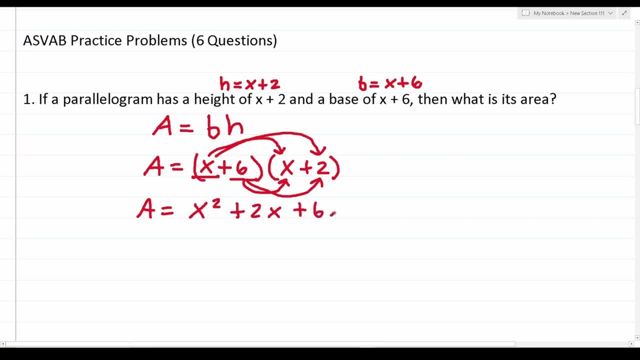 Then we have x times 6, which is 6x, And then we have 6 times 2, which is 12.. Of course, we can combine like terms. now, Notably we can combine 2x and 6x to be 8x. All right, so to answer this, 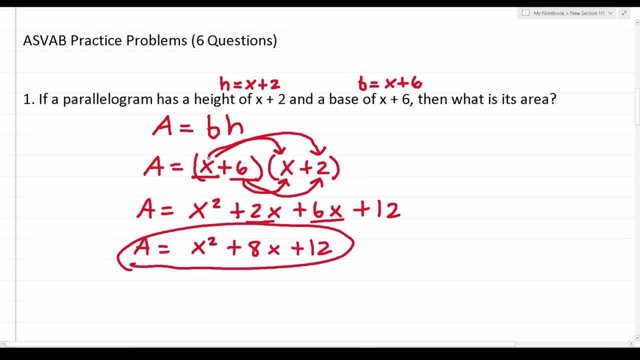 question. the area of this parallelogram that has a height of x plus 2 and a base of x plus 6 is x squared plus 8x plus 12.. All right, again we have to use our knowledge of how to find the area of a parallelogram. 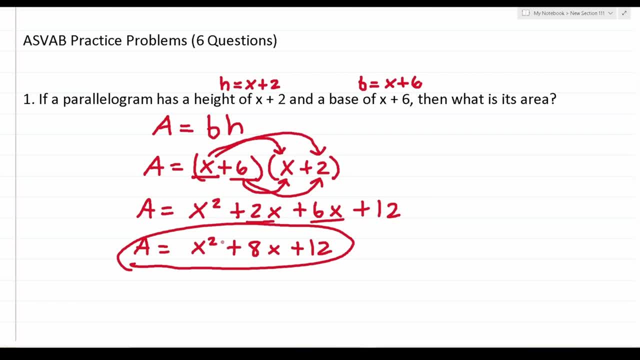 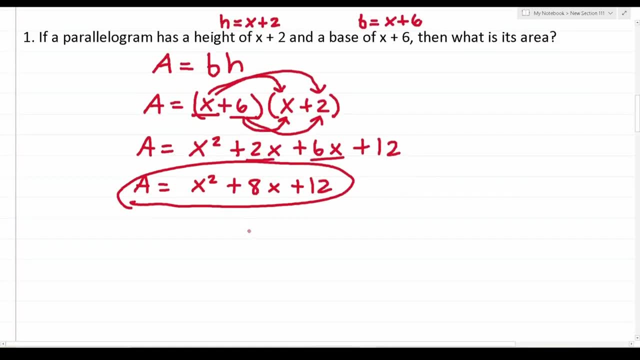 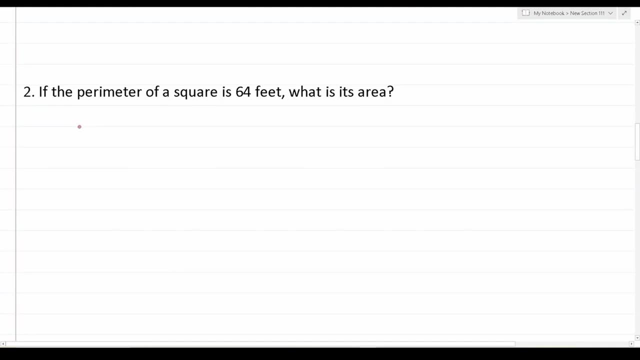 as well as our ability to multiply polynomials together in order to solve this one. All right, so that's a very good practice problem there. All right, so number two says: if the perimeter of a square is 64 feet, then what is its area? All right, so we know we're working with the square. 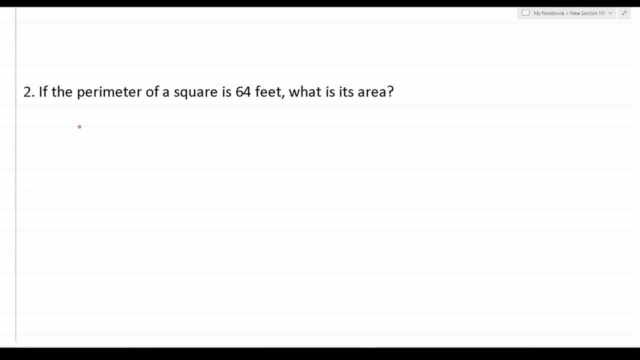 but this problem is challenging Because it's saying something. It's saying: if I give you the perimeter of this square, there must be a way for you to find its area. So that is the crux of this problem. Let's see how we're going to do that. When problems get slightly more challenging, I always like to sketch. 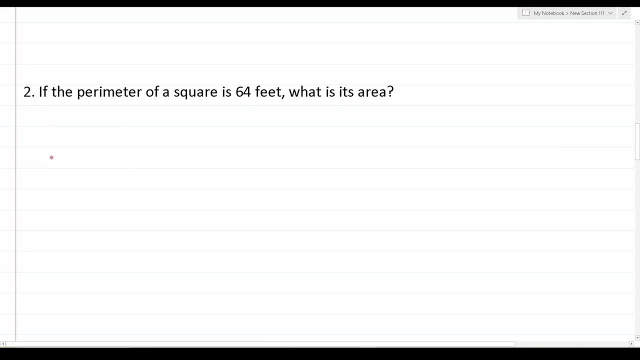 things out. So in this case, I'm going to start by making a square here. In fact, I'm going to make two squares, But to start, I'm just going to make one here And again, one of the properties I mentioned about squares is that they all have a square, So I'm going to make a square here. 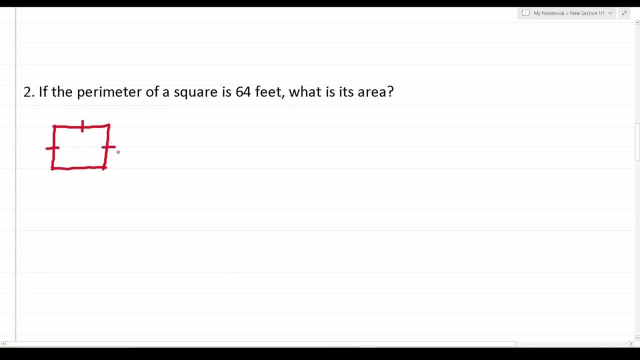 They all have equal sides. So this side is equal to this side, This side is equal to that side and that side is equal to that side. How would I find the perimeter of this square? Well, again, if you recall from when we reviewed the formulas, our unknown side here we labeled: 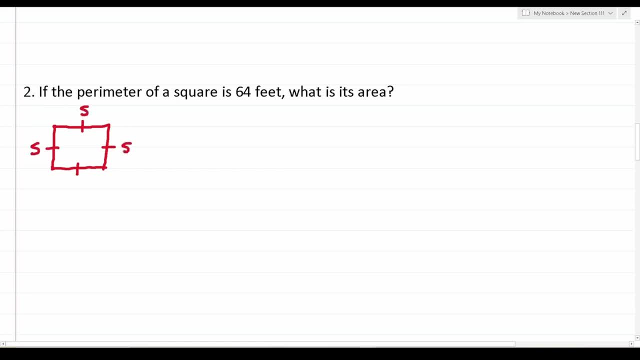 S, And if that side is S, this side is S, this side is S and this side is S. To find the perimeter of any quadrilateral, we just add up all the sides, So we're going to go perimeter of this square. 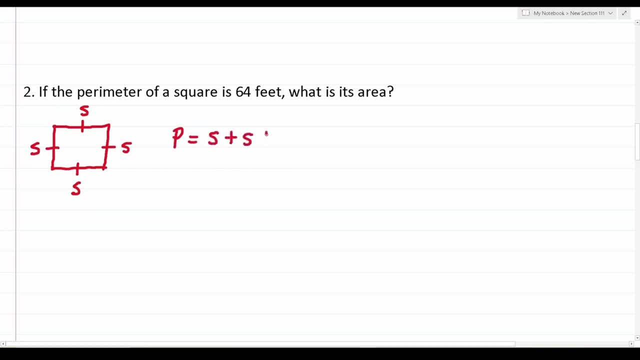 for the time being is going to be S plus S plus S plus S. That said, this problem told us what P is. It says the perimeter of this square is 64 feet. In other words, we know what P is. So, instead of 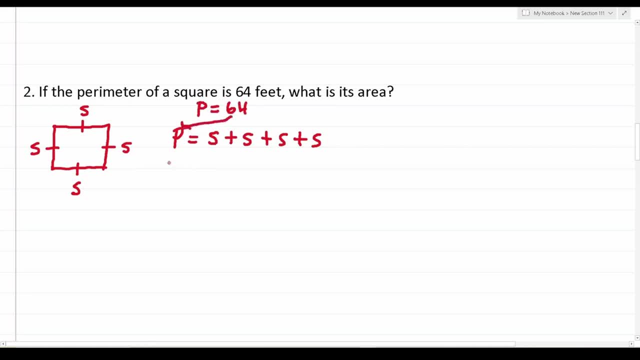 having P here we can actually plug in 64. So this becomes: 64 equals S plus S plus S plus S, And let's combine these S's to be one term. So this is: 64 equals S plus S is 2S plus S is 3S. 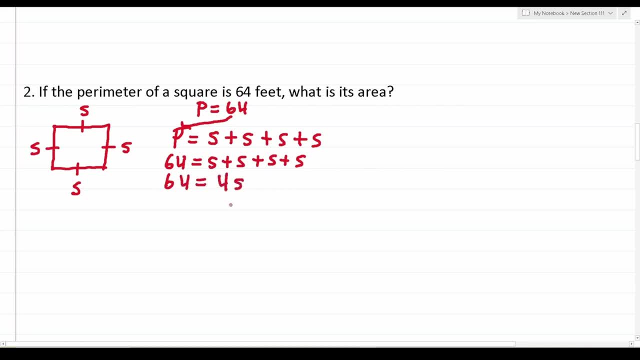 plus S is 4S. All right, Now let's divide both sides by 4 to get S by itself, And again S will tell us how long each of these sides is. So let's divide both sides by 4. next, 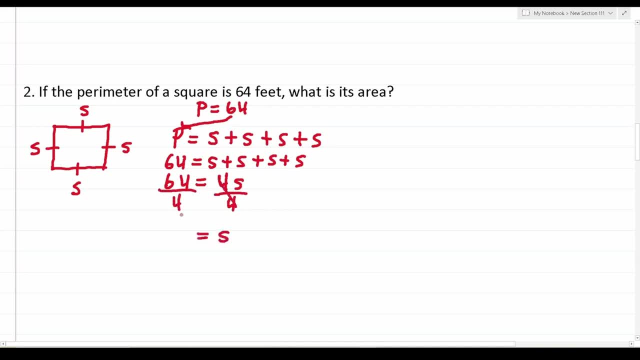 This crosses out, leaving you with S on this side, 64 divided by 4.. If you can't do that in your head, you're going to have to do it off to the side And you're going to have to do long division. So 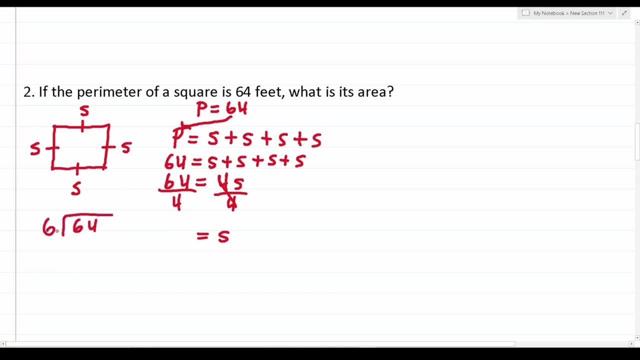 this is 64 divided by 4.. All right, And we start by asking ourselves: how many times does 4 go into 6 without going over? That's going to be one time, Given that 1 times 4 is 4.. 6 minus 4 is 2.. And 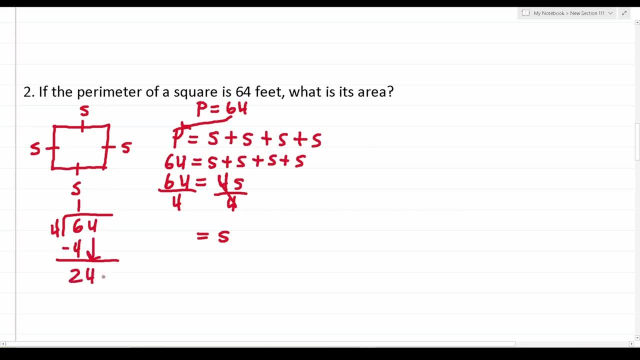 now we drop down this 4.. Now the question is: how many times does 4 go into 24? 24, without going over, That's going to be 6 times 4 times 6,, you should know, is 24.. So there's no. 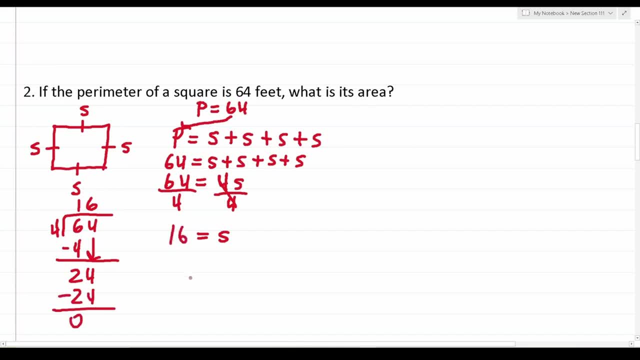 remainder, So S is 16 in this case, And in math we actually write the variable on the left. So this is S equals 16.. Well, you might be saying to yourself: how is that going to help me find the area of this square? Well, let's go ahead and make another square, if it's helpful. 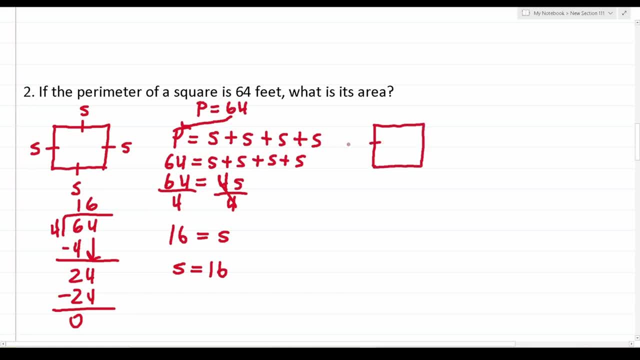 Again, we now know that this square has sides, Side lengths of 16.. All right, And how do you find the area of a square? Again, it's always S times S, And we know what those sides are. It's 16 by 16.. So this becomes 16 times 16.. 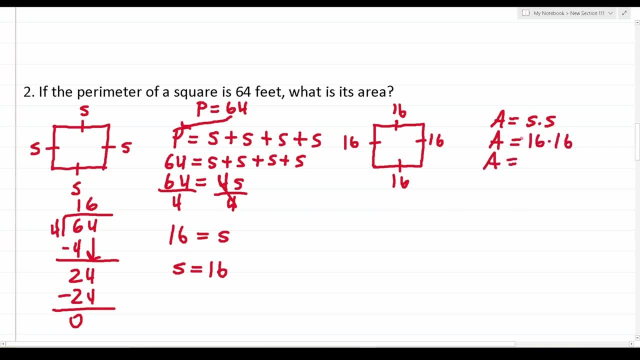 And if you don't want to make a mistake by doing this mental math wrong, you can go ahead and do the multiplication off to the side. 6 times 6 is 36.. So we drop down a 6 and carry a 3.. 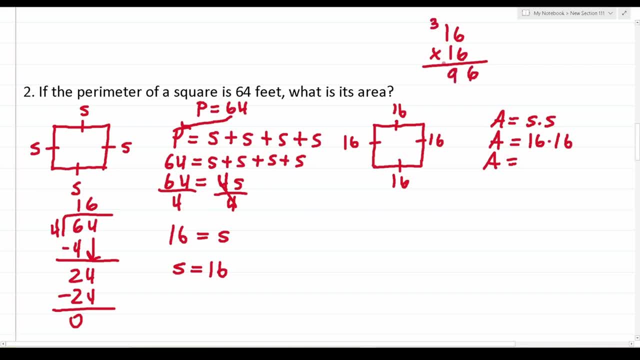 1 times 6 is 6 plus 3 is 9.. Before we start multiplication with this 1, we have to bring in a 0 placeholder. 1 times 6 is 6.. 1 times 1 is 1.. Let's add these together now. 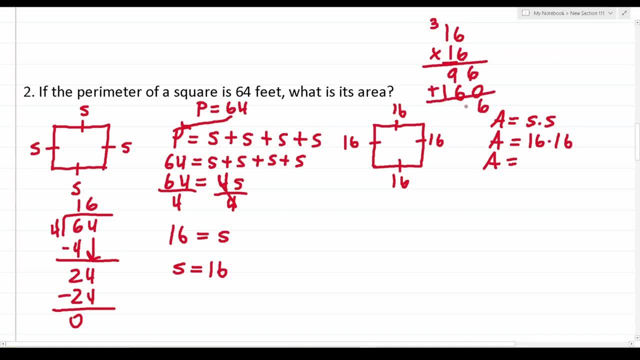 6 plus 0 is 6.. 9 plus 6 is going to be 15.. So drop down a 5 and carry a 1.. 1 plus 1 is 2.. So the area of this square is going to be 256.. 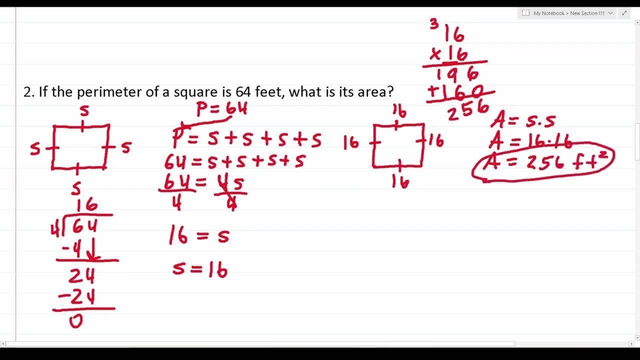 So the area of this square is going to be 265.. This is the area where S becomes 6. And that is the answer to this: 1. Again for the ASVAB, and as far as squares go, You have to realize that. 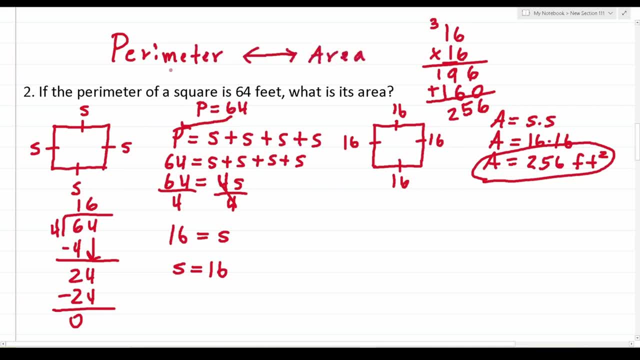 perimeter and area occupy a two-way street. That is to say, if I give you the perimeter of a square, you should be able to find its area. you should also be able to find its perimeter. Again, those occupy a two-way street. 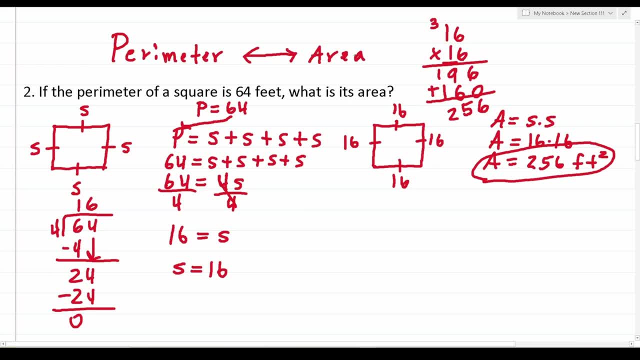 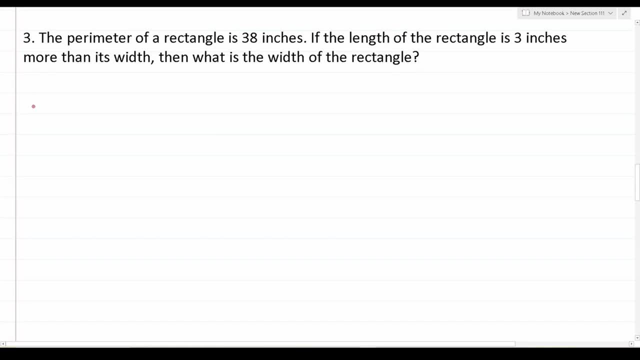 All right. so that's a good example of that one. All right. so number three here says the perimeter of a rectangle is 38 inches. If the length of a rectangle is three inches more than its width, what is the width of the rectangle? 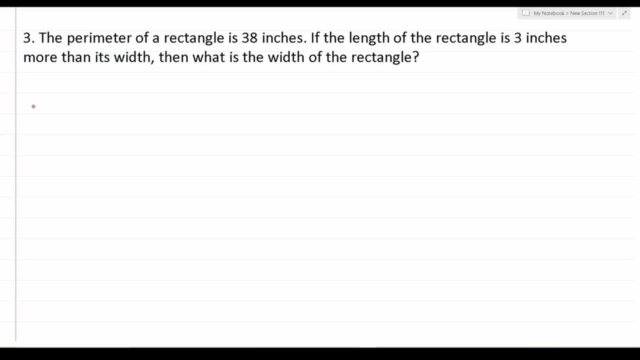 All right, so we're working with a rectangle. This problem seems somewhat challenging at first, so first thing I'm going to do is quickly sketch a rectangle here And again. we should know some properties of rectangles, notably that this width is equal to. 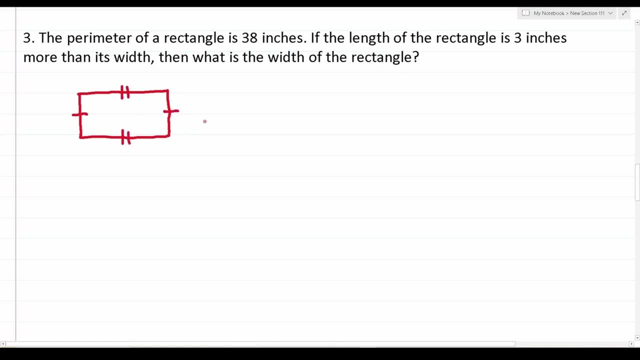 this width and this length is equal to this length. Additionally, we were told that this rectangle had a perimeter of 38 inches, so I'm going to say p equals 38.. What's more, we were told that the length of the rectangle is 38 inches, So we're going to say p equals 38 inches. 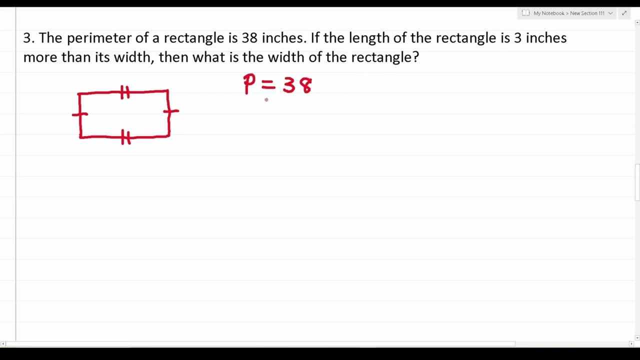 The length of the rectangle is three more inches than its width. Okay, so we don't know how wide it is, so I'm going to call it x inches wide, And if its length is three more inches than its width, that means its length is x plus three. All right. likewise, we know if this width is x. 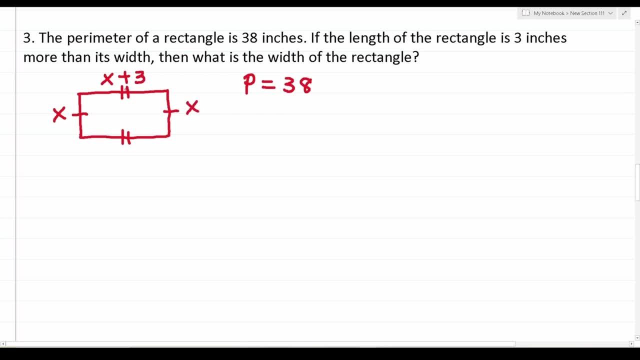 this side's also going to be x, And if this length is x plus three, that means this length is going to be x plus three. All right, how do we find the perimeter of a rectangle? We just add up all of its sides. So 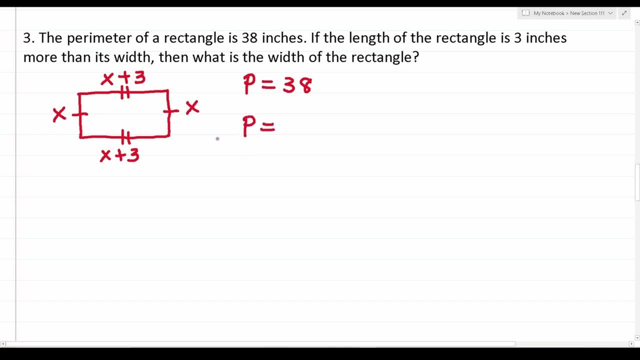 I'm going to add this x, this x plus three, this x and this x plus three together. So that's going to look like this x plus x plus three plus x plus x plus three And, if it's helpful, you can see. 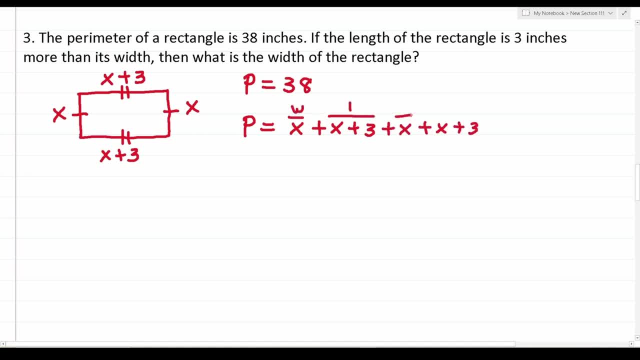 that this is the width. this is one of the lengths, this is another width and this is another length. All right, so let's go ahead, Add these together, Let's combine all of our x's. We have x, x, x and x. We have four x's. 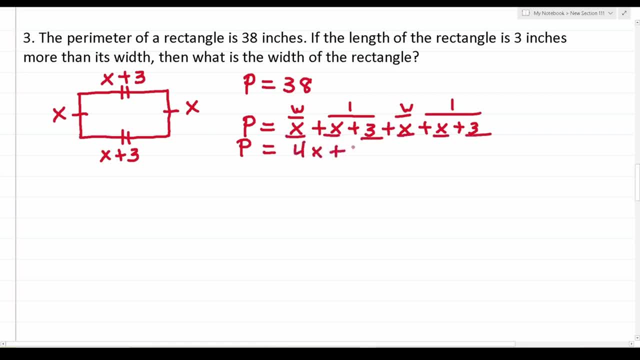 and then we have three and three, So we just have plus six. Again we were told what p is. P is 38. So in place of p here I'm going to put 38. This becomes: 38 equals four x plus six. 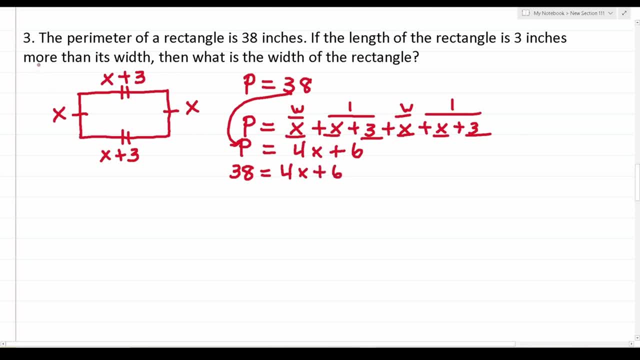 All right, and we should see that if we solve for x, we'll know the width of this rectangle. Because here look, x is the width of this rectangle. So our goal here is to solve for x. Let's start by subtracting six from both sides. This crosses out here: 38 minus six is going to be. 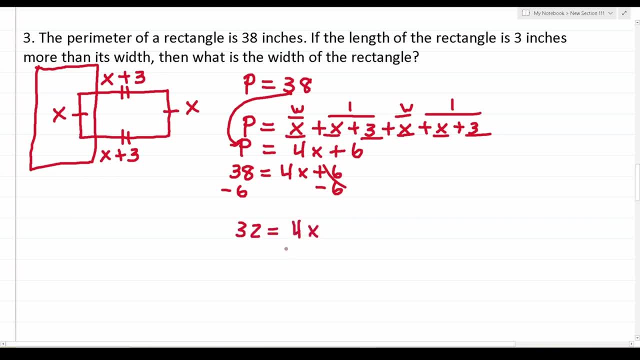 32.. So this is 32 equals four x. Let's divide both sides by four now to get x. by itself, This crosses out, leaving you with x equals 32, divided by four is eight, So x equals eight in this case. 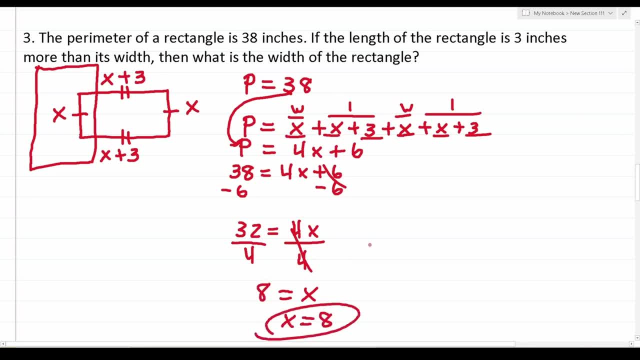 In other words, the width of this rectangle is eight inches. Again, x corresponds to the width of this rectangle, So x is eight. We know its width is eight, All right. so the challenging part of this problem was you had to use some basic algebra as well as your knowledge of how to find. 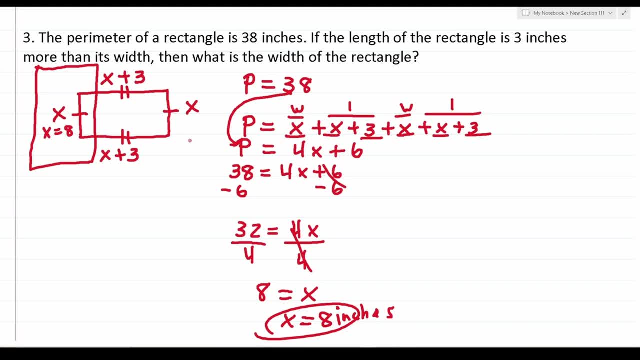 the perimeter of a quadrilateral, notably a rectangle, in order to solve this one. So again, you should see a pattern. We're combining two basic concepts into one: some basic algebra and some basic knowledge of geometry, And that's what makes the ASVAB difficult. All right, so let's go ahead and move on to the fourth question now. 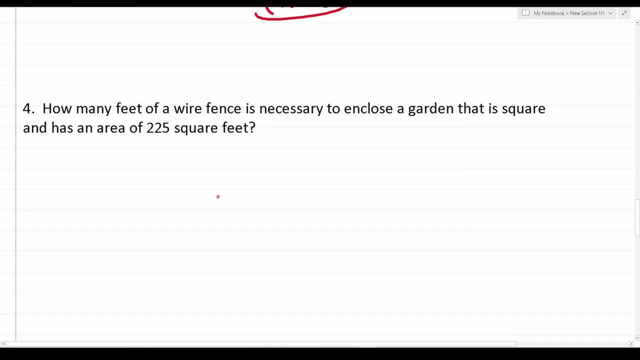 All right. so number four here says how many feet of a wire fence is necessary to enclose a garden that is square and has an area of 225 square feet. All right. so, while it may not be obvious at first glance, this is a problem. 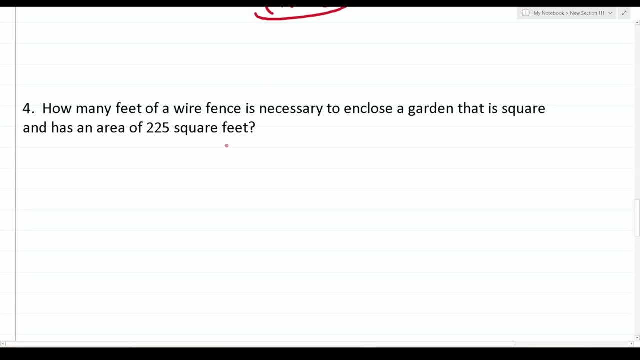 Testing your understanding of the relationship between the area and perimeter of squares. And, as I said previously, perimeter and area live on a two-way street, That is to say, if you're given the perimeter of a square, you can find its area. Likewise, if you're given the area of a square, 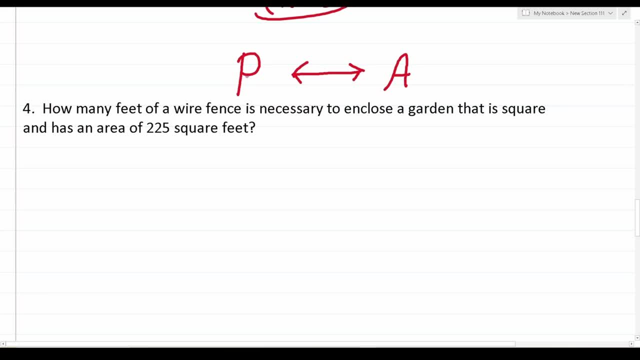 you can find its perimeter. So in a previous problem we went from perimeter to area. In this problem we're going to be going from area back down to perimeter, So let's see what that looks like. All right, first things first. I'm going to start this one by making a quick sketch, And we 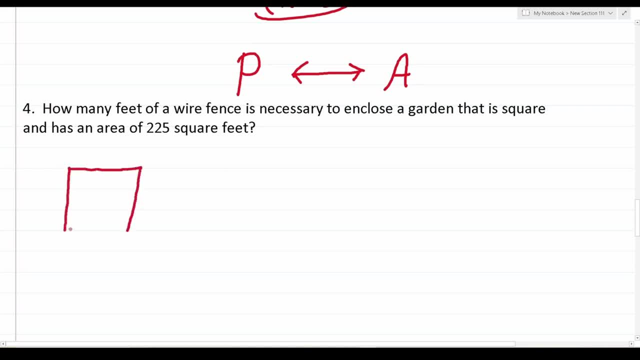 know we're working with the square in this case, so let's quickly make one of those as best we can here, And one of the properties of squares that we should know is that all the sides are equal. This side's equal to this side, that side's equal to that side and that side's equal to that side. 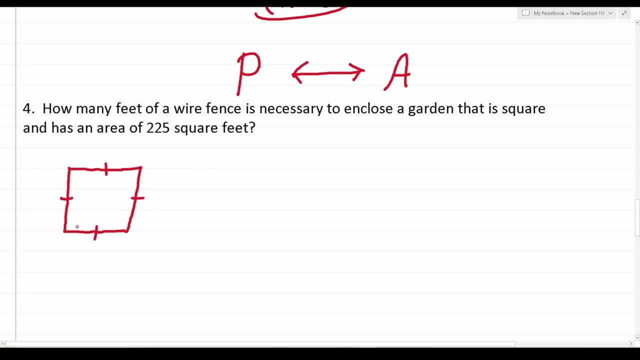 You may recall that if we don't know how long these sides are, we can call them s, And if that side's s, this side's s, this side's s and this side's s, All right. so let's start with finding the area of this square. We know what its area is, According. 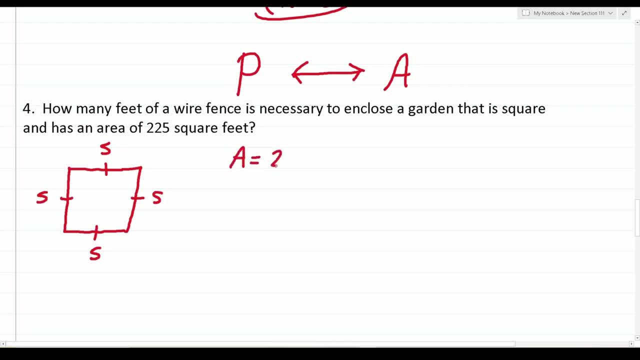 to the problem. this square has an area of 225 square feet And I'm going to drop off that square feet since we're just doing some math here. How do you find the area of a square? Remember, area of a square is s times s. 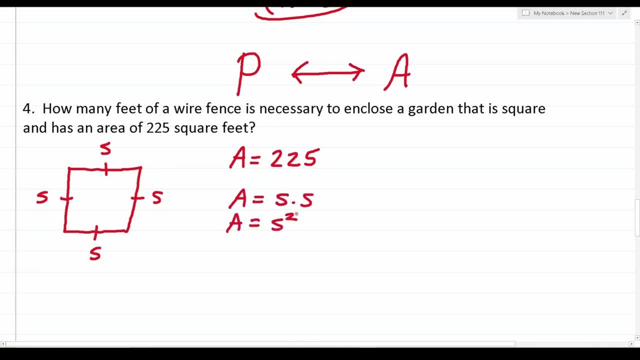 which is the same thing as s squared Again s times. s is s squared. Well, we know what our area is. according to the problem, It's 225.. So, in place of a here, I'm going to plug in 225.. This becomes: 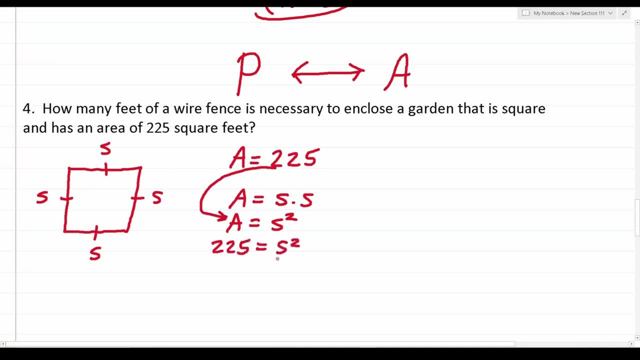 225 equals s squared. And now we should see that if I solve for s, I'll know how long the sides of this square is All right. So in order to solve for s, we're actually going to need to find the area of 225.. So we're going to have to take the square root of both sides here. This will cross. 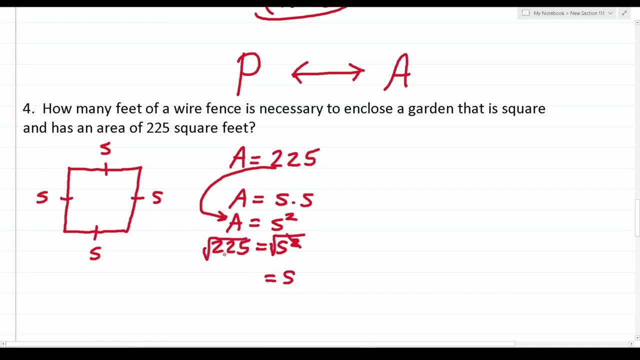 out this square here, leaving you with just s on this side. What is the square root of 225?? You should know this one: It's going to be 15.. So s in this case is 15.. All right Again. 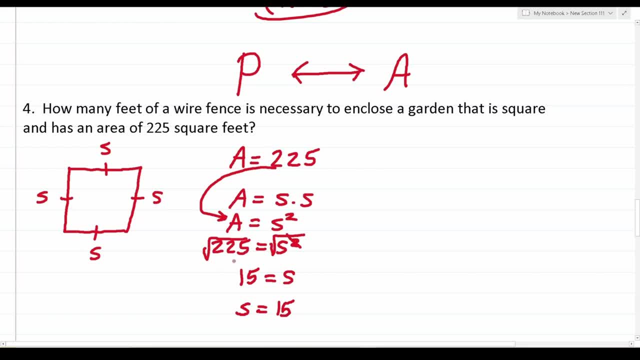 on my formula sheet on my website, I have a list of perfect squares that you should memorize, 1 through 20.. And you should know that the square root of 225 is going to be 15.. All right, So now we know we're working with a square garden that has sides that measure 15,. 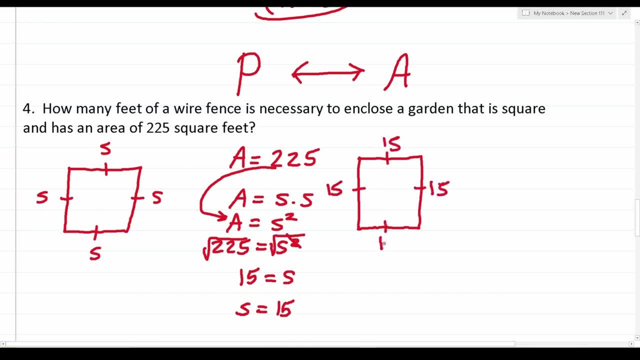 15,, 15, and 15.. And the question is: how many feet of wire fence is necessary to enclose this garden? Well, from here to here, this section of the fence is 15 feet. From here to here is 15 feet. 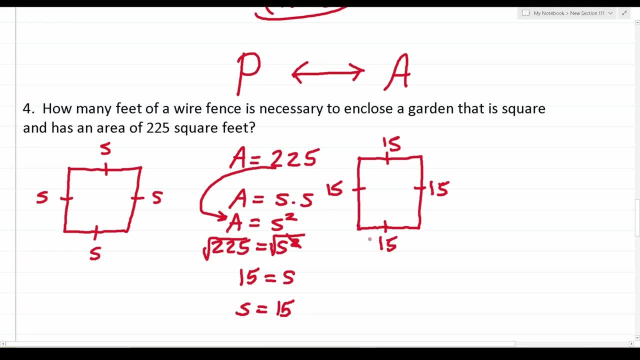 From here to here is 15 feet, And from here to here is 15 feet. In other words, in order to solve for s, we're going to have to take the square root of 225.. So we're going to find out how much feet we need to enclose this garden. We're going to be finding the perimeter. 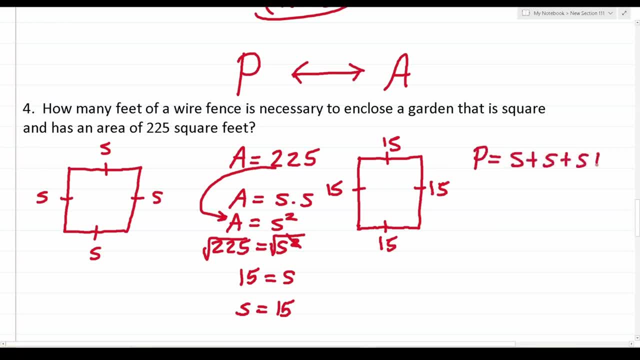 of this garden, which is s plus s, plus s plus s, And we know what all those values are. They're 15 plus 15 plus 15 plus 15.. And you should be able to do this one mentally. We have 15 and 15, and 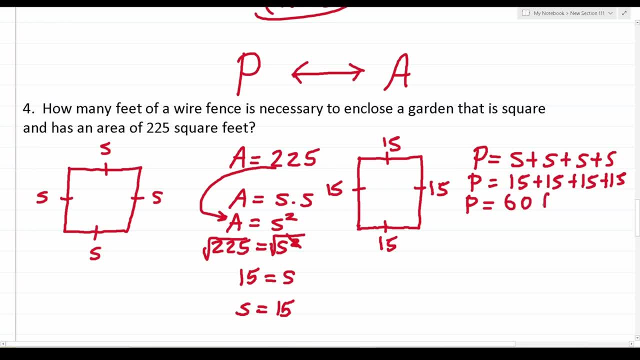 15 and 15.. This is 30 plus 30,, which is 60. So you're going to need 60 feet of wire fence to enclose a garden that has an area of 225 square feet. Again, you have to understand that. 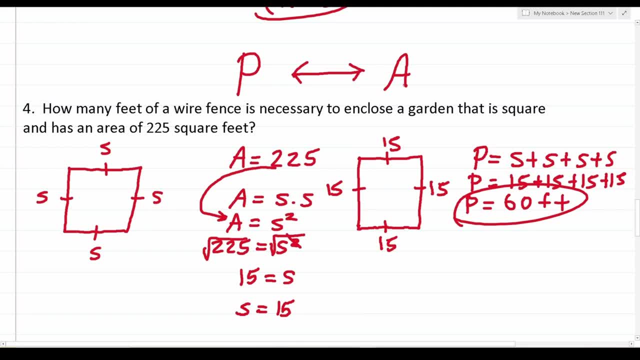 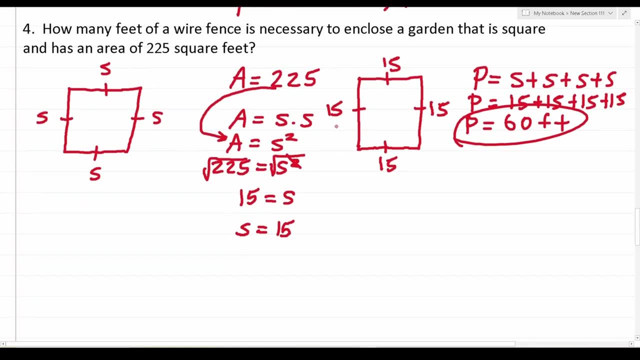 for squares at least. if you're given the perimeter, you can find the area. If you're given the area, you can find the perimeter, All right. so that's that one, All right. so number five says what is the length of the diagonal of a rectangle? that 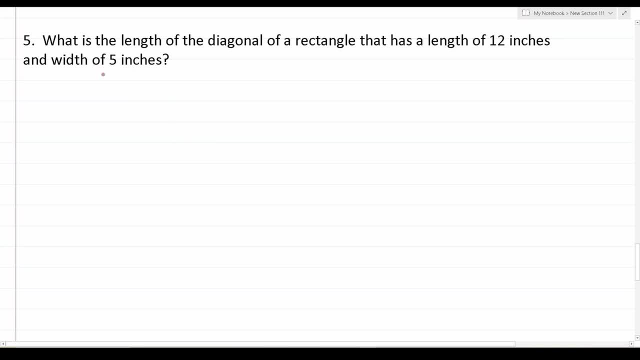 has a length of 12 inches and a width of five inches. So for this problem, we know we're working with a rectangle, So let's quickly sketch one of those. And we should know some properties of rectangles, Notably, this width is equal to this width. 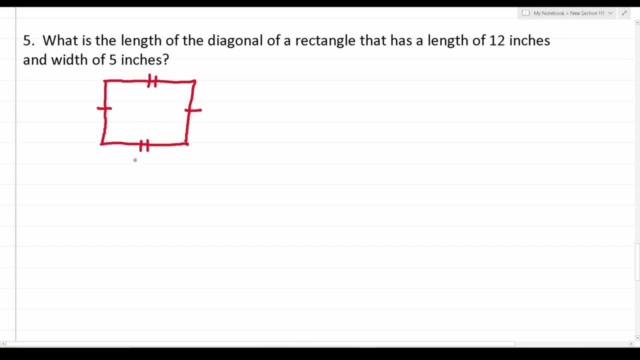 and this length is going to be equal to this length. And we're told what those values are. We're told that this rectangle has a length of 12.. So this is 12, and this is also 12, and a width of five. So this is five. 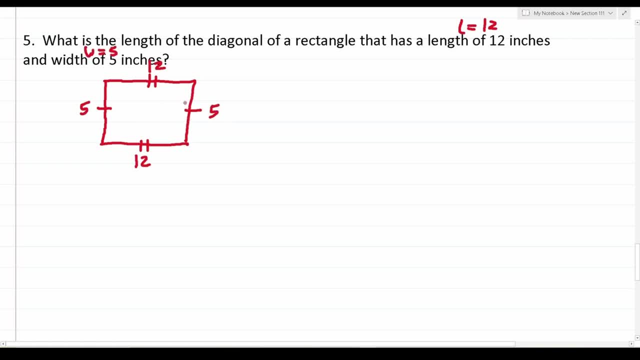 and this is five. What's more, the problem's asking us to find the length of the diagonal of our rectangle. Well, what is the diagonal of our rectangle? It's the distance from here to here. That is, we're slicing this rectangle in half. And when we slice a rectangle in half, 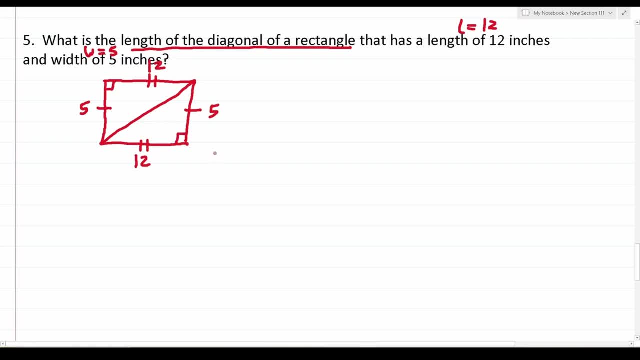 we get two right triangles, All right. so the question is, how can we use this information about these right triangles to find the length of this diagonal? Well, let's pull one of those right triangles out. So I'm going to draw one of these right. 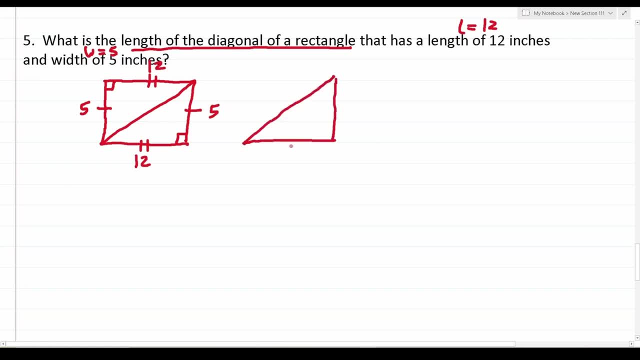 triangles off to the side here, And this is 12 here and this is five here. Here's our right angle, And we should know something about right triangles that's going to help us do this. Well, according to the Pythagorean theorem, if you're given legs of a right triangle, 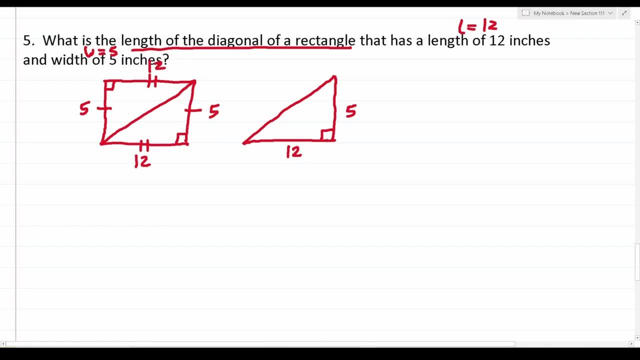 you can always find the length of its hypotenuse. And how do you identify its hypotenuse? Its hypotenuse is always directly across from its right angle. So this length right here is our hypotenuse and we can find it using the Pythagorean theorem And, as you can see, 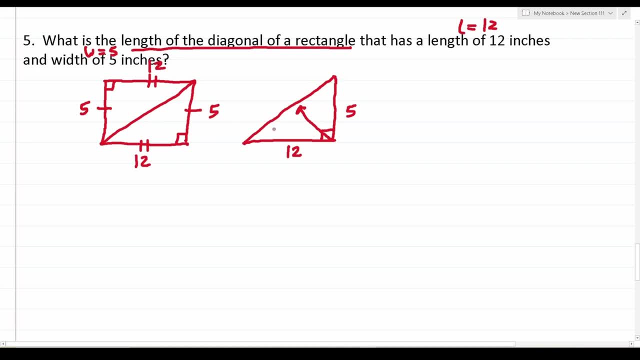 this length is this diagonal. So if we find the hypotenuse of this right triangle, we'll know the length of this diagonal. All right, so again, the Pythagorean theorem says: a squared plus b squared is equal to c squared, where a and b refer to the legs of your right triangle. 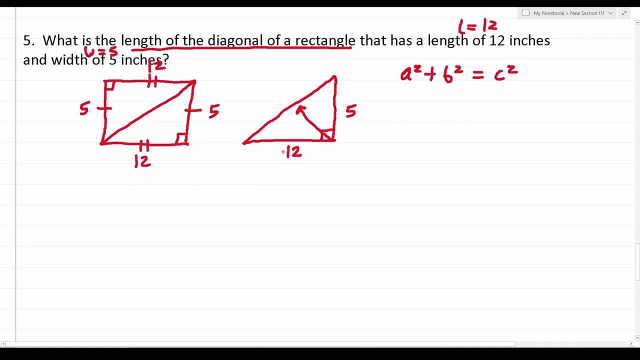 And c refers to your hypotenuse. So a is going to be 12,, b is going to be 5, and c is going to be the length of our hypotenuse. Let's go ahead and plug those values in accordingly. This becomes: 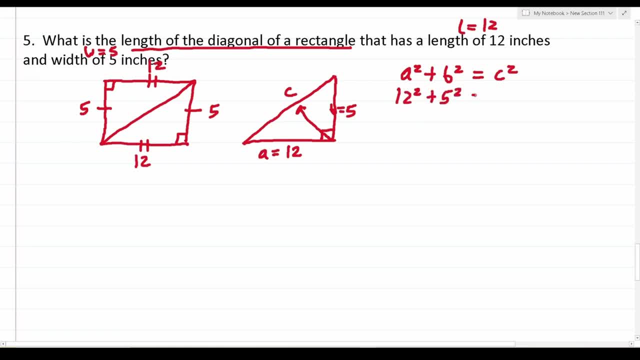 12 squared plus 5 squared equals c squared. We should know that 12 squared is going to be 144.. 5 squared is 25.. Of course, this equals c squared. Let's add these two together And we should know. 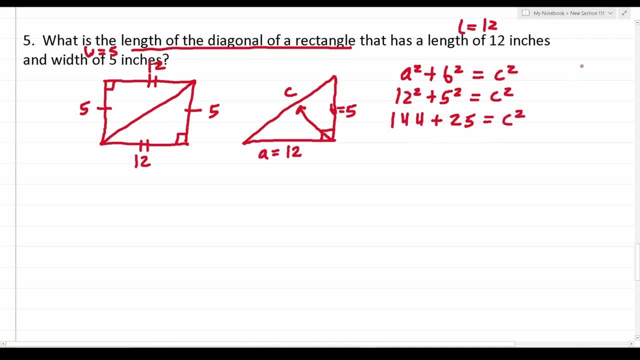 together And, so as not to make any mistakes, let's go ahead and add these together. off to the side, We have 144 plus 25.. 4 plus 5 is 9.. 4 plus 2 is 6. And 1 plus nothing is 1.. So this becomes: 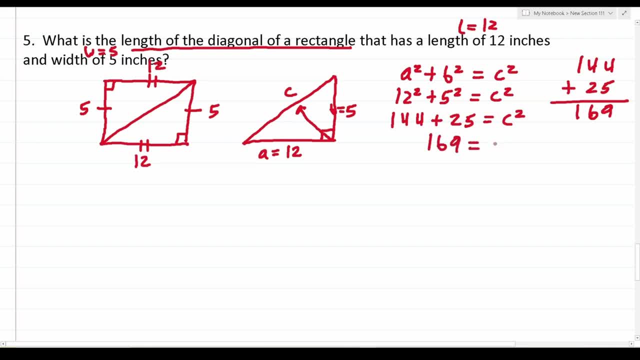 169 equals c squared. Again, we just want to know c, not c squared. So to get c by itself, we're going to think about this, So we're going to think about this, So we're going to think about the square root of both sides. This crosses out here, leaving you with just c on this side. What? 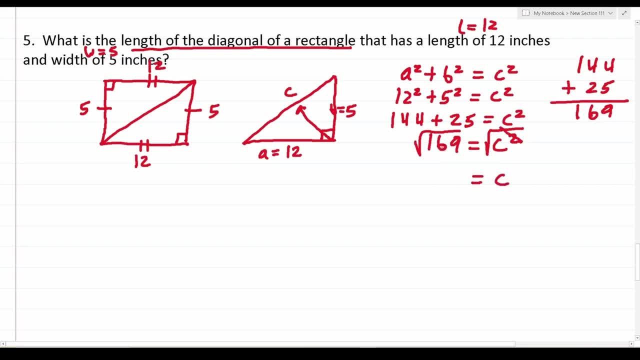 is the square root of 169?? It's on my reference sheet. You should be able to find it. It's going to be 13.. So c in this case is 13.. That means the length of our hypotenuse here is 13.. Likewise, 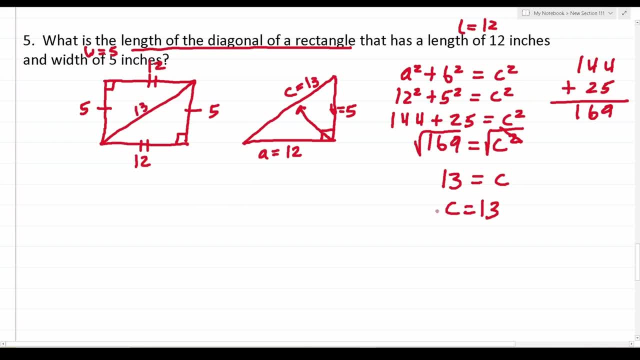 that tells us the length of our diagonal here is 13.. So to answer this question, the length of our diagonal is going to be 13 inches, All right. So again, I kind of threw this one in here, because sometimes your knowledge of rectangles is. 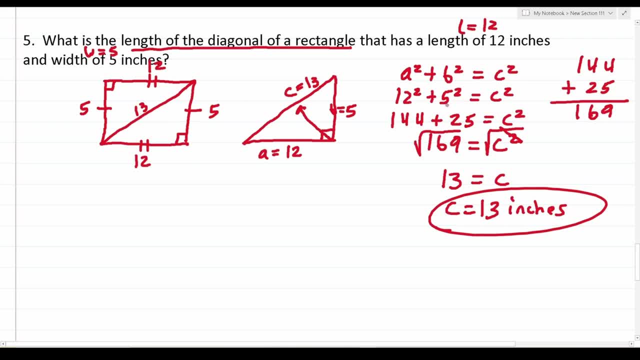 going to be combined with your knowledge of the Pythagorean theorem, which I've discussed in other videos. So again, the ASVAB likes to take two simple concepts and combine them into one problem, to make one challenging problem. And you've seen that for all the practice problems in this video. 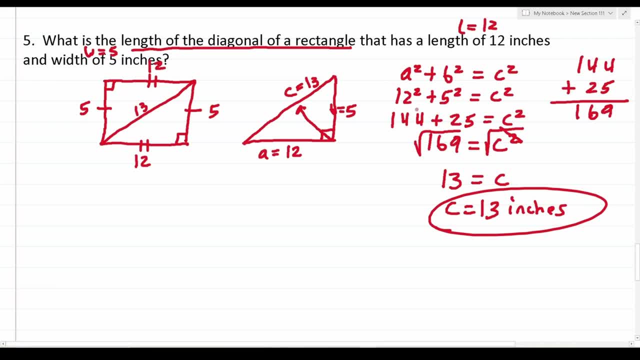 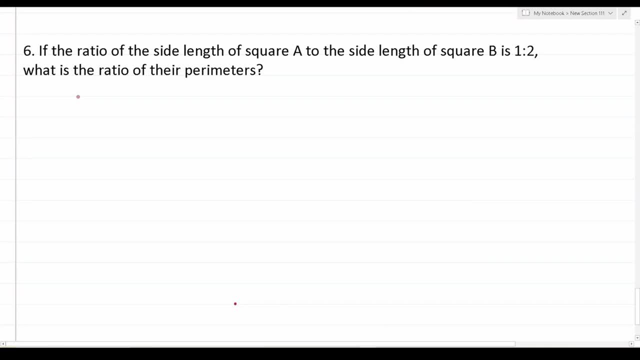 All right. So that's that one. Let's go ahead and move on to the final problem in this video. All right, So number six says: if the ratio of the side length of square A to the side length of square B is one to two, what is the ratio of their perimeters? All right, So for this one it should be pretty. 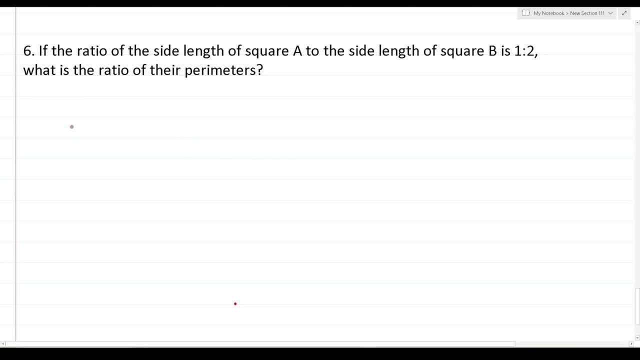 obvious that we're comparing two squares. We have one little square which I'm going to draw right here And I'm going to call this- let me fix that bottom part real quick. I'm going to call this square A And we're comparing that. 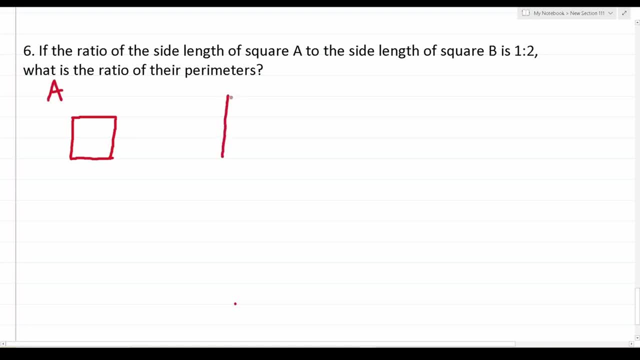 To a bigger square called square B, which I'm going to draw over here. This is square B. Again, the same properties about square still apply. This side's equal to this side, That side's equal to that side And that side's equal to that side. Likewise. 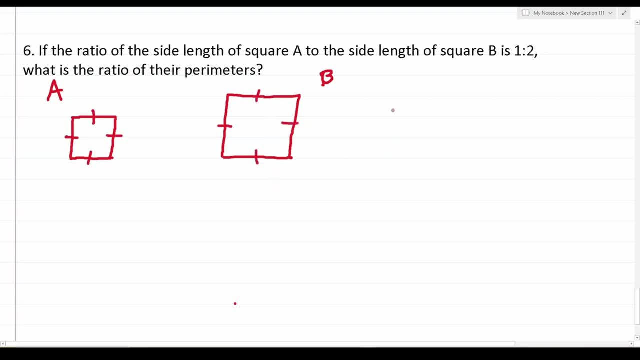 all these sides are equal too. We're told that the side length of square A to the side length of square B is one to two. So to me that means that we can let this side be one inch and this side be two inches. Again, if I were to ask you what the ratio of the side length of 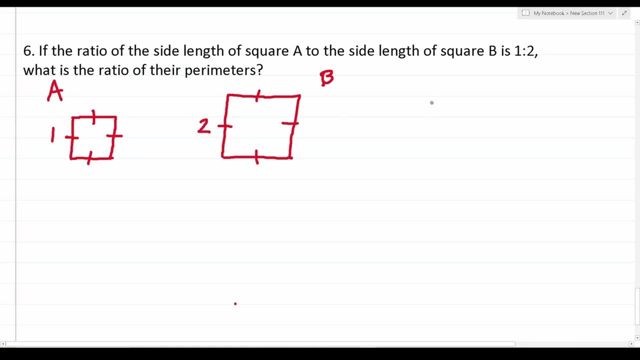 square A to the side length of square B is, you would say, it's one to two, Again, one to two, All right. And the question is this: Given this ratio of their side lengths, what is the ratio of their perimeters? So we're going to have to find the perimeter of square A. 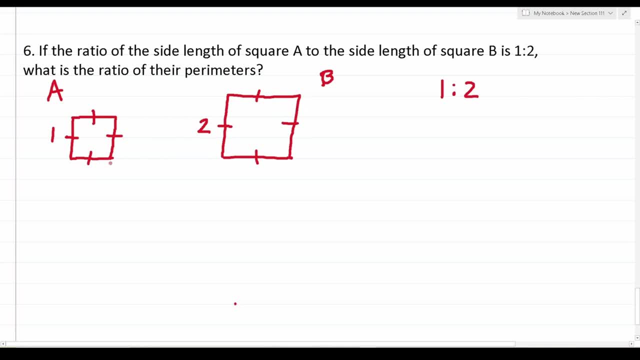 as well as the perimeter of square B And, as it happens, that's pretty easy to do. Again, if this side's one, this side's also going to be one. this side's going to be one and this side's going to be one. Likewise, this side's going to be two. this side's going to be. 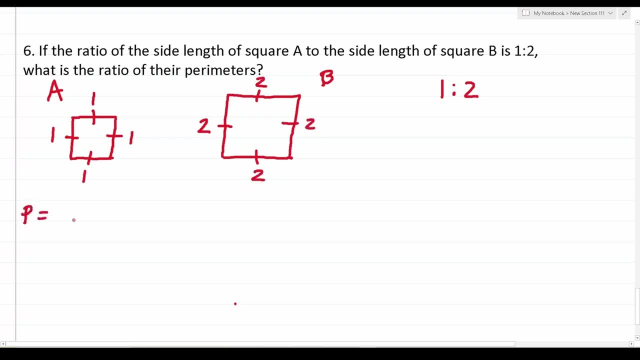 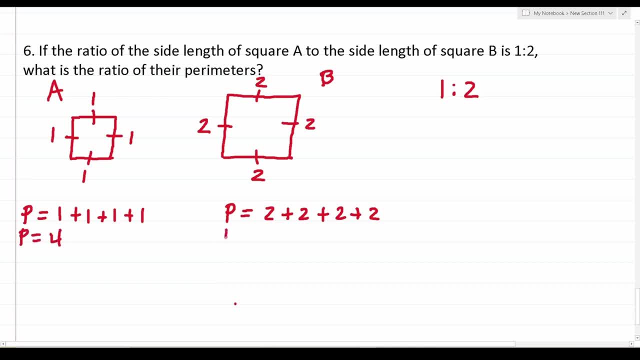 So the perimeter of square A is four And the perimeter of square B is two, four, six, eight. All right, So what is the ratio of their perimeters? Again, it's four to eight. But that said, can't we reduce that? Isn't four and eight both divisible? Aren't four and eight both? 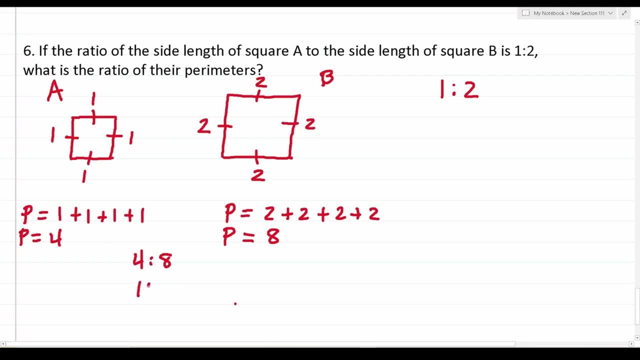 divisible by four. Again, four divided by four is one. Eight divided by four is two. All right, So the ratio of their perimeters is either four to eight, which is the same as one to two. In other words, the ratio of their side lengths is the same ratio as their perimeters. Again, their side. 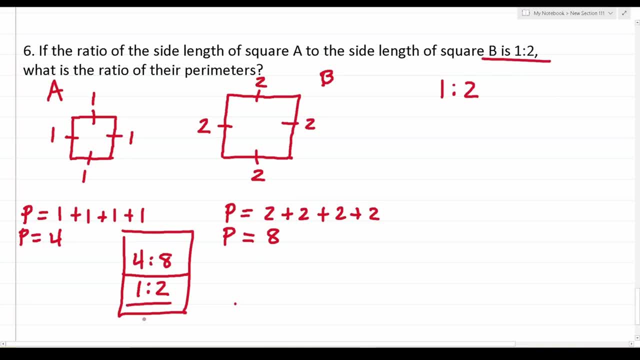 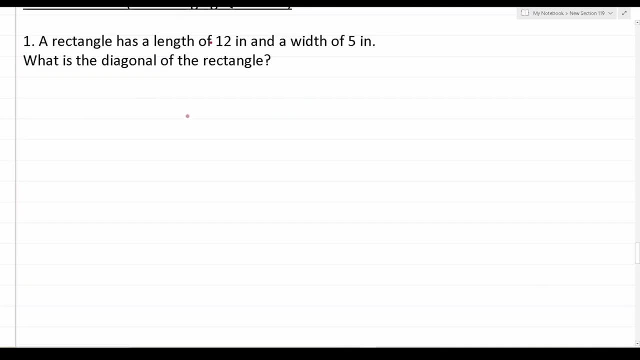 lengths had a ratio of one to two And ultimately their perimeters have a ratio of one to two as well. So number one says a rectangle has a length of 12 inches and a width of five inches. What is the diagonal of the rectangle? 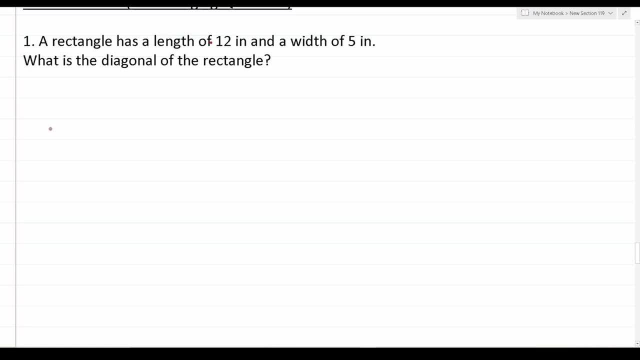 You might be saying to yourself: how am I going to figure out what this is using my knowledge of triangles? Well, let's make a sketch here. First, let's sketch a rectangle, since we know that's what we're dealing with, And you should know some properties of rectangles, Notably this length of 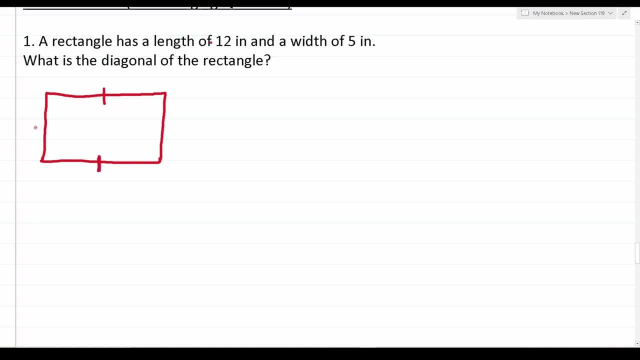 this rectangle is the same as this length And this width of the rectangle is the same as this width. So, according to the problem, this is 12,, which means that this is 12.. And this is 12.. And this is five, which means that this is five. And we want to know what is the diagonal of the. 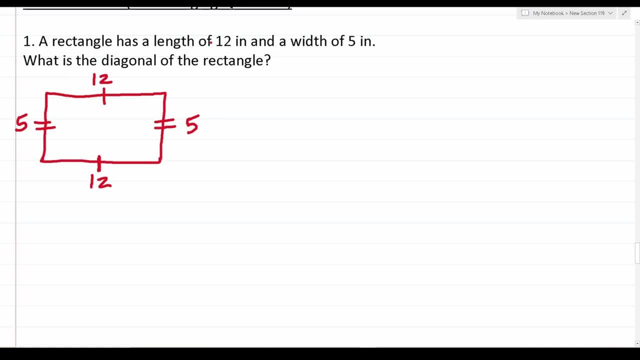 rectangle. Well, a diagonal of a rectangle basically means you cut it in half from here to here, And when you do that, what you get is a pair of right triangles. As a matter of fact, I can go ahead and pull one of those right triangles off to the side here. So we know, this is five and this. 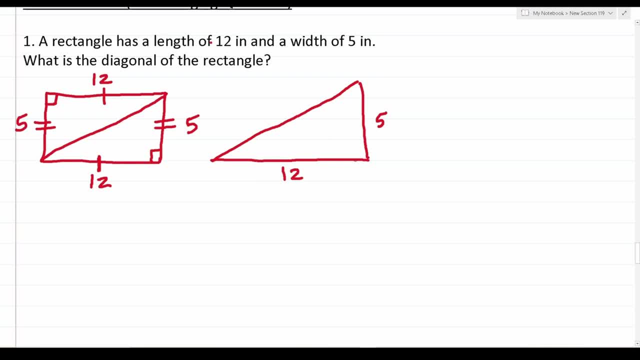 is 12.. Well, here's our right angle, And we know that right across from our right angle is our hypotenuse, our C. In other words, if we figure out what C is here, we'll know the length of this. 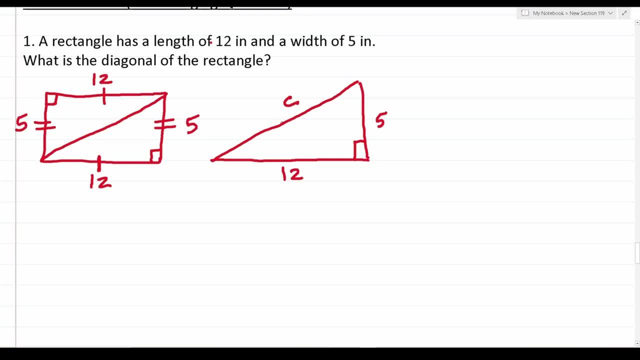 diagonal in this rectangle. And how can we figure out what C is the hypotenuse? Well, we can use the Pythagorean theorem. And the Pythagorean theorem says this: a squared plus b squared has to equal C squared, where a and b are the legs of the right triangle And C is the hypotenuse of. 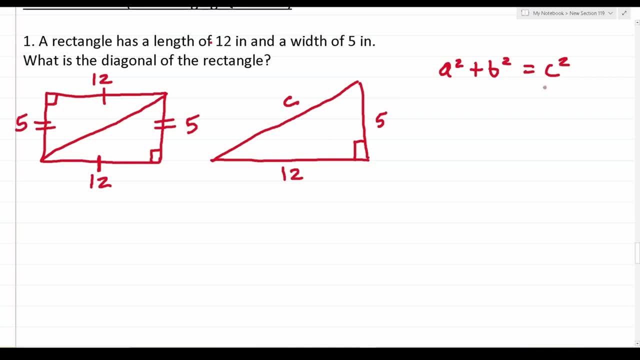 the right triangle. So we're going to be solving the Pythagorean theorem for C. we're going to let this be a and this be b, So this becomes 12 squared plus five squared equals C squared. 12 squared, of course, is the same as 12 times 12, which is 144.. 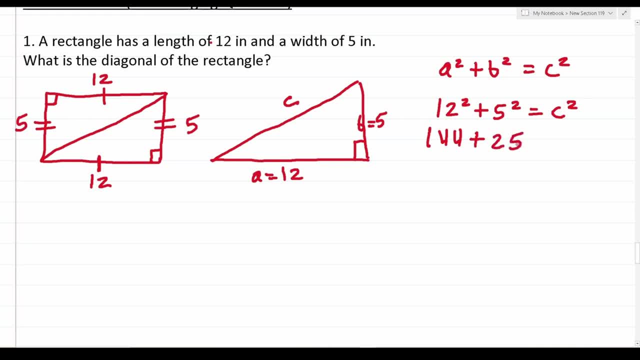 Five squared is 12 times 12,, which is 144.. Five squared is five times five, which is 25 equals C squared. So as not to make any mistakes here, I'm going to add these off to the side: 144 plus 25, four plus five is nine. four plus two. 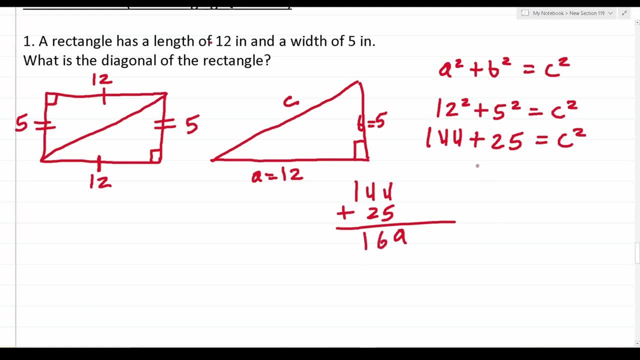 is going to be six and one plus nothing is one. So this is 169 equals C squared. We want to get C by itself, not C squared, So we're going to take the square root of both sides. This will cross out. 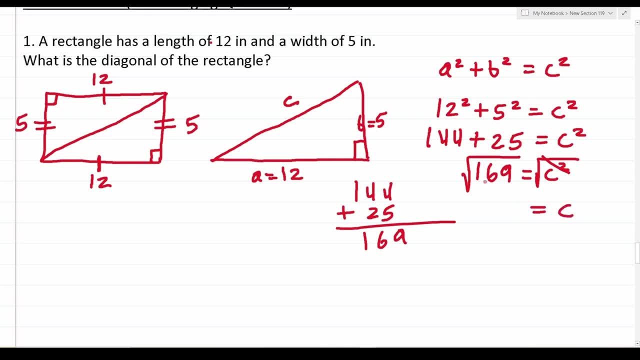 this square here, leaving us with just C on this side. What is the square root of 169?? It's on my reference sheet on my website. It's 13. So C in this case is 13.. Since C is 13,. 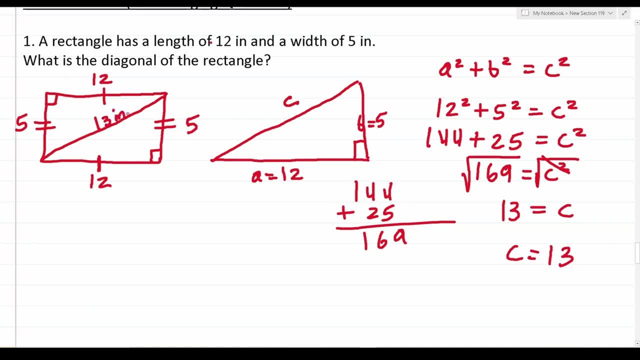 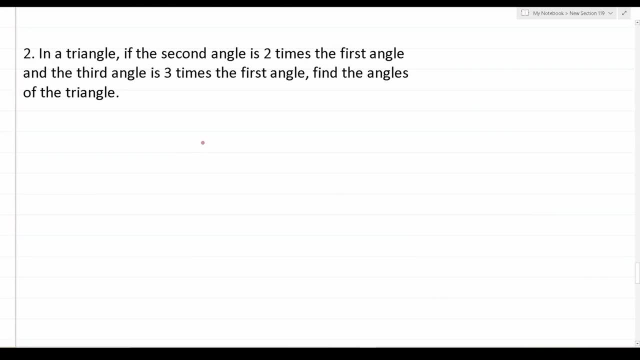 we know the length of this diagonal is also 13 inches. All right, so the answer to this one is 13.. All right, so number two here says: in a triangle, if the second angle is two times the first angle and the third angle is three times the first angle, then the second angle is three times the first angle. 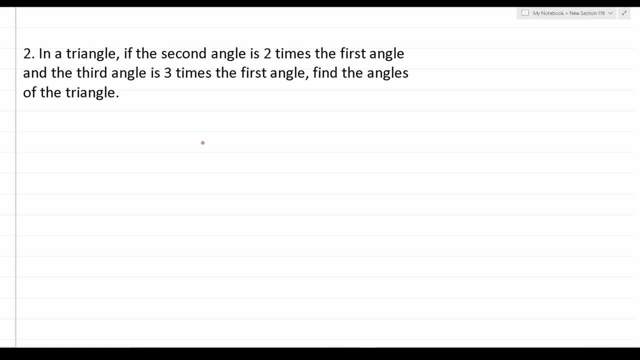 Find the angles of the triangle. Well, we can use the triangle sum theorem to figure this one out Again. according to the triangle sum theorem, angle one plus angle two plus angle three in a triangle are always going to add up to 180 degrees. And let's make a sketch, in this case to try to. 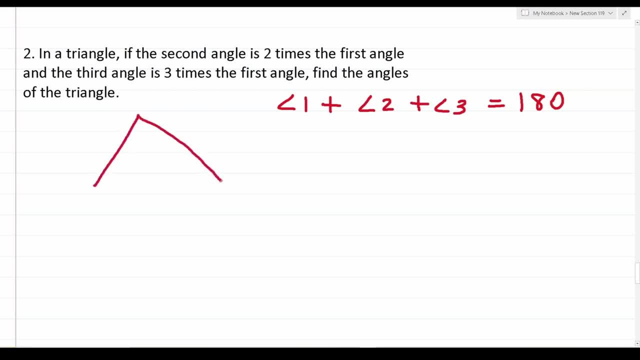 figure out what's going on in number two. So we have our triangle here and it seems to me that both angle two and angle three are going to add up to 180 degrees. So we're going to add up to 180 degrees. 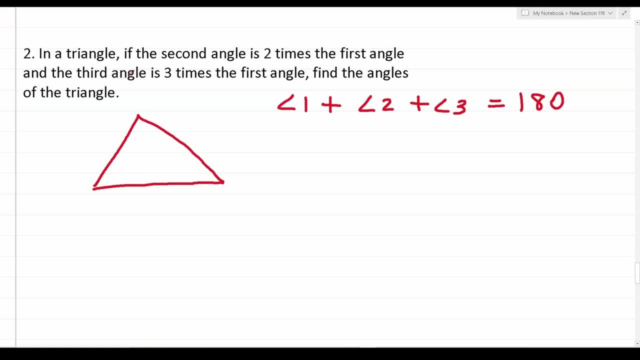 So we're going to add up to 180 degrees. So we're going to add up to 180 degrees And we're going to angle three reference angle one: It says the second angle is two times the first angle and the third angle is three times the first angle. And we don't know any of those values. 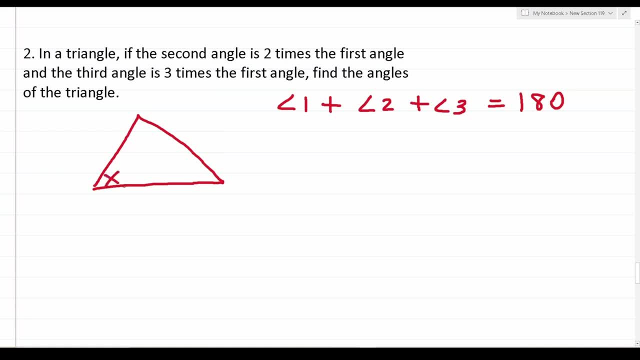 So I'm going to let angle one be x And let's go from there. If the second angle is two times the first angle, well, if the first angle is x, that means the second angle is 2x. Similarly, if the third angle is three times the first angle, that means that if the first angle is x, 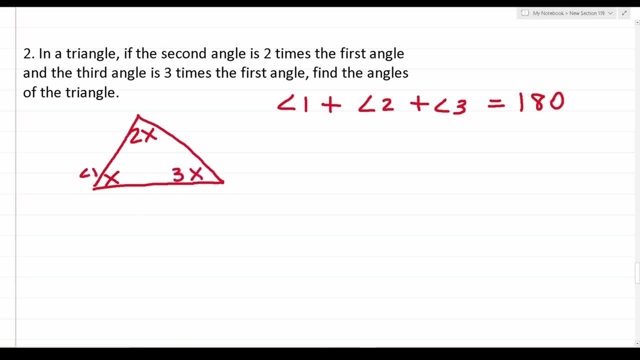 the third angle is going to be 3x. So here's angle one, here's angle two, here's angle three. Now let's plug those values into the triangle sum theorem. here This becomes x plus 2x plus 3x. 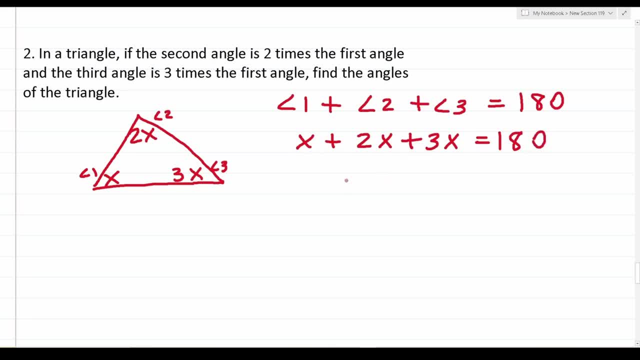 equals 180.. All these are like terms, so we can combine them. Plus 2x is 3x, 3x plus 3x is going to be 6x equals 180.. Now let's divide both sides by 6. 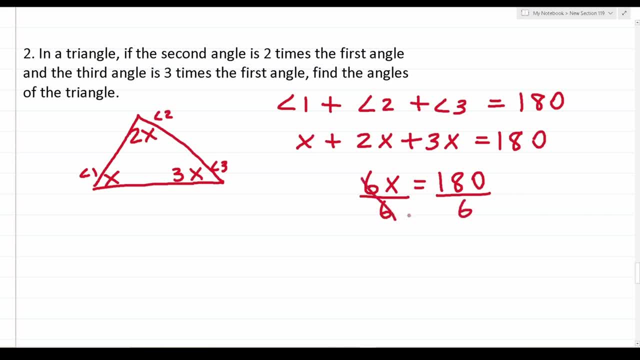 to get x by itself. This crosses out here, leaving us with just x, And you should be able to do this in your head. How many times does 6 go into 18?? Well, that's going to be three times, and then just drop down that zero. So, in other words, 180 divided by 6 is 30.. 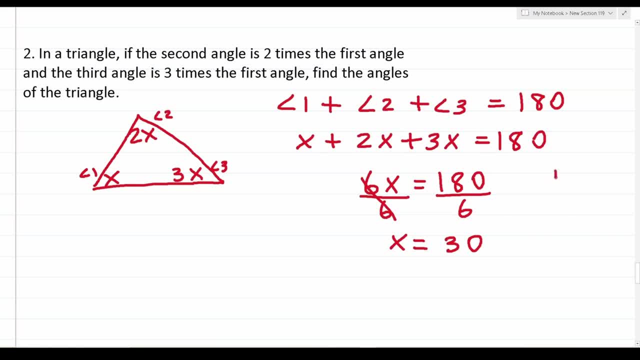 I'll do this. That's the long way, if you need to see it. This says 180 divided by 6.. 6 doesn't go to 1.. 6 goes into 18 three times, but that said 6 goes into 180 30 times. 30 times 6 is 180.. 180 minus 180. 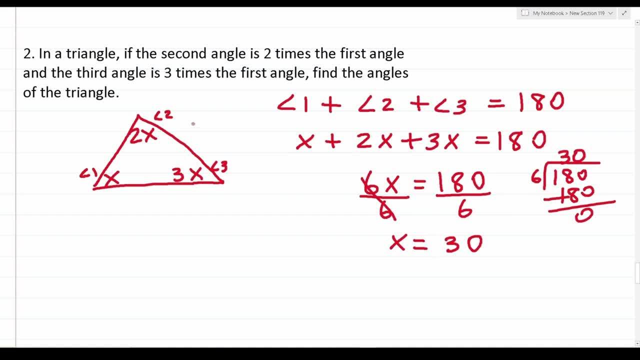 is zero. All right, Now we had to find all the angles of this triangle and we can see those are right here. Angle one is x, Angle two is 2x and angle three is 3x. So angle one is equal to x, and we know x is 30. So angle: 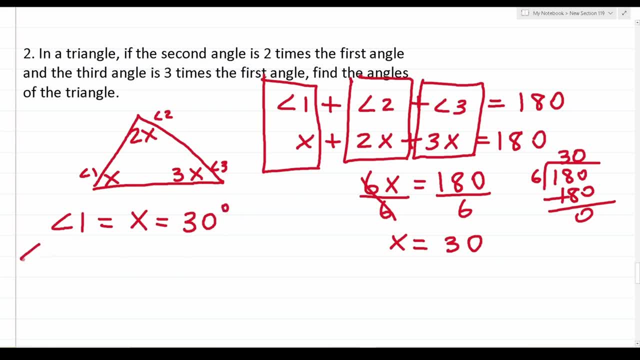 one is 30 degrees, Angle two is 2x and we know x is 30. So this becomes 2 times 30, which is 60 degrees. And then finally, angle three we can see is 30 degrees. So angle two is 2x and we know x is. 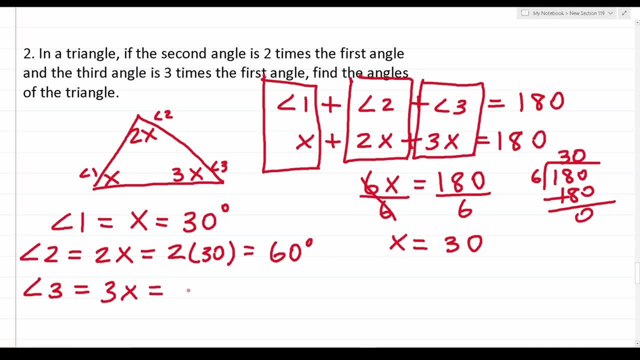 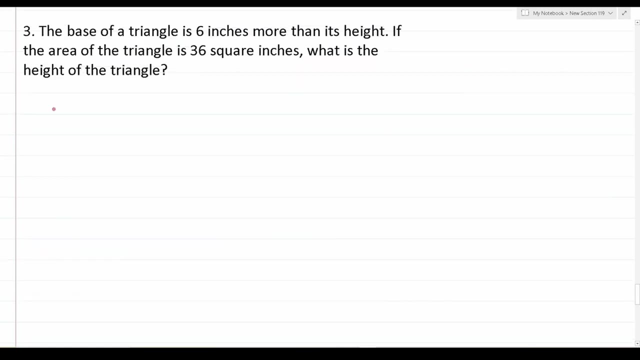 3x. We know x is now 30, so this becomes 3 times 30,, which is 90 degrees. All right, So those are our angle measures: 30,, 60, and 90.. And that is that one. So number three says the base of a. 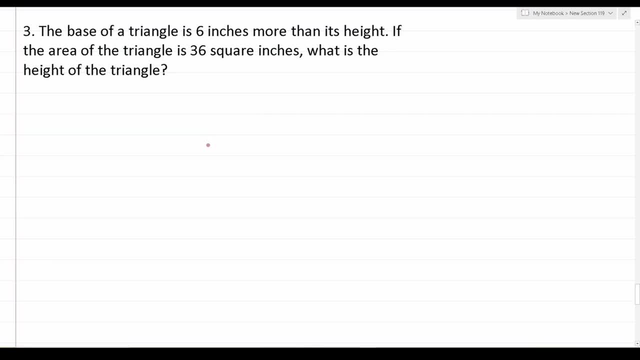 triangle is six inches more than its height. If the area of a triangle is 30, then it's 90 degrees 36 square inches. what is the height of the triangle? So it should be pretty clear that at some point we're going to have to use the area formula to figure this one out And to find the. 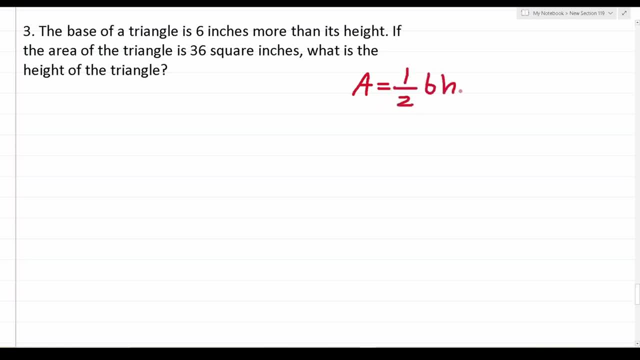 area of a triangle. it's one half base times height, So let's go ahead and just jot that down from the get go. And this problem is a little bit challenging because you also have to think about this problem both visually as well as algebraically. So let's start by thinking about 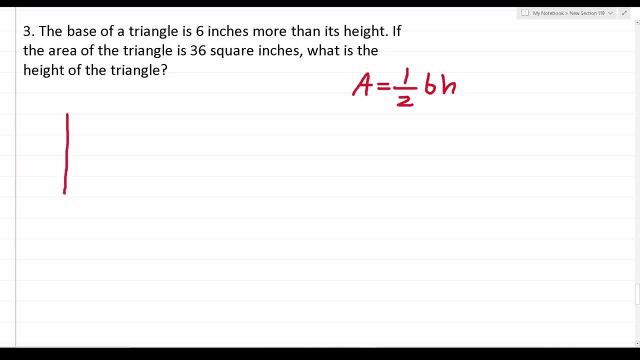 this problem visually. Visually, we're dealing with a triangle And, as it happens, I'm going to make a right triangle, since I think those are pretty easy to deal with. Here's the height of my right triangle And here's the base of my right triangle, That is this side. length is our height. 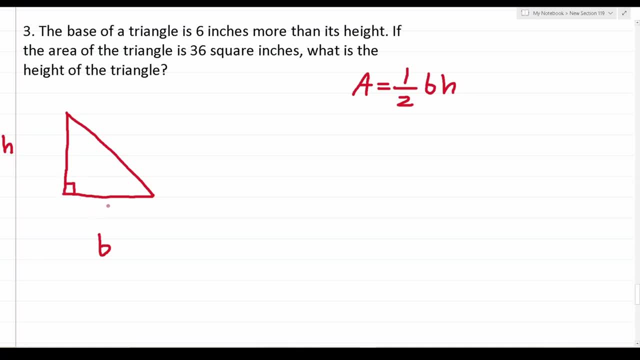 And this side length is our base. Well, what's this problem? say So, if we're going to do a right triangle, we're going to do a right triangle and we're going to. the base of the triangle is six inches more than its height. So we don't know how. 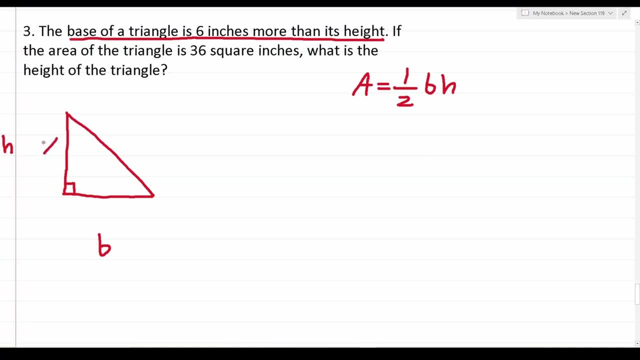 high this triangle is, So it's going to be x inches high, And that means its base is going to be x plus six inches long. All right, So we've taken care of the visual part as well as the algebraic part. Let's go ahead and try to solve this one. 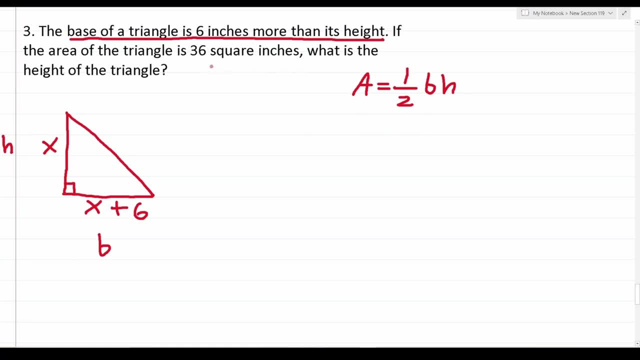 Using this formula. Now we're told, according to the problem, that the triangle has an area of 36 square inches. So we know a is 36 square inches. So this becomes: 36 equals one half. What is our base? It's x plus six. What is our height? A height is x. All right, So clearly, if we solve, 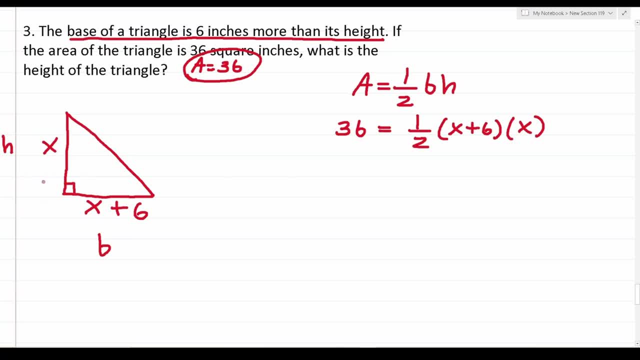 for x. here we'll know the height of this triangle. That said, we got this pesky fraction hanging out in front here, So let's go ahead and clear that by multiplying both sides of this equation by two, This will cross out here, And two times one half is just one. Anything times one is. 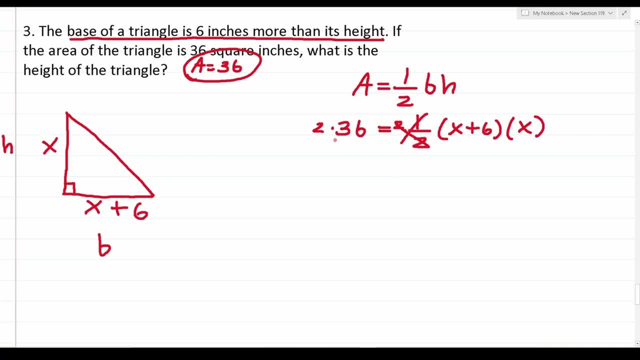 itself. So this goes away here. That said, we still have to work this out. 36 times two, Six times two is 12.. Carry a one Three times two is six plus one is seven. So this becomes 72 equals x plus six times x. 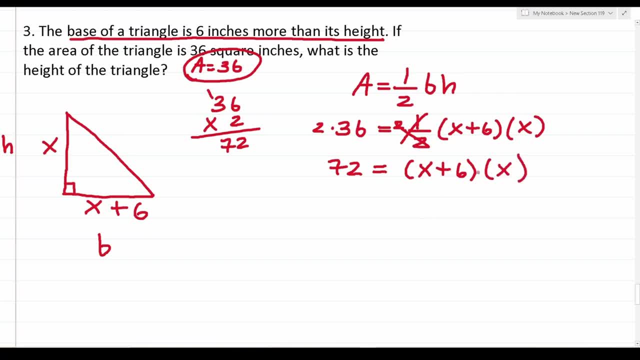 Let's go ahead and work this out using the distributive property. We got to take this x, We got to multiply it to this x, And then we have to multiply it to this six, So this becomes x times x, which is x squared, plus six times x, which is six. x equals 72.. 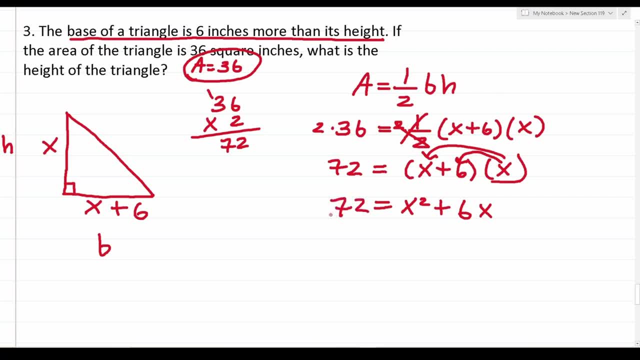 And at this point you're probably saying to yourself: how am I going to solve this one for x when I have x squared six, x and 72?? Well, if we subtract 72 from both sides, this crosses out here, leaving with zero on this side: x squared plus six, x minus 72.. 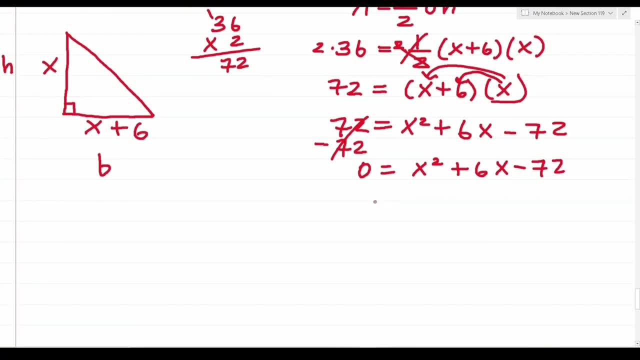 And let's go ahead and rewrite this such that the zeros on this side, this becomes x squared plus six, x minus 72, equals zero. Well, as it happens, you should be able to factor this, since this is a quadratic equation that has a leading coefficient of one. More specifically, 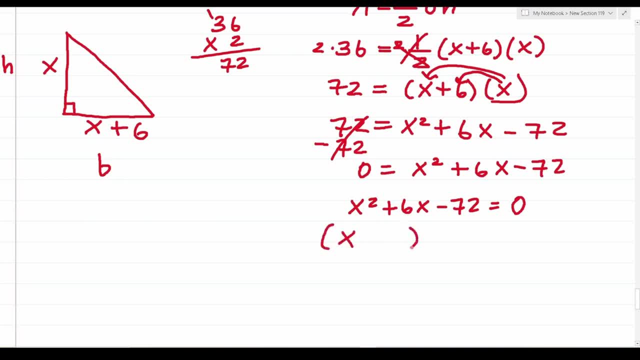 you should be able to factor this one like this: You should be able to go x times x. Now we have to figure out two numbers that multiply to negative 72, but add to positive six. Well, I know that 12 times negative six is negative 72. And similarly, 12 minus six is. 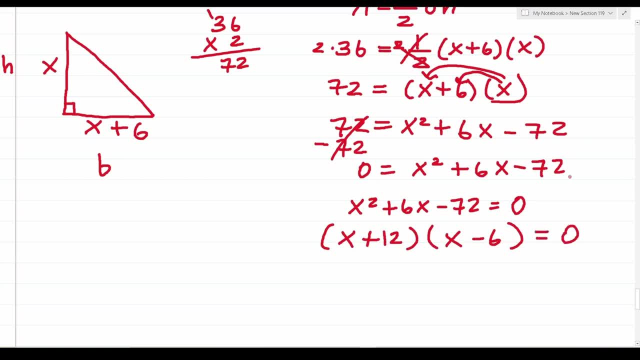 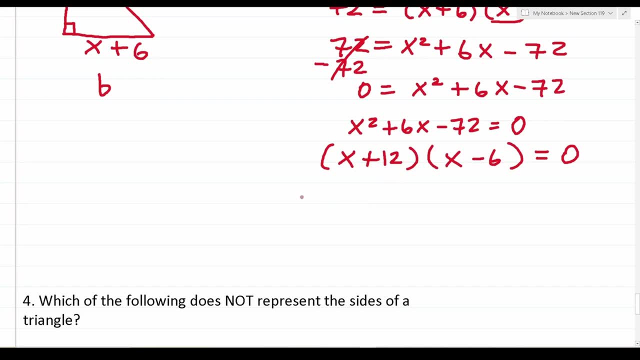 positive six. All right, so here are our two factors, But, that said, we're not done yet, because we have to solve these for x, which means we're going to set them both equal to zero. like this: x plus 12 equals zero and x minus six equals zero. 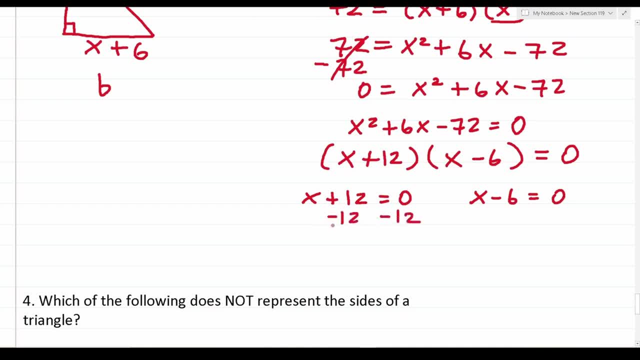 When we solve for x, here we're going to subtract 12 from both sides. This crosses out, leaving you with x equals negative 12.. And to solve for x, here we're going to add six to both sides. My pen's starting to die here. This crosses out here, leaving you with x equals six. Well, 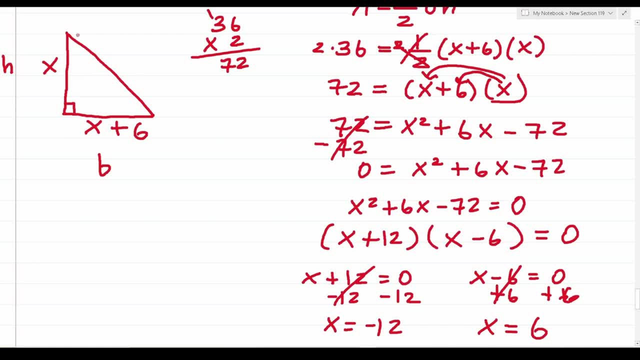 let's think about this. We know that the height of our triangle is x. Do you think it can be a negative value? It can't. so we know that's not correct. So we know x in this case is going to be six. So x is six And of course we can see that x corresponds to the height of this triangle. 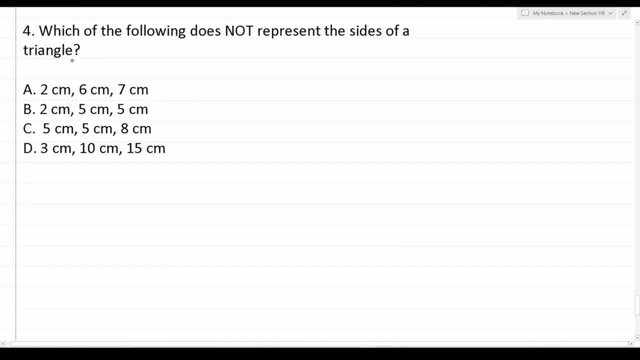 So that is that one. So number four, as you can see, says which of the following does not represent the sides of a triangle. Well, as you may recall, we can use the side lengths and the triangle inequality theorem to determine if something is a triangle or not. Specifically, 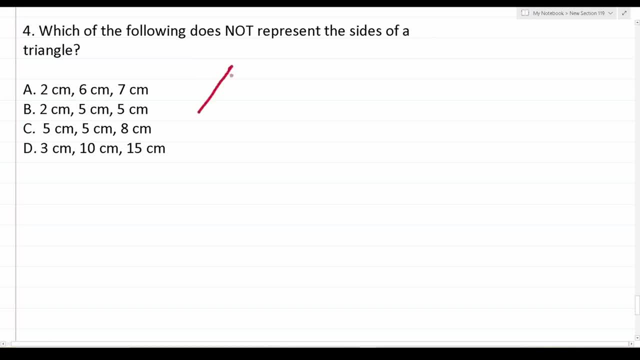 the triangle inequality theorem. So we can use the side lengths. and the triangle inequality theorem says this: We have a triangle. Let's go ahead and quickly draw a triangle. Then the sum of two of its sides always has to be greater than the third side. So if I let this side be a, this side be b. 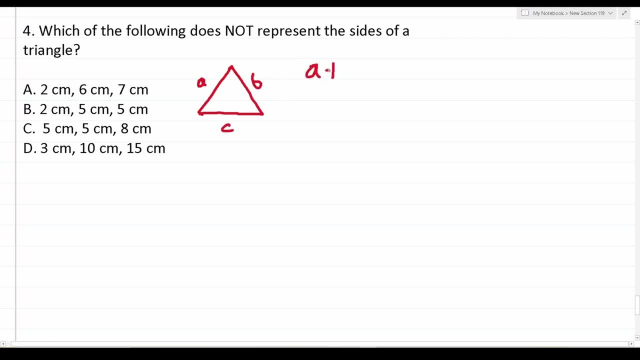 and this side be c. that means this: A plus b has to be greater than c. Likewise, a plus c has to be greater than b. And finally, b plus c has to be greater than c. So if I let this side be a, this: 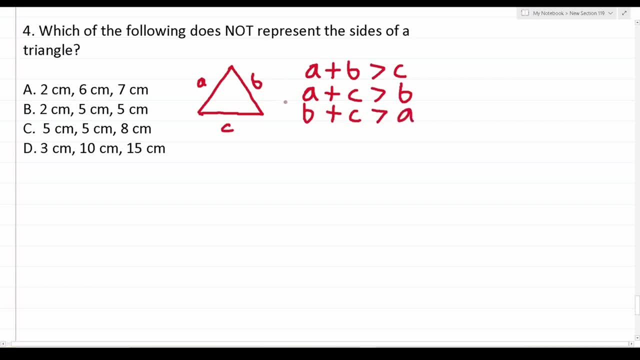 side has to be greater than a. If we fail to meet any of these conditions, then we do not have a triangle. So let's go ahead and apply that theorem to each of our answer choices here. And let me say this: I know this theorem so well and the math is so easy to do that just by looking. 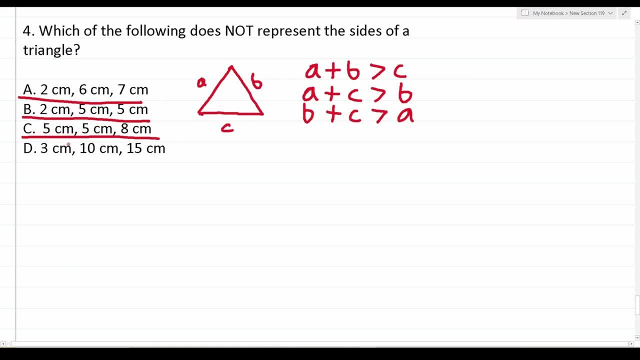 at the answer choices, I can tell you which of these is not a triangle. But, that said, let's work out one or two of these And then I'll explain how I quickly determine which one's not a triangle. So let's start with a here, And I'm going to make a triangle, since I think it will be helpful. 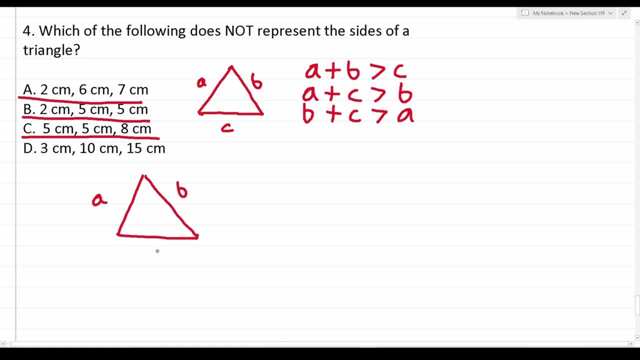 Again, let's call this a, this b and this c, And let's label these correspondingly: This is a, this is b, this is c, So this is two, this is six and this is seven, And let's apply these tests. 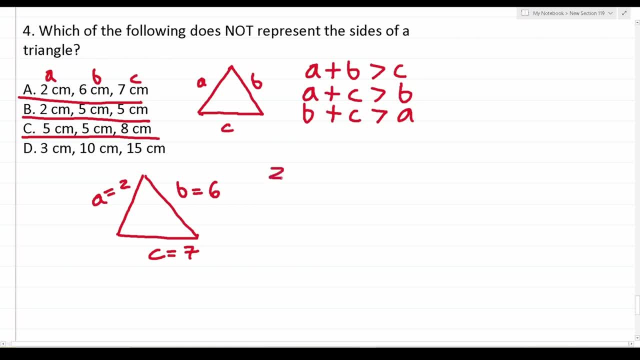 a plus b has to be greater than c, So two plus six has to be greater than seven. Two plus six is eight. Is eight greater than seven? It is All right, so we pass there. Next let's move to a. 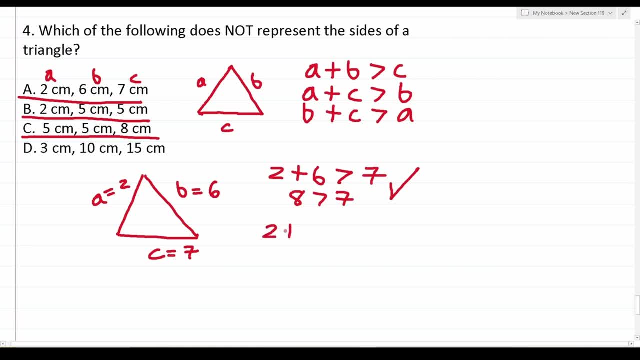 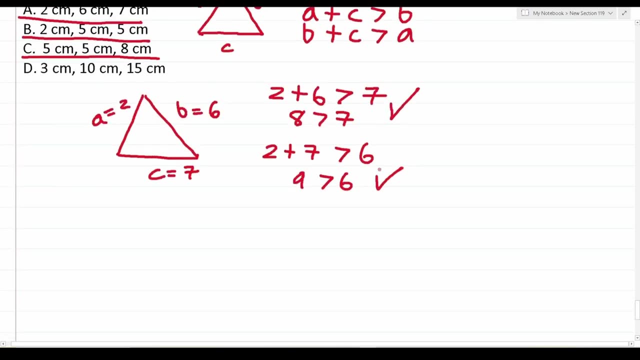 plus c, So that's going to be two plus seven. Two plus seven has to be greater than b, which is six. Two plus seven is nine Is nine, greater than six It is. And finally, let's move on to b plus c, And that has to be greater than a. b is six, c is seven. 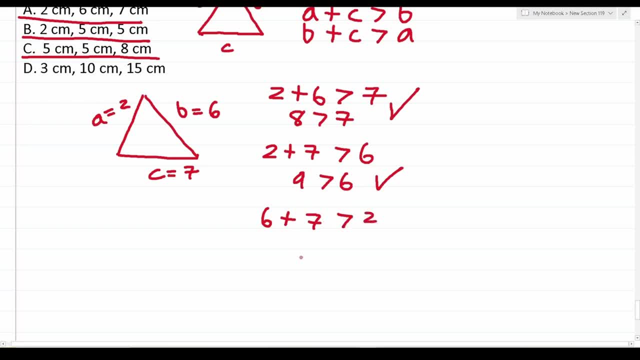 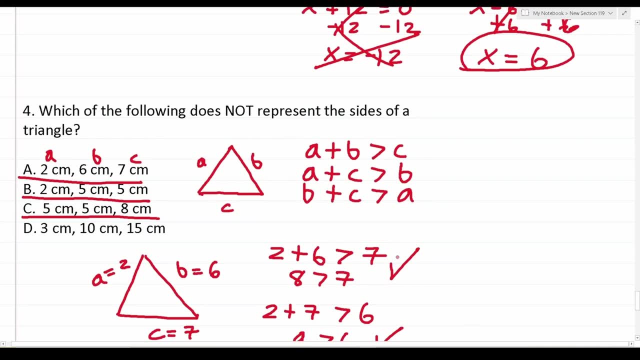 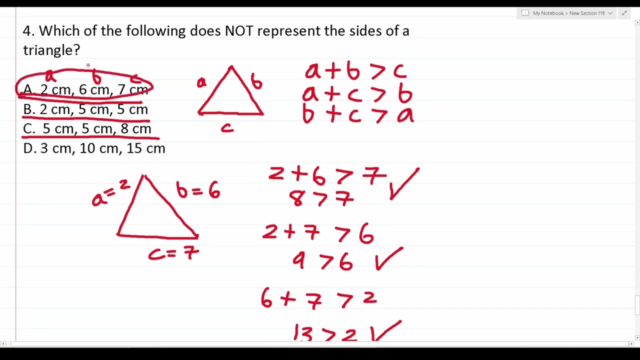 That has to be greater than a, which is two. Six plus seven is 13.. So 13 has to be greater than two. It is So, since these side lengths all passed the triangle inequality theorem, we know that a is in fact a triangle. 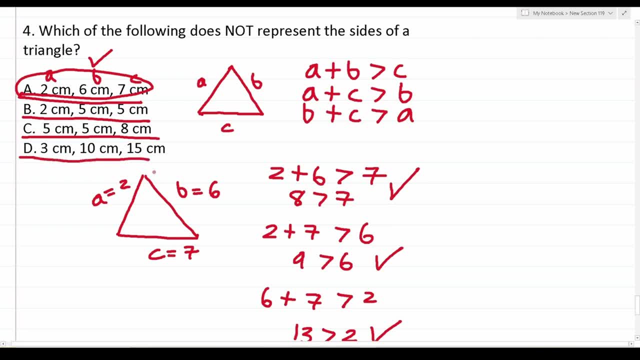 All right, let's go ahead and move to d and test that one out And if it's helpful, you can quickly make a triangle And I'm going to call this a, b and c And let's label these accordingly. This is. 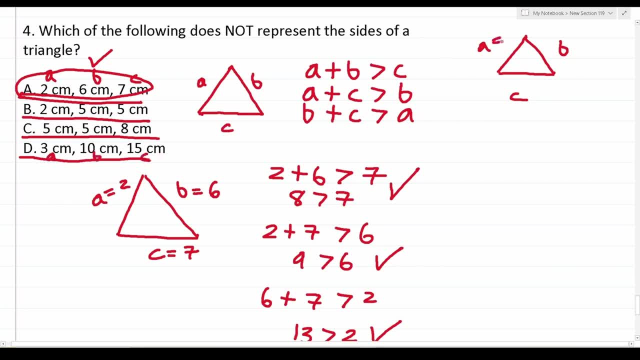 a, this is b and this is c. So this is three, 10, and 15.. And let's start applying these tests here. A plus B has to be greater than C, So 3 plus 10 has to be greater than 15.. 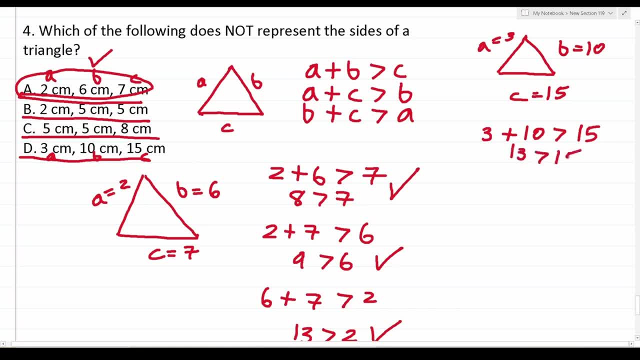 3 plus 10 is 13.. Is 13 greater than 15? It isn't, So this fails one of the conditions in the triangle inequality theorem. And therefore I know D is not a triangle, All right. And by the way, I knew that almost immediately because I said 3 plus 10 is less than 15.. 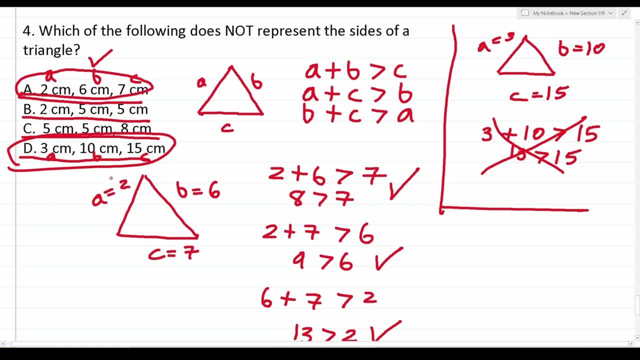 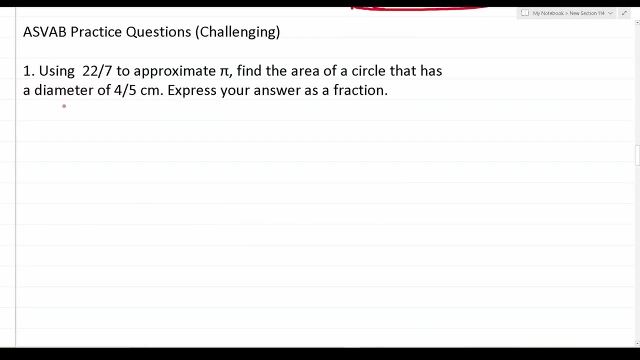 It fails to meet the conditions set out by the triangle inequality theorem. So again, don't be afraid to use mental math to figure these out, As long as you know that the sum of two lengths has to be greater than the third length. So this first question says: 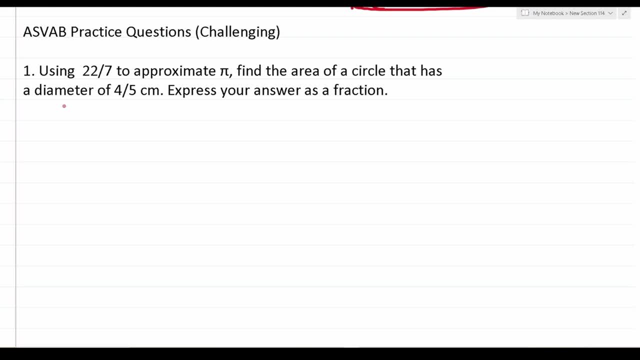 Using 22 over 7 to approximate pi, find the area of a circle That has a diameter of four-fifths of a centimeter. Express your answer as a fraction. All right. So first things first, we know we're going to be finding the area of this circle. 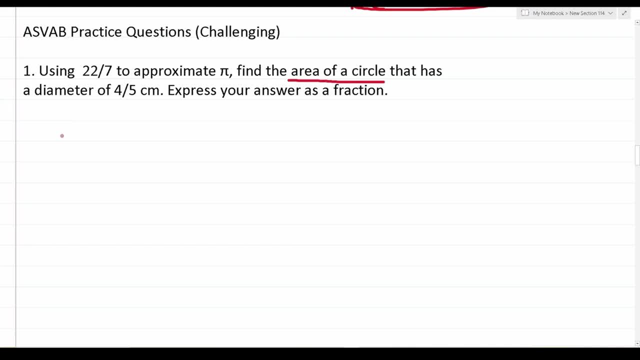 And there's only one formula we can use to find the area of a circle. Notably, area is equal to pi r squared, where r, of course, refers to the radius of a circle. All right, We have a little bit of a problem here. 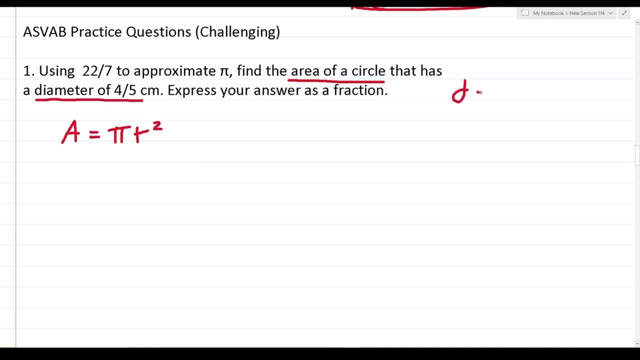 According to this problem, we know the diameter of this circle is four-fifths of a centimeter. That said, to find the area of this circle, we don't need its diameter, We need its radius. So, again, we're going to have to fall back on the relationship. 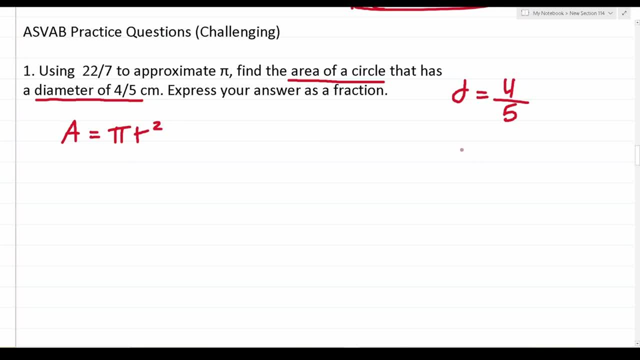 between diameter and radius of a circle. Notably, diameter is always twice as long as the radius, So in place of d here I can go ahead and plug in four-fifths. This becomes four-fifths equals divided by two r. 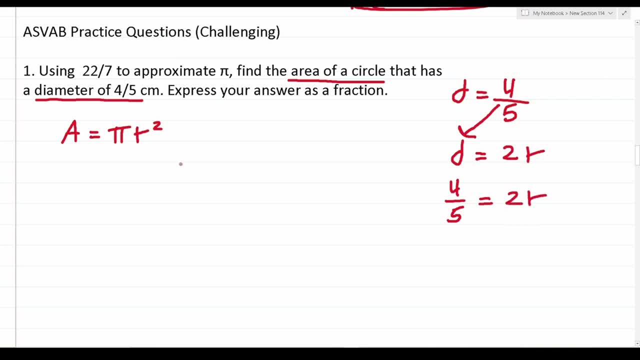 If we solve for r, we'll know what our radius is. So we're going to divide both sides by two. now This will cross out over here, leaving you with just r on this side, But, that said, we have this left. 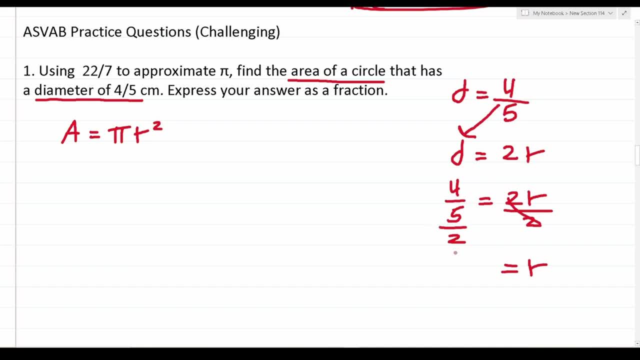 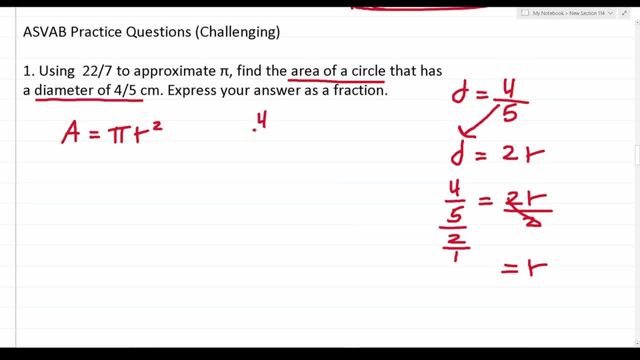 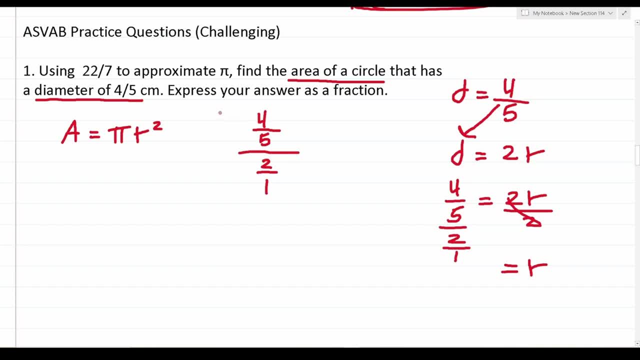 Well, how are we going to proceed? When you divide two fractions? you follow the algorithm keep change flip. That means you keep this top fraction as is, So that's going to be four-fifths. You change from division to multiplication. 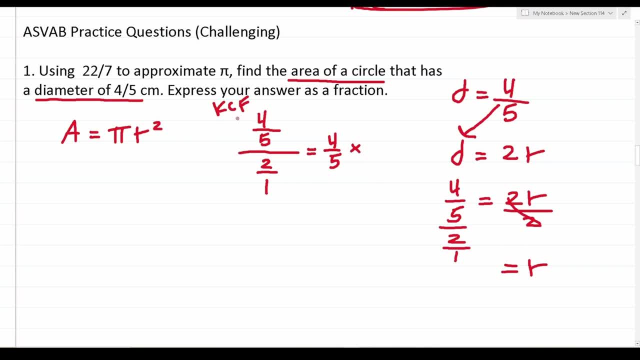 So we went from division to multiplication. That's our change. And then you flip this second fraction, So instead of being two over one, it's going to be one over two. All right, So now we're just multiplying four-fifths by one-half. 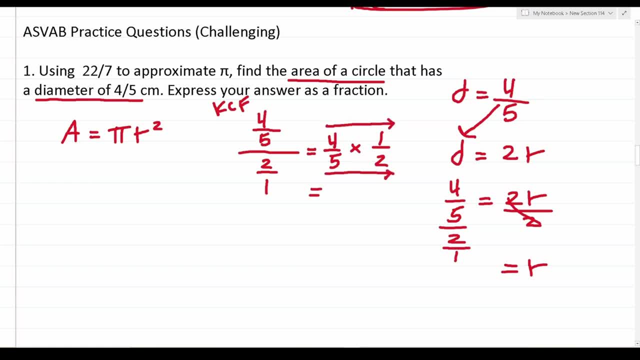 When you multiply fractions, you just multiply straight across. So four times one is four. Five times two is ten. This becomes four-tenths, And we can reduce this very quickly. You should notice that both four and ten are divisible by a common factor of two. 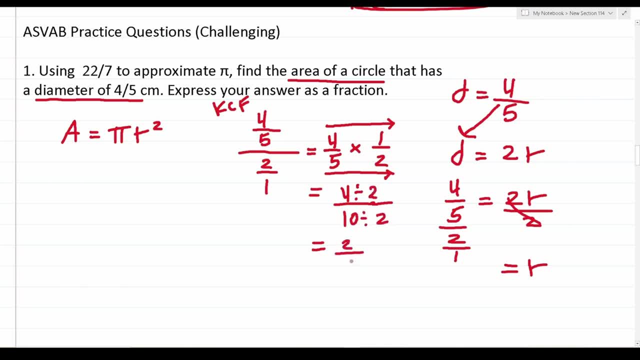 Four divided by two is two. Ten divided by two is five. So we know our radius in this case is going to be two-fifths. All right, So now that we've figured out what our radius is, we can go ahead and plug it into our formula over here. 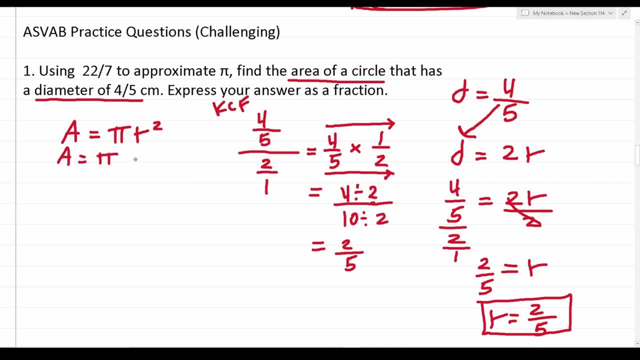 This becomes: area equals pi and radius is two-fifths. All right, So let's go ahead and work this out. Two-fifths squared. How are we going to deal with that? Well, whenever you have a fraction squared like this: 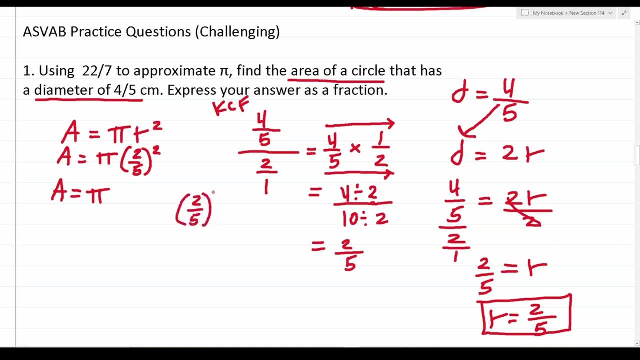 it becomes this: Okay, We have two-fifths squared. This square is going to be applied to each of these separately, So I like to think about this one like this: Two squared over five squared. Two squared is four. Five squared is twenty-five. 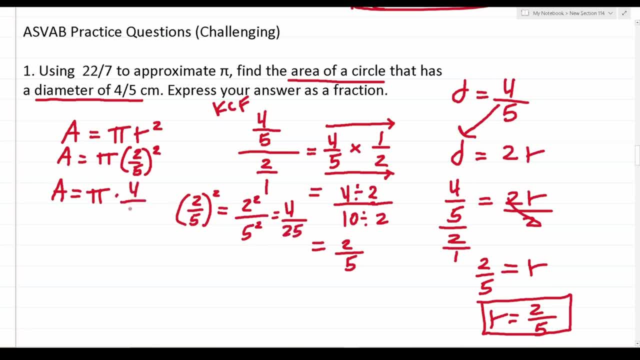 So this becomes pi times four over twenty-five. Of course we were told to use twenty-two over seven to approximate pi. So we know pi is going to be twenty-two over seven times four over twenty-five. And now we're just multiplying two fractions again. 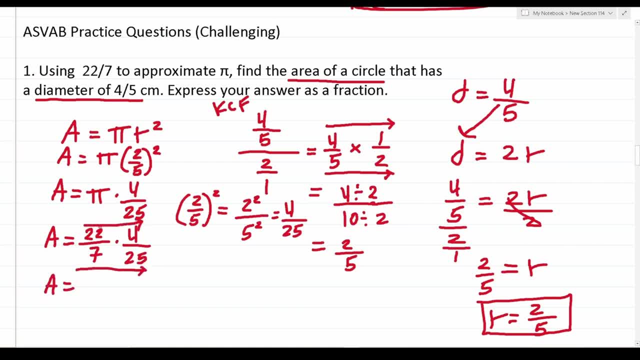 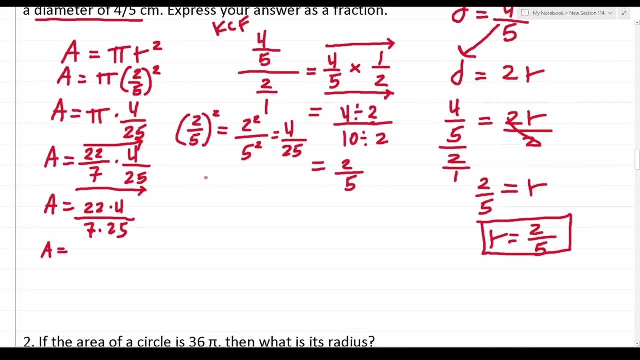 So we're going to multiply straight across. That is to say, this is going to become twenty-two times four over seven times twenty-five. Let me go ahead and scroll down a little bit. If you can't do this mentally, you can always do it off to the side. 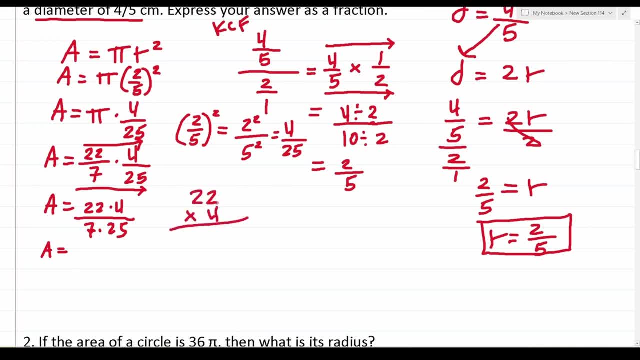 Twenty-two times four. Two times four is eight. Two times four is eight. So this becomes eighty-eight over What is seven times twenty-five. Again, if you can't do that mentally, you can always work it off to the side. 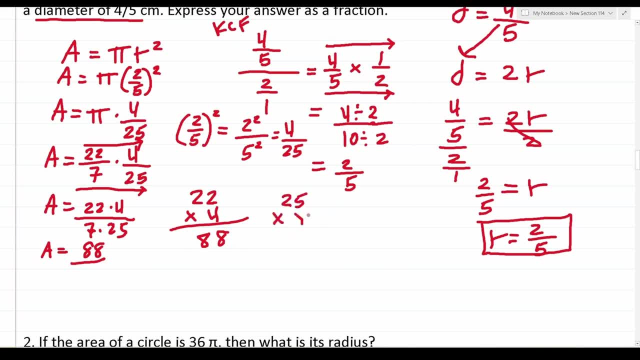 Like this. My pen's starting to act up on this. one Seven times five is thirty-five, So bring down a five, carry a three Seven times two is fourteen, fifteen, sixteen, seventeen, So this is eighty-eight over one-seventy-five. 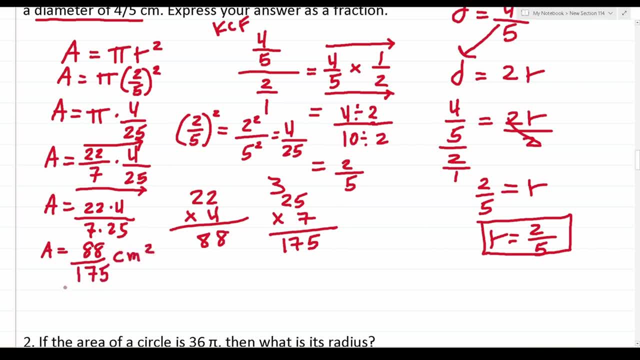 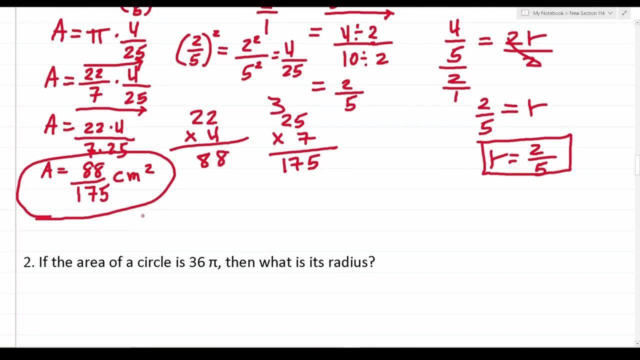 Of course this is going to be centimeters squared And the problem said: leave your answer as a fraction, And I do not believe we can reduce that. So our answer to this one is: its area is eighty-eight over one-hundred-and-seventy-five centimeters squared. 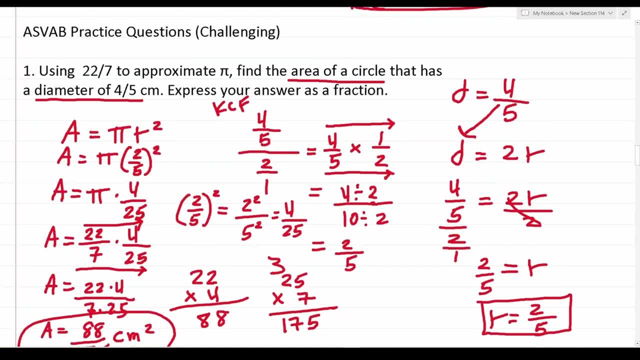 All right. So, as you can see, I can quickly throw in a lot of simple things into a word problem to make it much more challenging than what we've seen so far. As a matter of fact, first I tested your knowledge of knowing the formula to find the area of a circle. 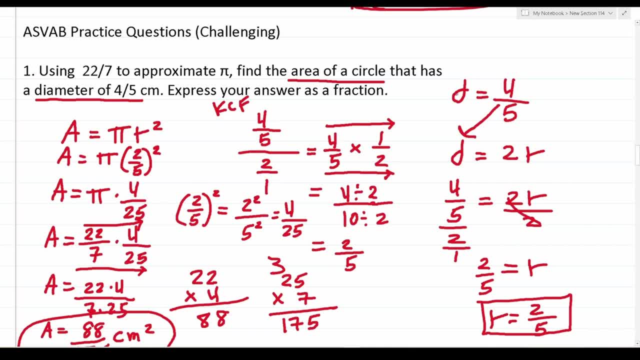 After that, I tested your knowledge of the relationship between diameter and radius. In the middle of that, you had to know how to divide fractions and multiply fractions. Okay, So this is a very typical question that you may see on the ASVAB or PI-CAT. 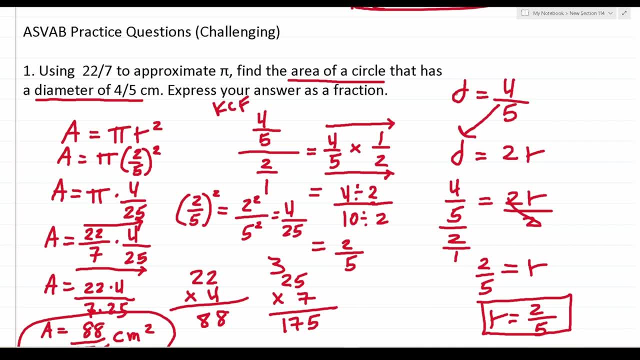 You can't escape working with fractions. You have to know how to work with fractions. In addition, you have to memorize these formulas and you also have to know the relationship between diameter and radius of a circle. So, again, that's a very challenging problem. 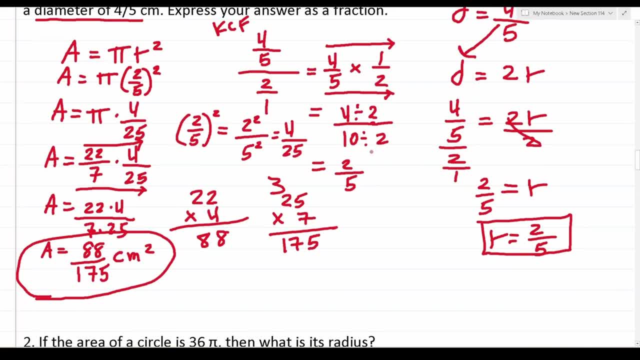 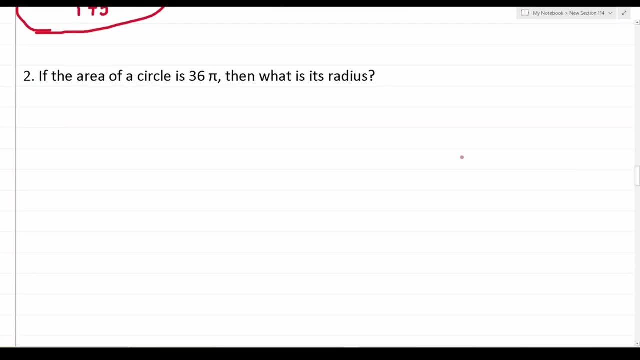 but it's representative of what may show up on the actual test. All right, So that's that one. All right. So number two says: if the area of a circle is thirty-six pi, then what is its radius? All right, 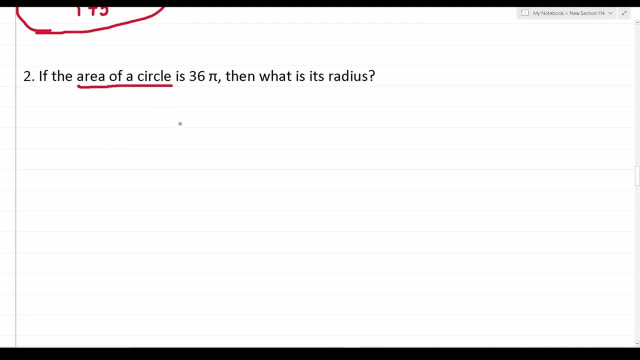 So we know we're working with the area of a circle. So let's write down that formula: Area equals pi, r squared. In this case, we were told that the area of this circle is thirty-six pi And we want to figure out what its radius. 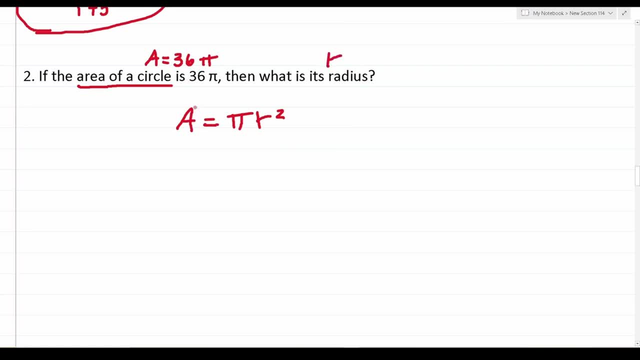 or r is. So in place of a, I'm going to go ahead and plug in thirty-six pi. This becomes thirty-six pi equals pi r squared, And again we're trying to figure out what its radius or r is. 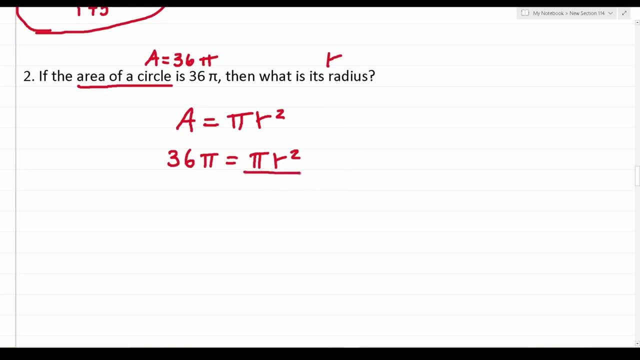 So we're going to be solving for r in this case. So let's start by dividing both sides by pi. This crosses out here, leaving you with just r squared on this side. These two pi's cross out over here, leaving you with just thirty-six on this side. 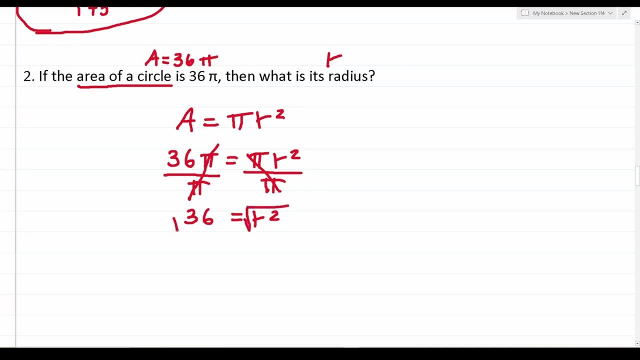 To get rid of this square, we're going to take the square root of both sides. This will cross out this square, leaving you with just r here. The square root of thirty-six is just six, So we can see r in this case is six. 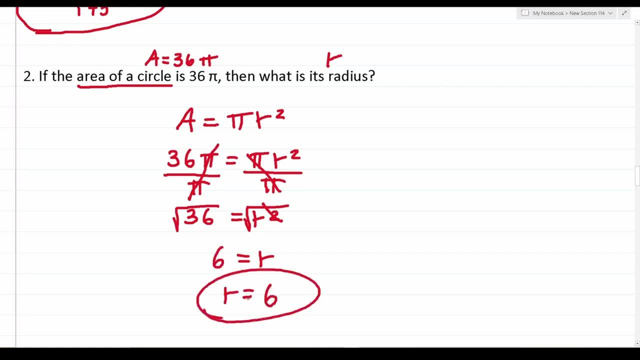 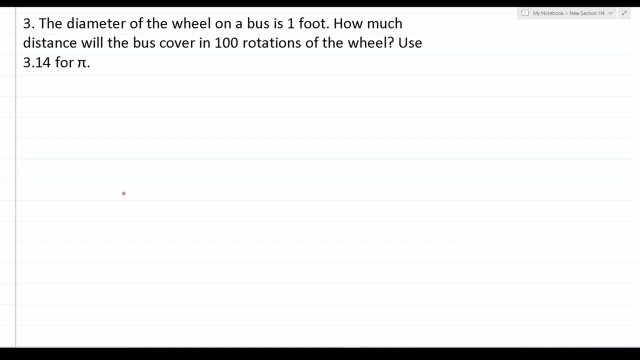 And we weren't given a unit, so we're just going to say the radius is six. All right, So number three says the diameter of the wheel on a bus is one foot. How much distance will the bus cover in a hundred rotations of the wheel? 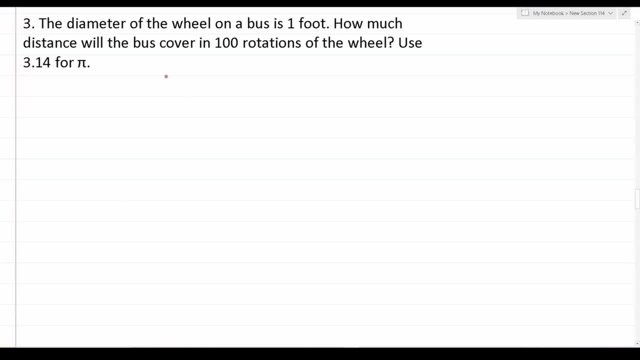 Use three point one, four for pi. All right. So for this problem you have to understand that there is a relationship between the circumference of a circle and the distance a wheel travels on the ground, And let me go ahead and try to explain that for you. 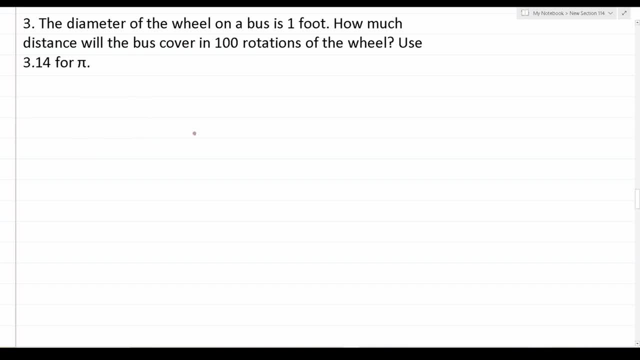 So let's say we had this circle here. Let me draw a better circle. Let's say we had this circle Here and let's imagine I tied a string around this circle, So it's snug all the way around. Well, what if I cut that string and then laid it out flat on the 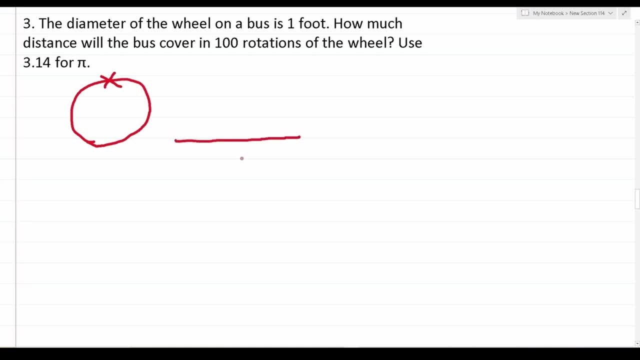 ground like. so What that would tell you is: the circumference of the circle is the same distance that the wheel travels upon one rotation. Again, the circumference of a circle Is the same distance that a wheel travels upon one rotation. And again, if it's helpful, think about tying the string. 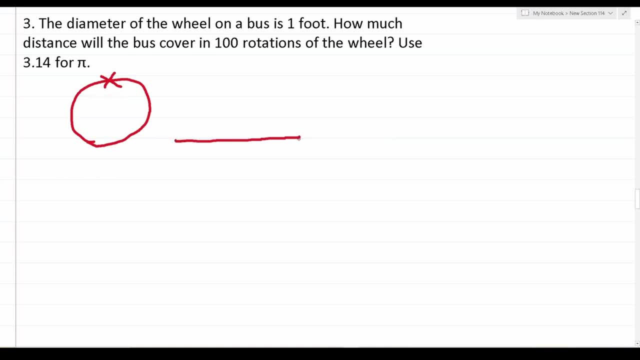 around a circle, cutting that string and then laying that string flat across the ground. All right, So for this one we're going to start by finding the circumference of this wheel. We know this wheel has a diameter of one foot And again, there are two formulas to find the circumference. 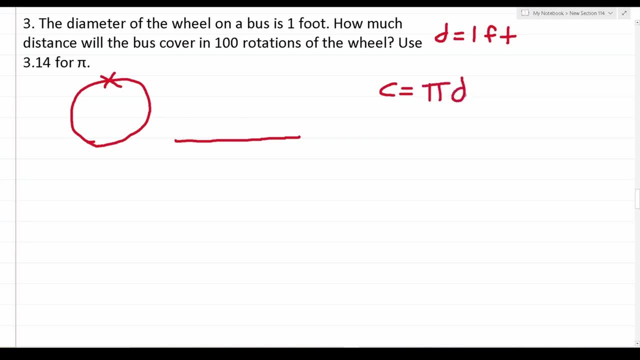 of a circle. Notably, we're going to use pi r as well as pi times diameter. since we were given diameter, We're going to use pi times diameter in this case And, of course, we're going to take one and plug it in for D. 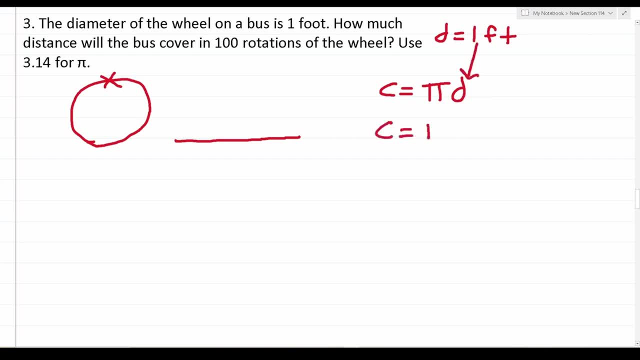 So this becomes: circumference equals pi times one, And of course we were told to use 3.14 to approximate pi, So let's plug that in as well. Anything times one is itself, So 3.14 times one Is 3.14.. 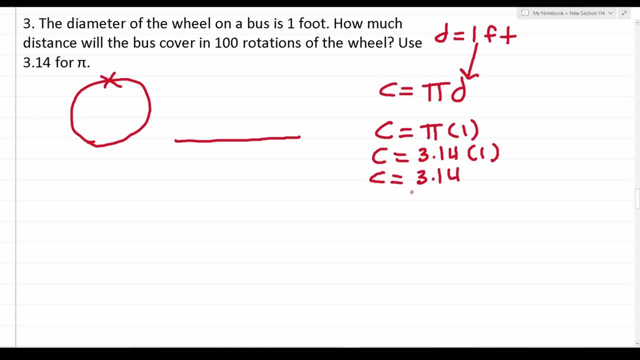 So we know that this bus wheel has a circumference of 3.14.. That means that upon one rotation it goes 3.14 feet across the ground. In order to figure out how much ground it covers upon a hundred rotations, we're going to take 3.14 and we're going to multiply. 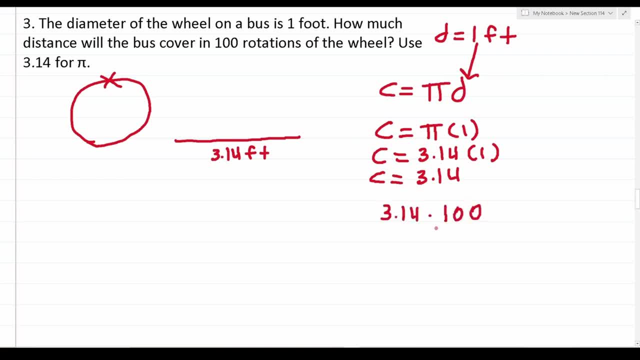 that by 100.. All right, And this math, as it turns out, is very easy to do. As you can see, we're multiplying 3.14 by a power of 10, notably 100.. As I mentioned in this video previously, when you multiply a, 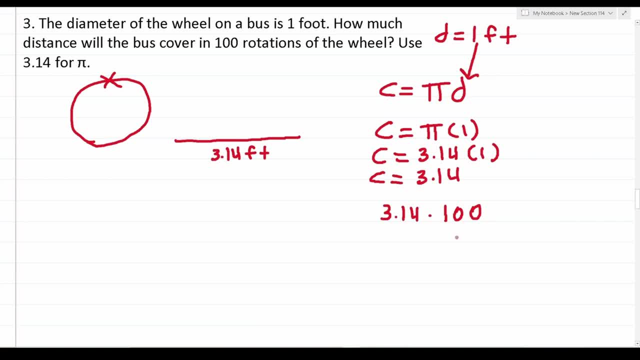 decimal by a power of 10,, such as 10,, 100,, 1,000,, 10,000, and so on. you just take that decimal and you shift it to the right according to how many zeros there are in your power of 10.. 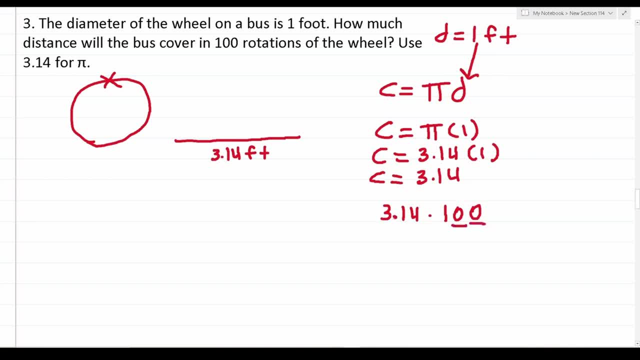 Well, in 100, there are two zeros, So we're going to take 3.14.. We're going to shift it one, two times to the right and our decimals right here, So this becomes 314.. In other words, if this wheel on the bus that has a diameter of one, 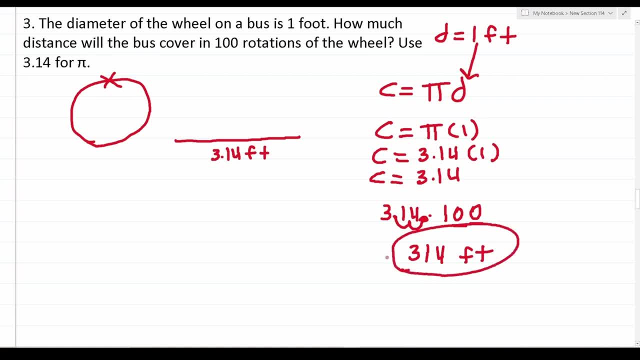 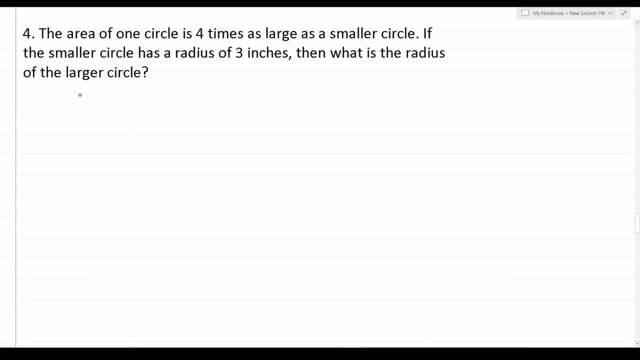 foot is rotated a hundred times, that means that the bus will have traveled the total distance of 314 feet. All right, So number four says the area of one circle is four times as large as a smaller circle. If the smaller circle has a radius of three inches, then what is the? 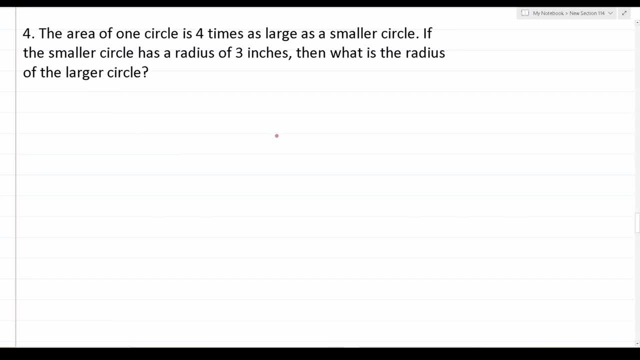 radius of the larger circle. So at first glance, this problem seems pretty challenging, and it is. That said, at the end of the day, we're just comparing two circles with each other. In addition, we know that this small circle has a radius of three inches. 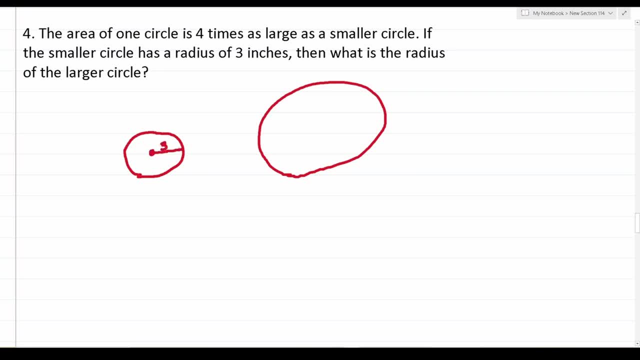 And we want to know what the radius of this large circle is. Again, this large circle has four times the area of this small circle. So the first thing I want to do is figure out what the area of this smaller circle is And again to find the area of a circle. it's pi? r squared. 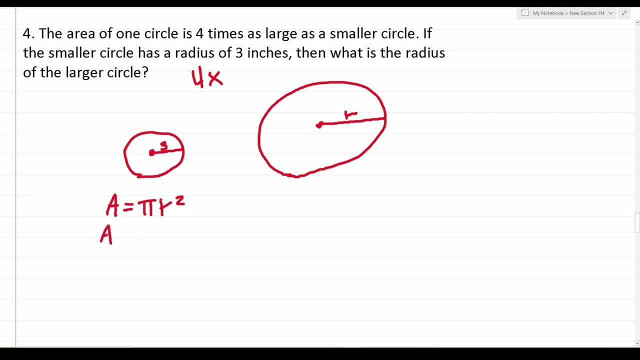 We know the radius of this small circle is three, so this becomes area equals pi three squared. Three squared is nine, So the area of this small circle is nine pi. Again, if the area of this small circle is nine pi, that means that the area of 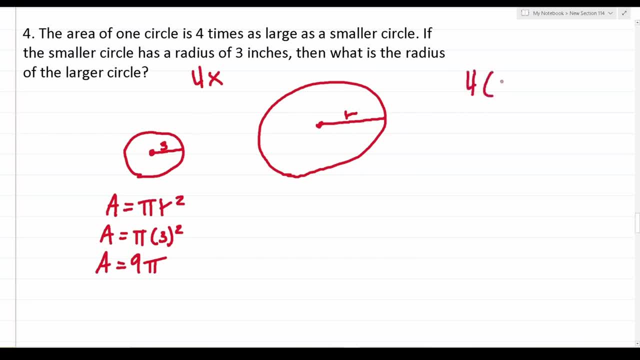 this big circle is going to be four times nine pi. What is four times nine- Four times nine, of course, is 36.. So the area Of this big circle here is 36 pi, And we saw previously that if we know the area of a circle we can find its radius. 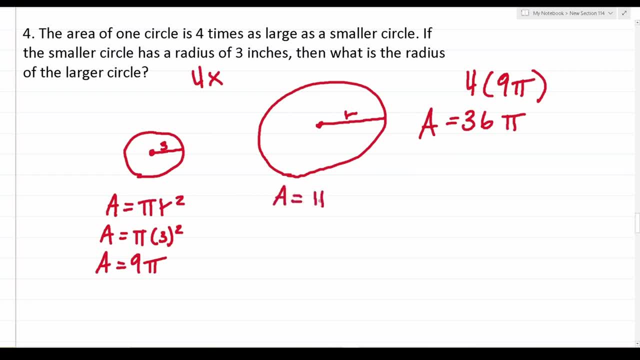 Again, the area of this big circle would be pi r squared. We know that this big circle has an area of 36 pi, So in place of a here, I'm going to put: 36 pi equals pi r squared. Let's divide, as we did previously, both sides by pi. now, 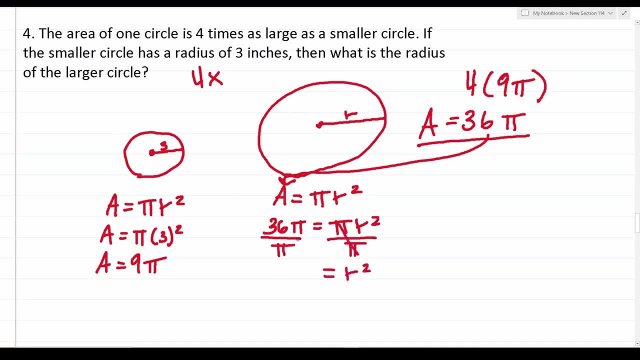 This crosses out, leaving you with r squared over here. These cross out as well, leaving you with 36.. To get rid of this square, we'll take the square root of both sides. This will cross out this square, leaving you with r on this side. 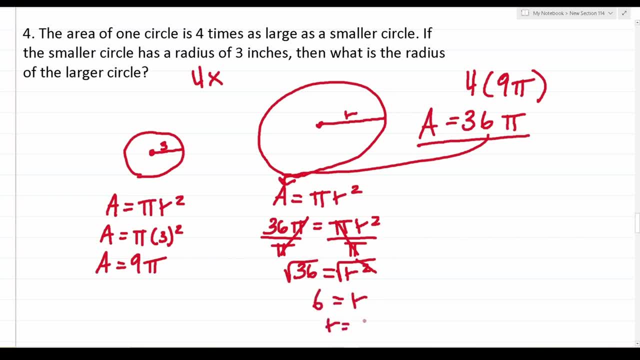 The square root of 36 is six, so r in this case is six, And that's going to be inches. All right, So The radius of our larger circle, as you can see, is six inches. All right, So that's that one. 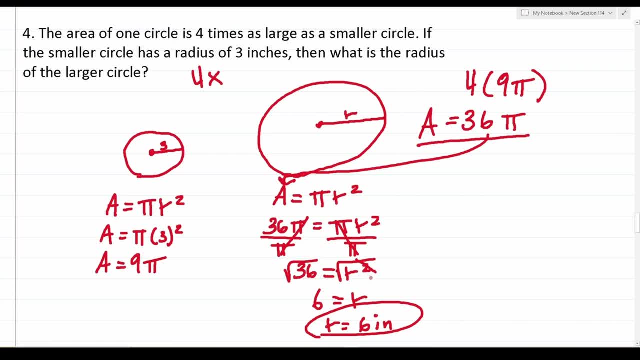 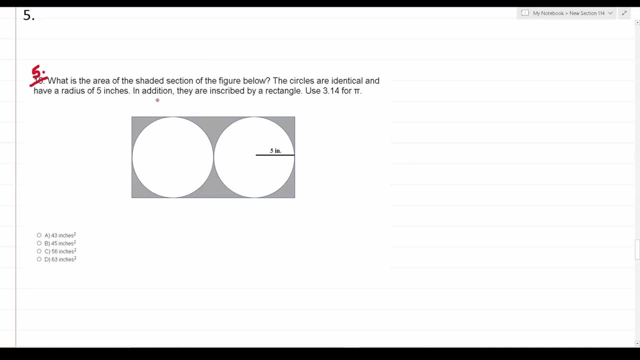 Somewhat of a challenging problem, but you may have noticed that to solve these more challenging problems, we're using all the smaller pieces that we worked out from the easy problems. All right, So number five, which is a question I got from one of my free practice tests on 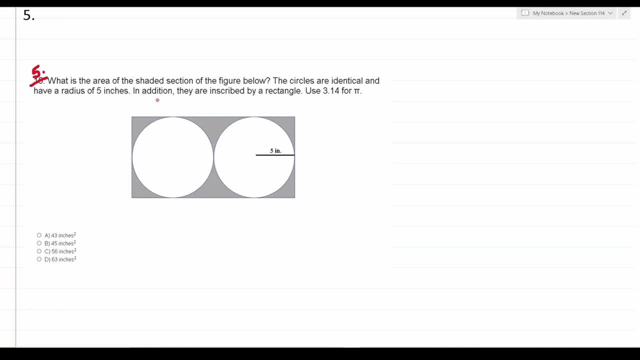 my website says this: What is the area of the shaded section of the figure below? The circles are identical and have a radius of five inches. In addition, they're inscribed by a rectangle. Use 3.14 for pi, All right. 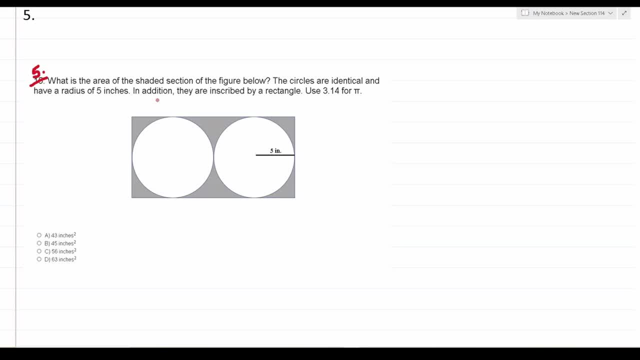 So again we're trying to figure out what the area of the shaded section below is, And it should be pretty obvious that to find the area of the shaded section we're first going to find the area of our rectangle And from that 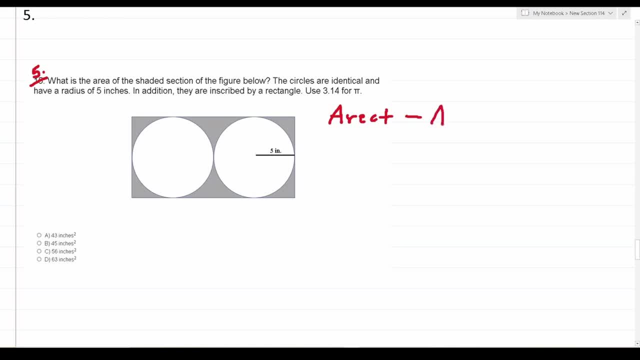 We're going to subtract the area of one of these circles, and I'm going to call that area of circle one, as well as the area of our other circle, which I'm going to call area of circle two. Now, since these circles are identical, we can actually just write this like: 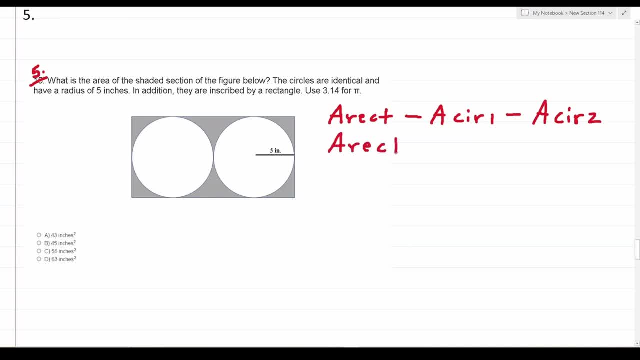 this area of our rectangle minus two times the area of circle one. Again, circle one And circle two are identical. Therefore their areas are the same. All right, Now how do we find the area of a rectangle? Of course, that's length times width. 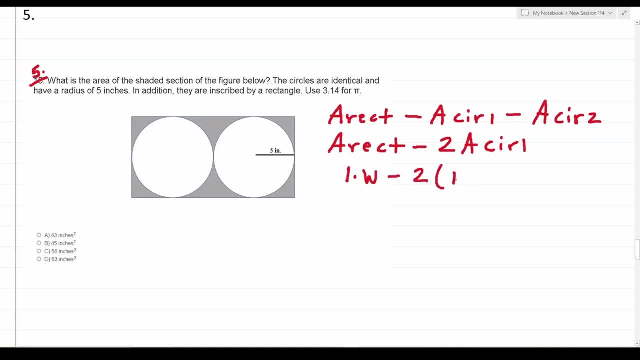 And how do we find the area of a circle? We should know by now that that's pi r squared. All right Again, according to the problem, we know what the radius of one of our circles is. It's right here, It's five. 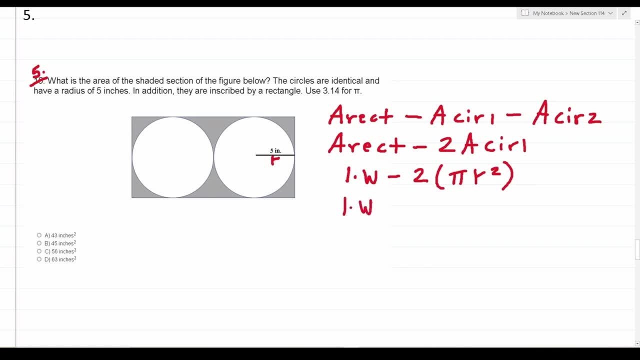 So let's go ahead and plug that in. This becomes length times width minus two Times pi five squared. Let's go ahead and work this out very quickly. This becomes length times width minus two times What is five squared. Five squared is 25.. 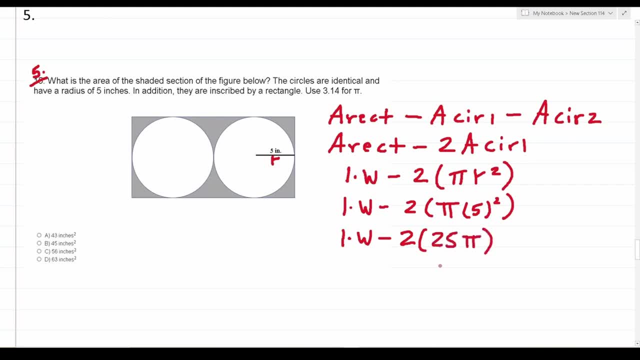 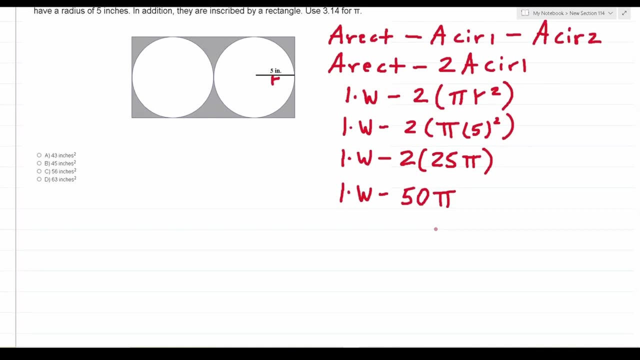 So this becomes 25 pi, And what is two times 25 pi? Well, that's going to be 50 pi, All right, So clearly we've worked this out as much as we can, And now we've hit a little bit of a roadblock. 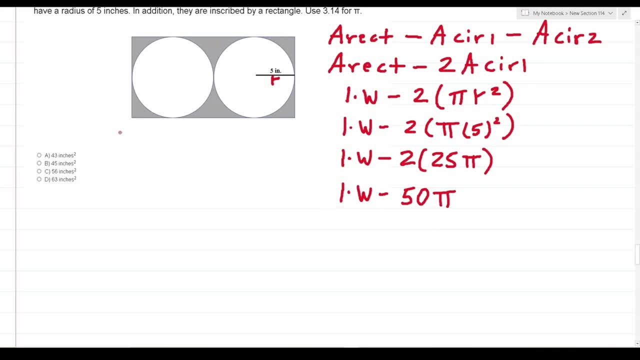 Insofar as we don't know what the length or width of this rectangle is. That said, using our knowledge of the definition of what a radius is, we can quickly figure out what L and W are. Again, as I said in this video, radius is defined as the distance from the center point of the circle. 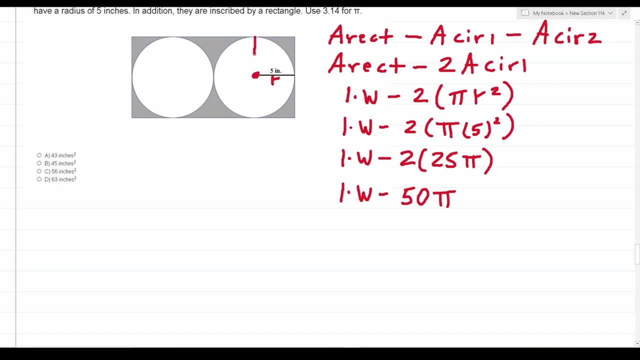 to the edge of the circle. So from here to here is a radius, And according to the problem, we know this circle has a radius of five. And from here to here is another radius, Again according to the problem, we know that that is five. 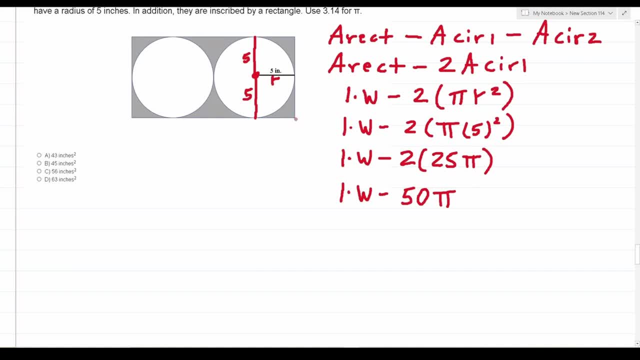 Clearly this is the same as the width of this rectangle, So we know width is going to be five plus five or ten. Again, using our definition of what a radius is, we can also find what the length of this rectangle is, Because from here to here is a radius. 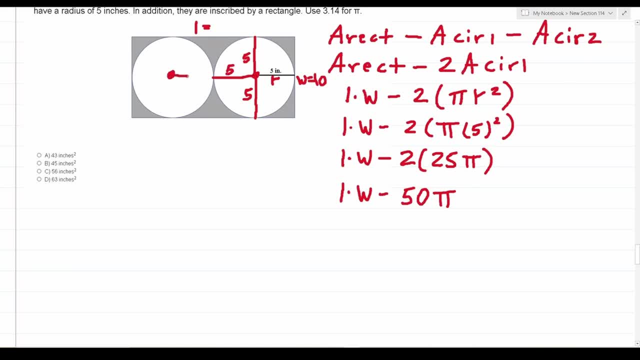 We know that's five. If we put our center point down, we know from here to here is five, And from here to here is five. So from here all the way to here is the same distance as the length of our rectangle. So that's going to be five plus five, ten plus five, fifteen plus five, twenty. 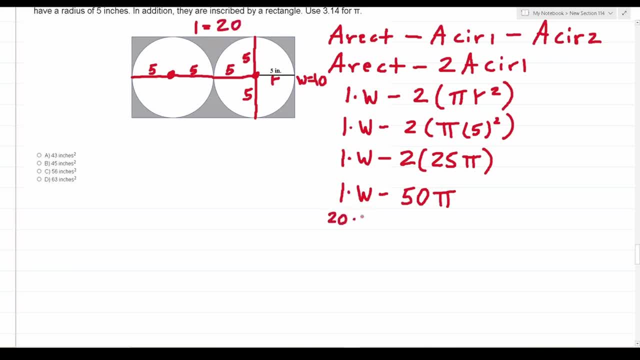 All right. So this becomes Twenty times ten minus fifty pi. Twenty times ten, that's fifty pi. Twenty times ten is going to be two hundred minus fifty pi. Now we have to figure out what fifty pi is. Again, according to the problem, we're going to approximate pi with three point one four. 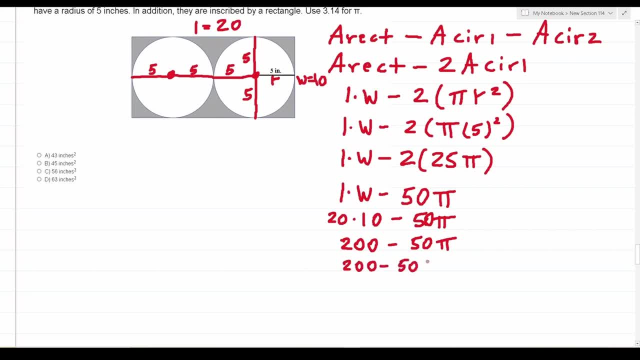 So this becomes two hundred minus fifty times three point one four, And I'm going to work that off To the side so as not to make any mistakes. we have fifty times three point one four. So what we want to do is take this decimal in three point one four and shift it one, two times to the right, such that this becomes three hundred and fourteen times fifty. 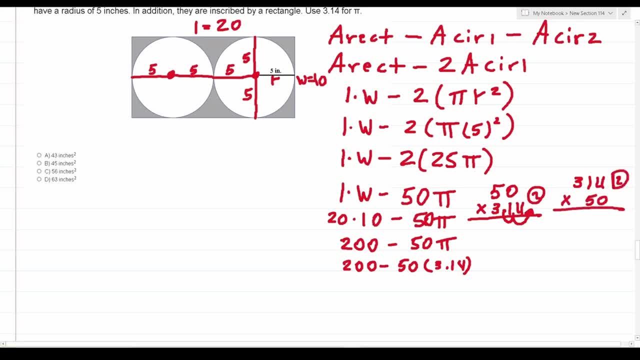 And once we work this out, we're going to take our two decimals that we move to the right here and shift them back into the left. So let's work this out: Four times zero is zero. One times zero is zero. Three times zero is zero. 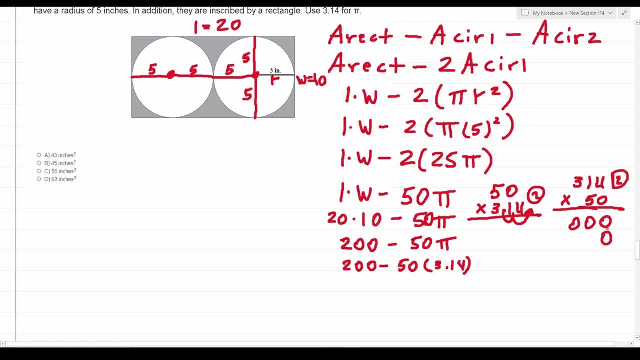 Before we start multiplication with that five, we have to bring in a zero placeholder. Five times four is twenty. So bring down a zero and carry a two. Five times one is five plus two is seven, And five times three is fifteen. Let's add these together. 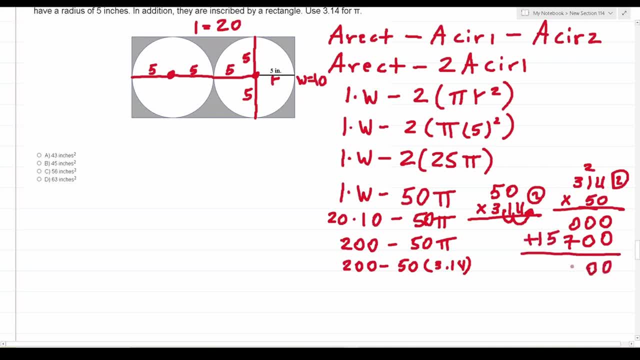 Zero plus zero is zero. Zero plus zero is zero. Seven plus zero is seven. Five plus nothing is five. One plus nothing is one. Let's bring our two decimals back in One, two, So this becomes two hundred minus one fifty seven. 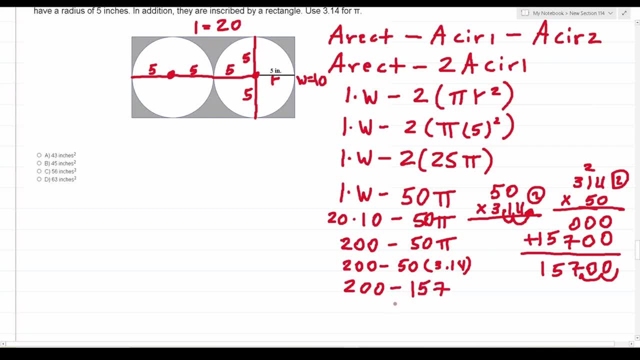 And if you can't do that in your head, let's go ahead and work that off to the side as well. We have two hundred minus one fifty seven, Zero minus seven. we can't do So. we have to look to the left to borrow. 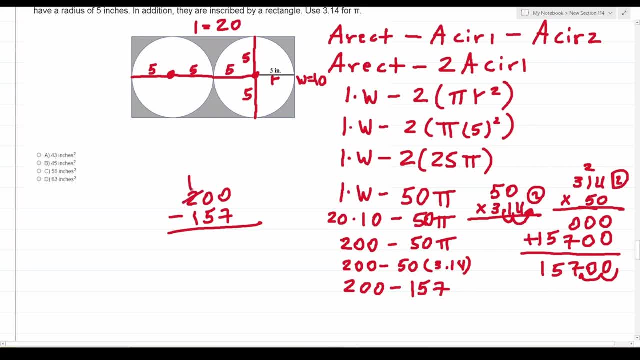 Can't borrow from a zero, So we're going to have to borrow all the way from this two. This is going to become one, This become ten. Borrow One more time. This become nine and this become ten. Ten minus seven is three. 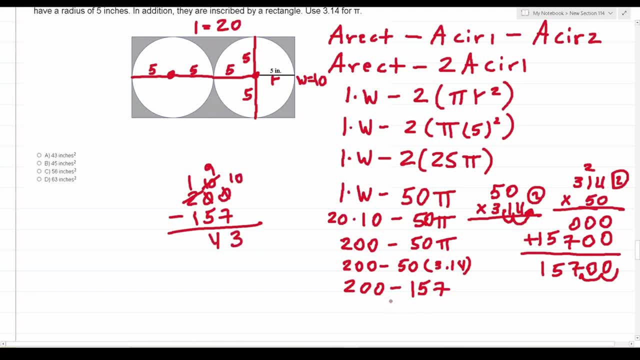 Nine minus five is four. One minus one is nothing, So this is forty three inches squared. In other words, the area of the shaded section of this figure is a forty three inches squared. All right, so That's a challenging problem. 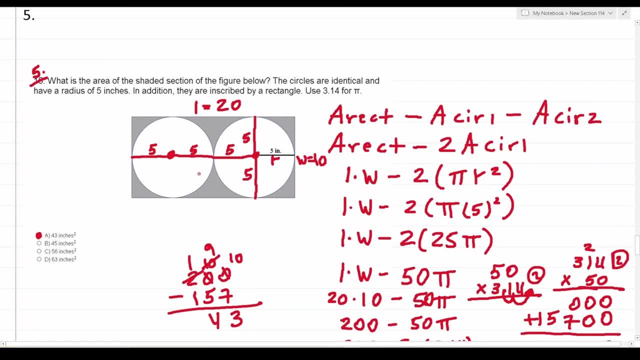 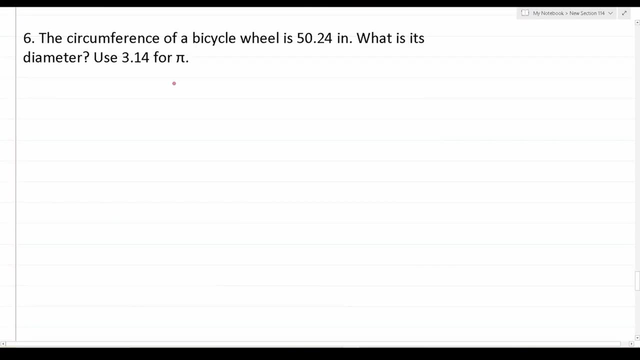 But that said again, if you use your knowledge of some basic principles of circles as well as rectangles, this problem was pretty simple and straightforward. All right, So that is that one, All right. So number six here says the circumference of a bicycle wheel is fifty point two, four inches. 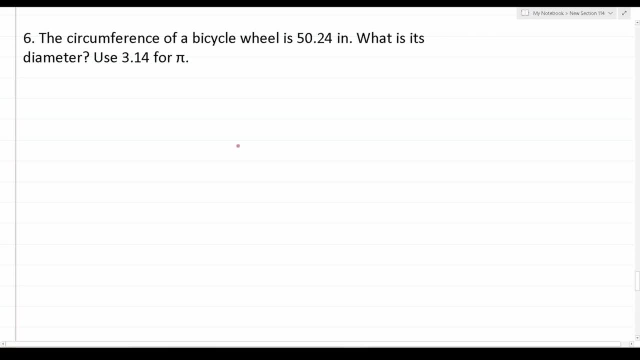 What is its diameter? Use three point one, four for pi. All right, So again we're given the circumference of this wheel. so we know we're going to be working with the circumference Formula. we want to know what its diameter is. 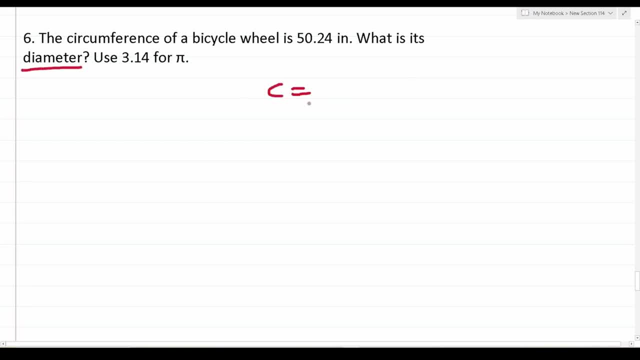 So of the two formulas to find the circumference of a circle we're going to use pi times diameter. This problem told us what C was. It said: circumference or C is fifty twenty four. So in place of C in our formula here I'm going to put fifty twenty four. 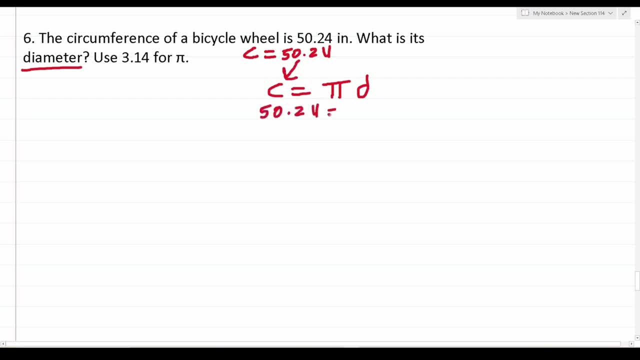 So this becomes fifty. twenty four equals What is pi? We're told to use three point one, four for pi, And that's times D for diameter. We're trying to solve for diameter. So what we want to do now Is get D by itself by dividing both sides by three point one, four. 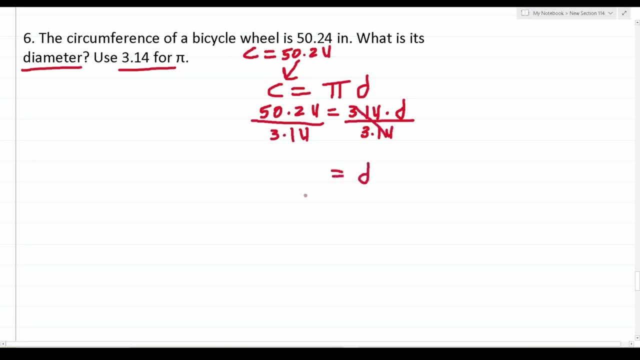 This will cross out over here, leaving us just D on this side, And, as you can see, D is fifty twenty four divided by three point one, four. In other words, by doing Fifty point two, four divided by three point one, four. 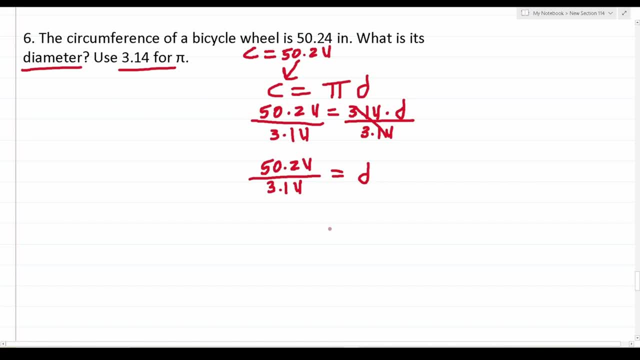 We'll know what the diameter of this bicycle wheel is. And in case you haven't worked with decimals in a long time, We can go ahead and write this first, like this: This says fifty Twenty four divided by three point one four. When you're dividing decimals like this, you can't have a decimal outside the division. 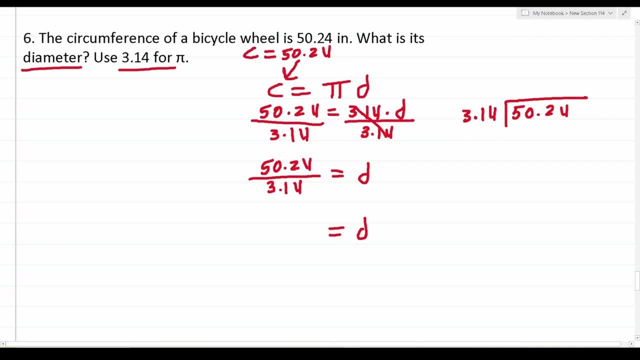 So what we have to do is we have to take this decimal in three point one, four and shift it one, two times to make three point one, four, three hundred and fourteen, And at the same time we're going to take this decimal inside the division bracket and shift it one, two times as well to make it five thousand and twenty four. 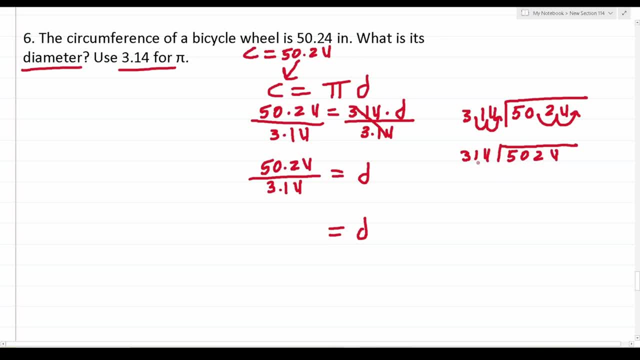 All right. So now that we cleared the decimal from outside the division bracket, We can go ahead and proceed As we normally would. We start by asking ourselves: how many times does three hundred and fourteen go into five? It doesn't. How many times does three hundred and fourteen go into fifty? 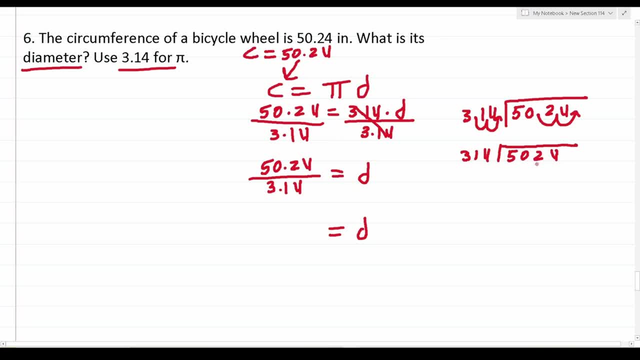 It doesn't. How many times does three hundred and fourteen go into five hundred and two without going over? Well, that's going to be one time Again. if this was three hundred times two, that would be six hundred, which is too big. 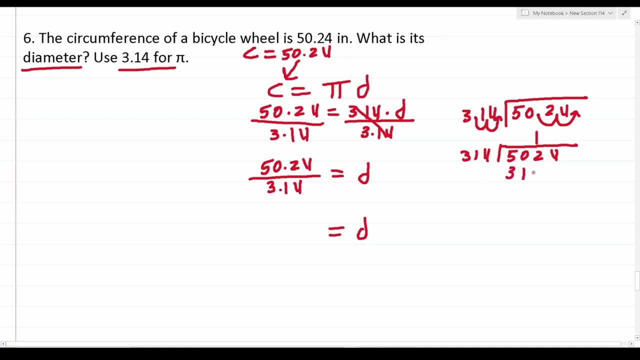 All right, So we know it's one. three hundred and fourteen times One is three hundred and fourteen. Let's go ahead and perform this Subtraction now: Two minus four. We can't do so. We're going to have to borrow. 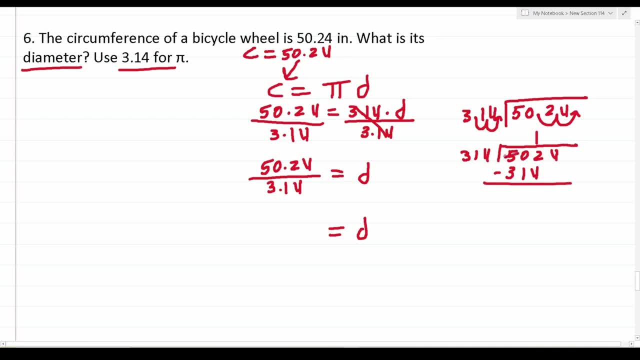 We have a zero here, So we can't borrow there. We're going to have to borrow from this five. This will become four, This become ten. We're going to borrow one more time. This become nine and this will become twelve. 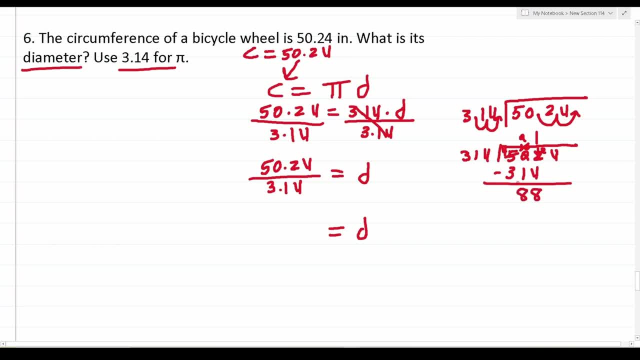 Twelve minus four is eight, Nine minus one is eight and four minus three is one. Now, of course, we got to drop down this four in the question Is this: how many times does three hundred and fourteen go into eighteen, eighty four, without going over? 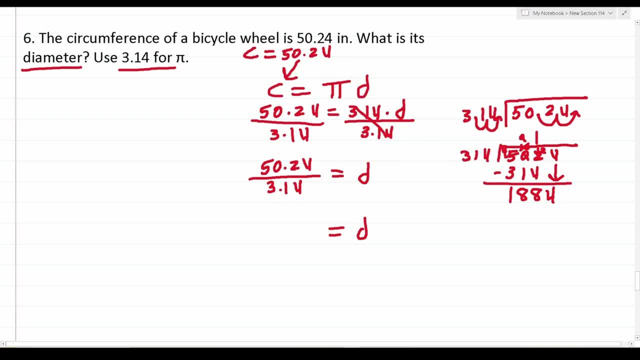 Well, let's use some estimation here. If this was three hundred and this was eighteen hundred, I would say three hundred times six would be eighteen hundred. So I'm going to say Three hundred fourteen is going to go into eighteen, eighty four, about six times, and before I write that six here, 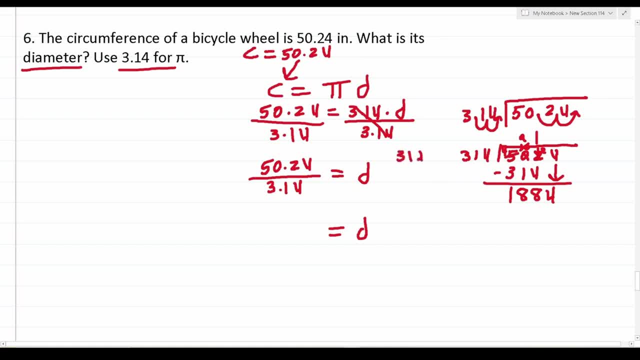 I'm going to work this off to the side to confirm it. We have three hundred and fourteen. We're multiplying that by six. Four times six is twenty four. So drop down a four, carry a two. One times six is six. plus two is eight, and three times six is eighteen. 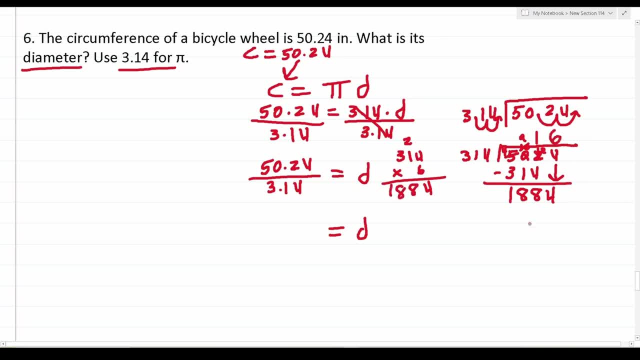 So three hundred and fourteen times six is eighteen, eighty four and there's no remainder. So the diameter Of this Circle that has the circumference of fifty twenty four is going to be sixteen, and in math we write the variable for which we solved on the left. 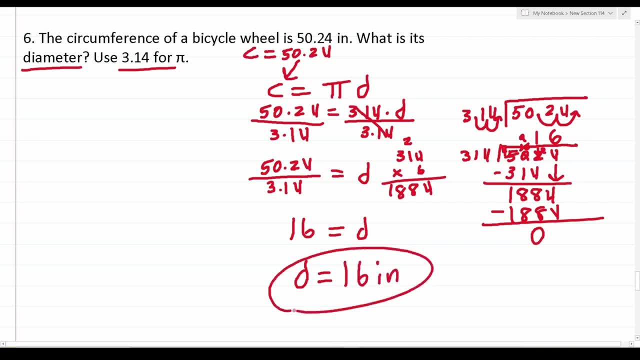 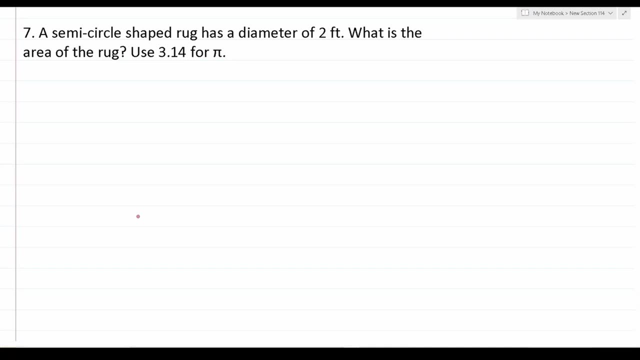 So this is going to be: D equals sixteen inches, All right. So again in this video you've had to work with decimals as well as fractions. There's no escaping that. on the ASVAB, All right. So number seven says a semicircle shaped rug has a diameter of two feet. 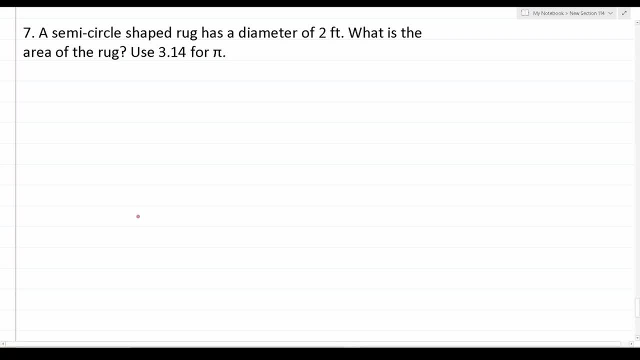 What is the area of the rug? We're going to use three point one, four for pi, All right. So in this video I've discussed how to find the area of circles, and we know that's. area equals pi, r squared. In this case we're working with a semicircle, and a semicircle is just a circle that's been cut right in half. 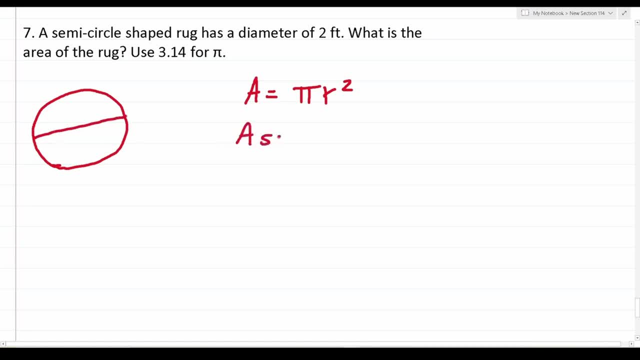 And, as you can imagine, to find the area of a semicircle, We're going to take the area of a circle which is pi? r squared And we're going to multiply that by one half. So in other words, we're going to be finding the area of this half of this circle, for instance. 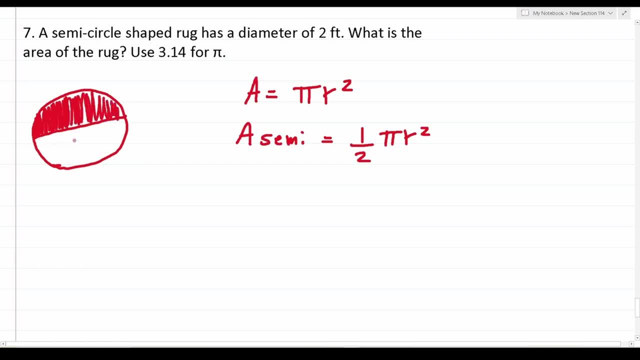 What's more, we know that the diameter of our rug is two feet. This case, so from here to here, is two feet. Well, as you can see, we need to know what the radius of our rug is In order to find it Area. 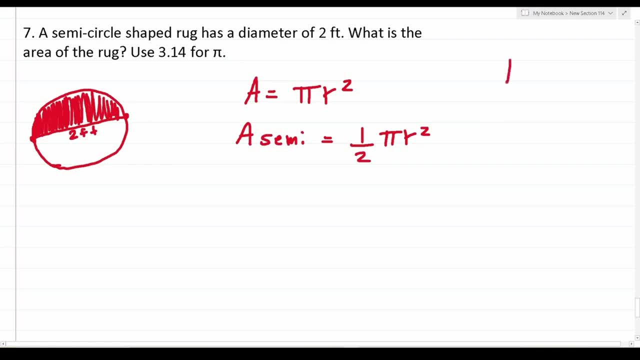 So we're going to fall back to this relationship. The diameter of a circle is always twice its radius. We know that the diameter of our semicircle is two feet, So that's two equals two r. If we divide both sides by two, we can get r by itself. 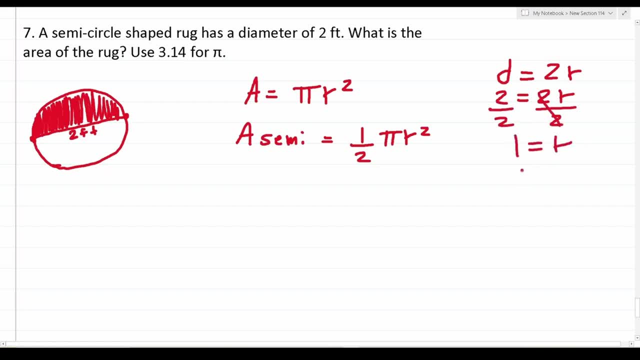 This crosses out there, leaving you with r. Two divided by two is one, So the radius of our semicircle is one. So now that we know what r is, We can go ahead and plug it in. Accordingly, this becomes one half. 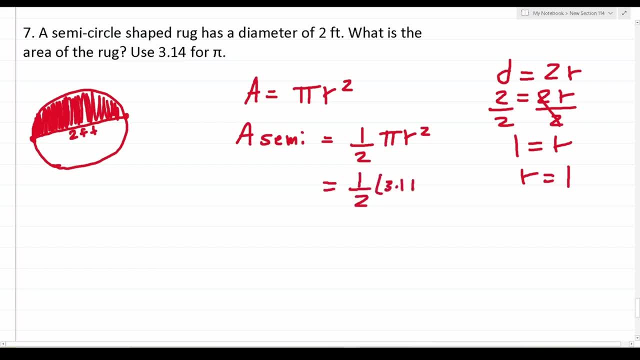 Again, pi is going to be three point one four, And this is going to be r of one squared. One squared is the same thing as one times one, So that's just one. So this becomes: one half equals r, one half times three point one four. 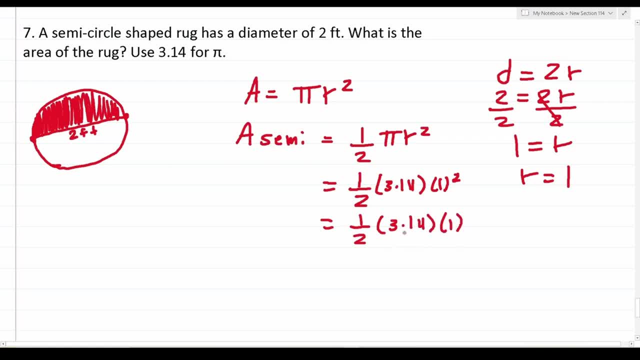 One squared is just one. Again, anything times one is just itself. So three point one. four times one is just three point one four. So this becomes one half times three point one four. Alright, so there are two approaches you can take to solving this. 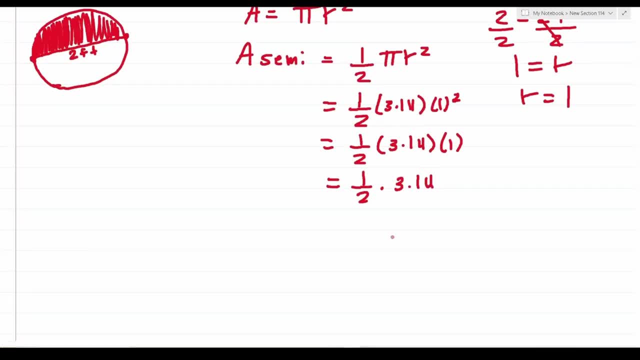 I've worked with circles so much that I know the answer is going to be one point five seven. Again, half of three. point one four is one point five seven. That said, if I was working this out on my own I would do this. 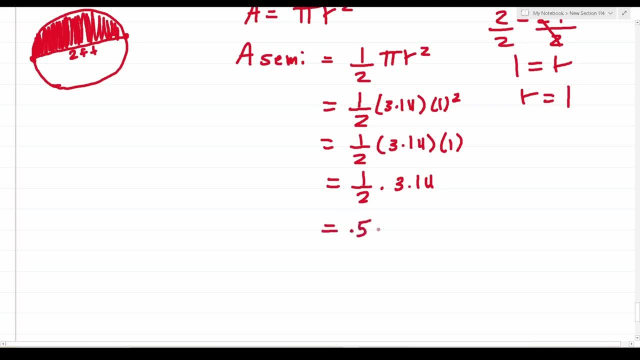 I would know one half is the decimal equivalent of point five. So this would be point five times three, point one, four, And then I would work this off to the side like this: Three point one, four times point five. And now we've got to clear these decimals. 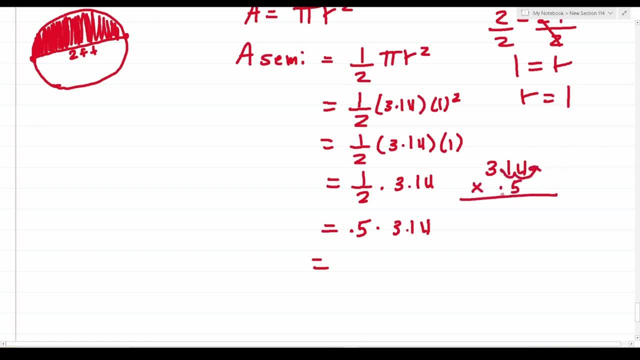 I've got to move the decimal place one, two times here and one time here. So in total I move the decimal place three times to make this three hundred and fourteen times five. Once I work this out without decimals, I'm going to take my decimal place and move it three times to the left. 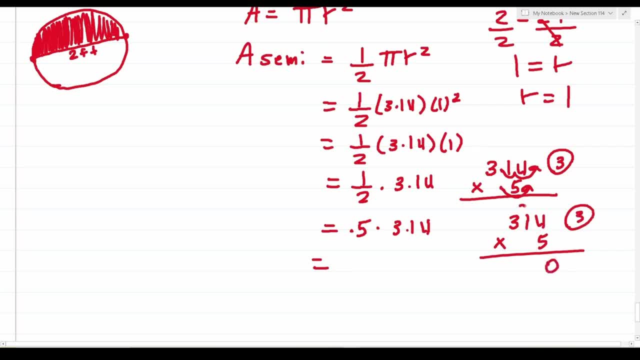 Alright. so four times five is twenty. Carry a two, Five times one is five plus two is seven, And three times five is fifteen. Bring our three decimals back in One, two, three, So we can see that point five times three, point one four is going to be one, point five, seven. 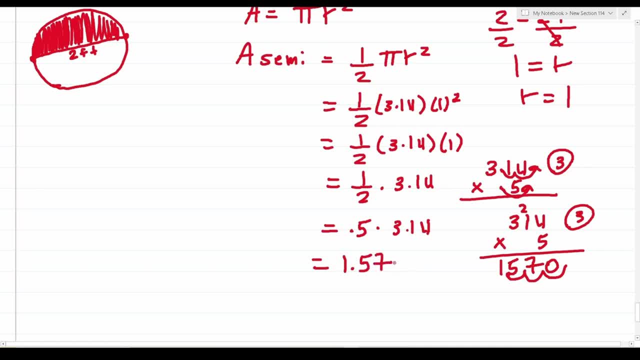 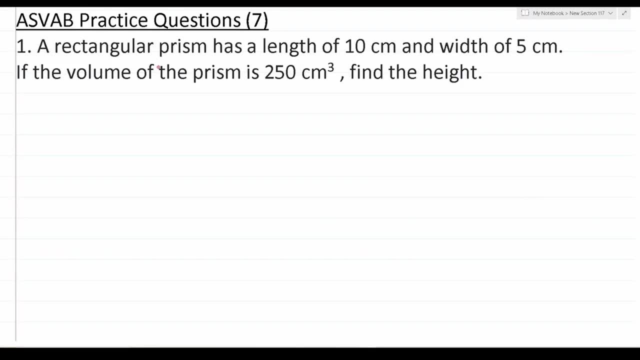 So the area of our semicircle is one point five seven, And this is going to be feet squared. This first one says a rectangular prism has a length of ten centimeters and a width of five centimeters. If the volume of the prism is two hundred and fifty centimeters cubed, find the height. 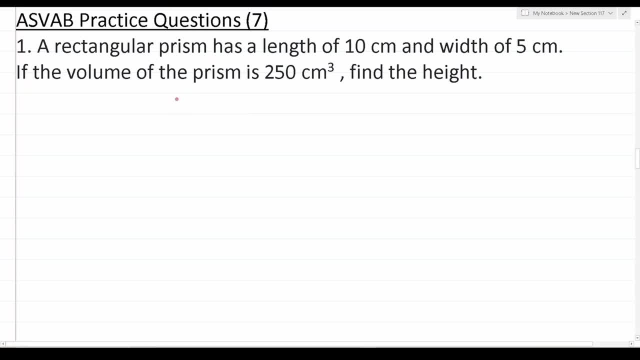 So of course you have to know that to find the volume of a rectangular prism, It's length times width times height. And according to this problem, our rectangular prism has a length of ten, a width of five and an unknown height, So we don't know what its height is. 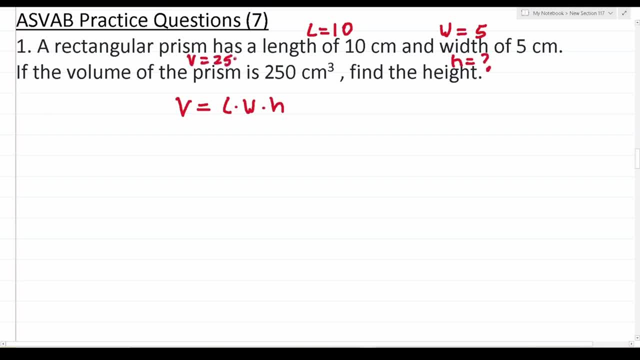 In addition, we were told that its volume is two hundred and fifty centimeters cubed, So let's plug those values in accordingly. Again, we were told that its volume is two hundred and fifty. So in place of b here I'm going to put two fifty. 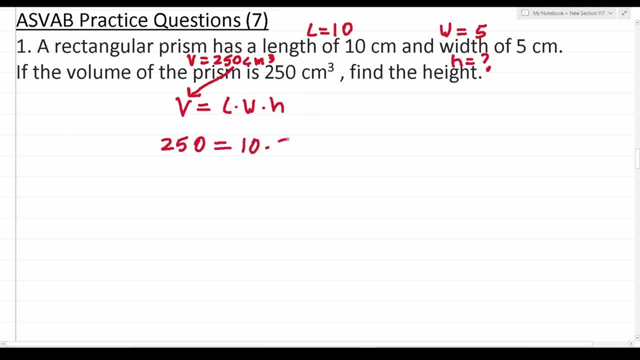 We know it has a length of ten. So this is ten, a width of five and an unknown height. So we'll just leave that as h And clearly by solving this equation for h We'll be able to answer this question. 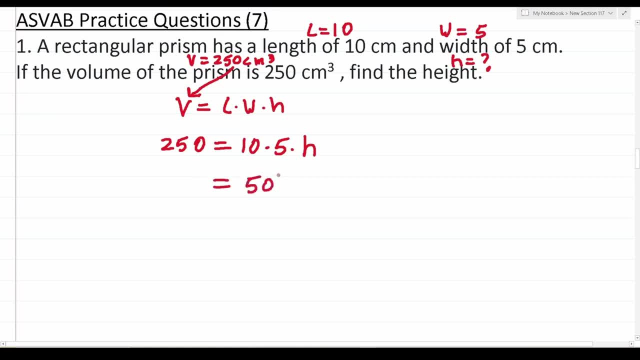 So let's go ahead and do that. Ten times five is going to be fifty, So this is fifty. h equals two fifty. To get h by itself, we'll divide both sides by fifty. now This crosses out here, leaving you with h on this side. 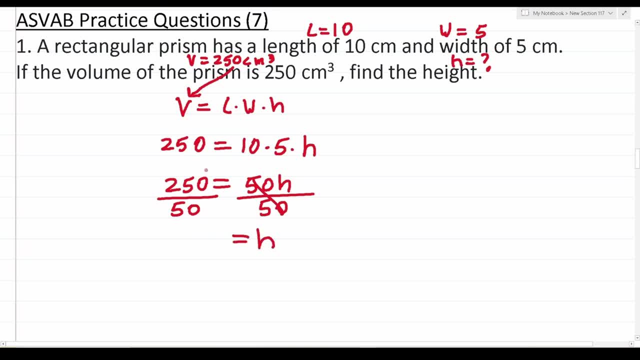 And this math is actually incredibly easy to do. You can cross out these corresponding zeros. What is twenty five divided by five, That's five. So the height Of our rectangular prism has to be five centimeters. All right, So that is that one. 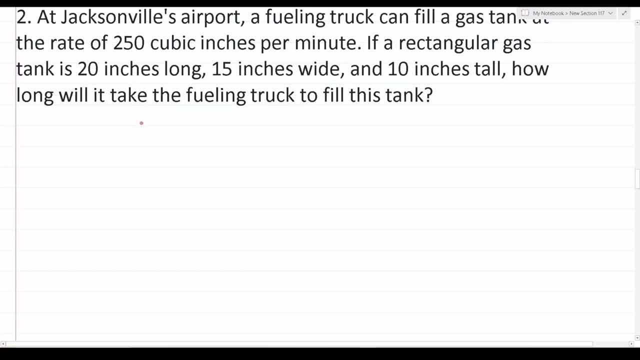 All right. So number two says: at Jacksonville's airport A fueling truck can fill a gas tank at the rate of two hundred and fifty cubic inches per minute If a rectangular gas tank is twenty inches long, fifteen inches wide and ten inches tall. 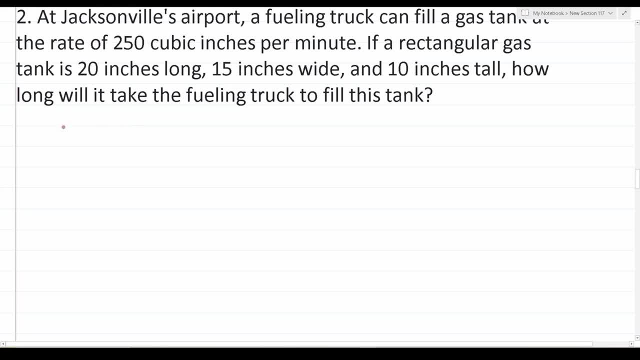 How long will it take the fueling trunk to fill this tank? All right, So we're going to be finding the volume Of our rectangular gas tank And since it's a rectangular gas tank, we know it's going to be a rectangular prism. 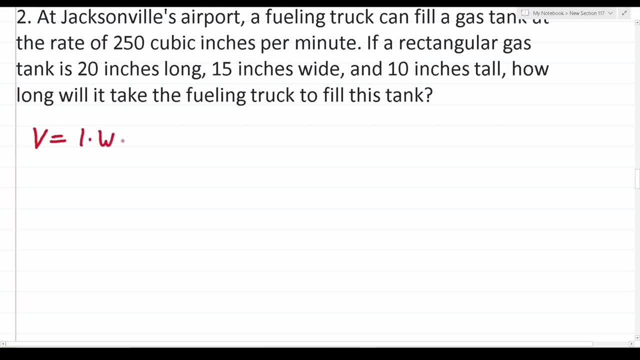 The volume of a rectangular prism is length times width times height And thankfully enough we were given all those things in this problem. We know our rectangular gas tank has a length of twenty inches, So L is twenty. Width of fifteen, So W is fifteen. 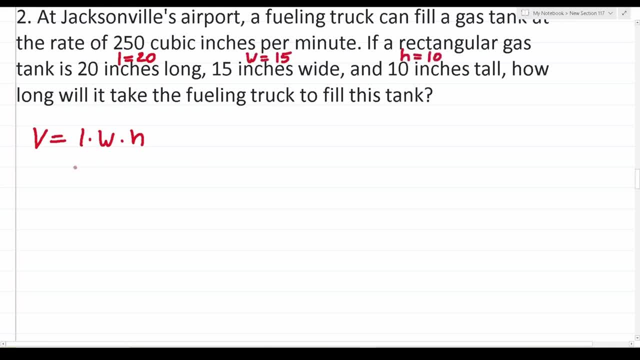 And a height of ten. So let's go ahead and plug those values in. This becomes twenty times fifteen times ten, And you could do this one mentally if you wanted to. You could say: Twenty times ten is two hundred. So that leaves us with two hundred times fifteen. 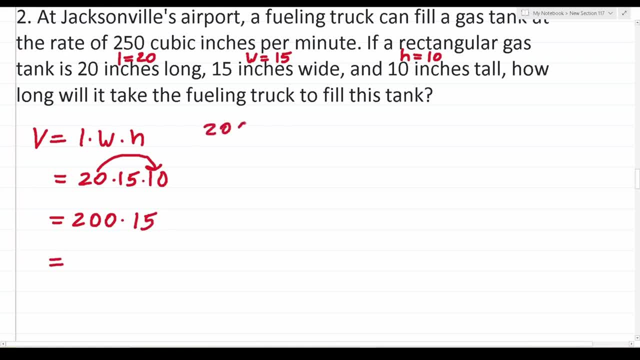 And at this point I might work this off to the side- to be two hundred times fifteen. Zero times five is zero. Zero times five is zero. Five times two is ten. Before you start multiplication with that one, you want to bring in a zero placeholder. 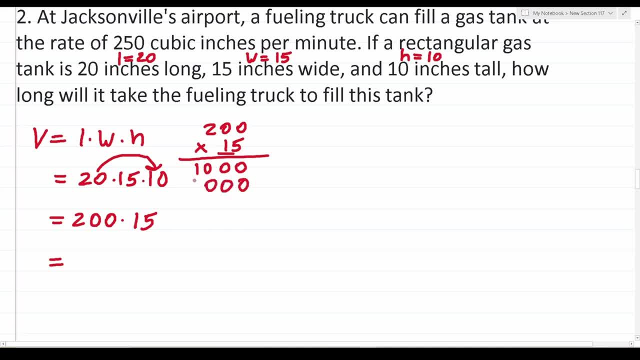 One times zero is zero. One times zero is zero. Two times one is two. So right here we have one thousand plus two thousand, which is three thousand. All right, So the volume of our rectangular gas tank is three thousand cubic inches. 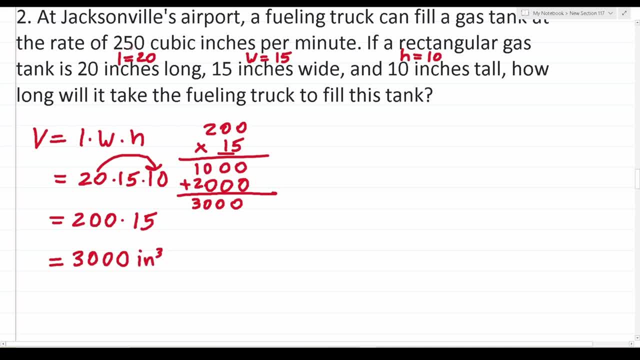 Now let's go back to the other part of this problem, where it says the fueling truck can fill a gas tank at a rate of two hundred and fifty cubic inches per minute. So to figure out how long it's going to take this truck to fill up our tank. 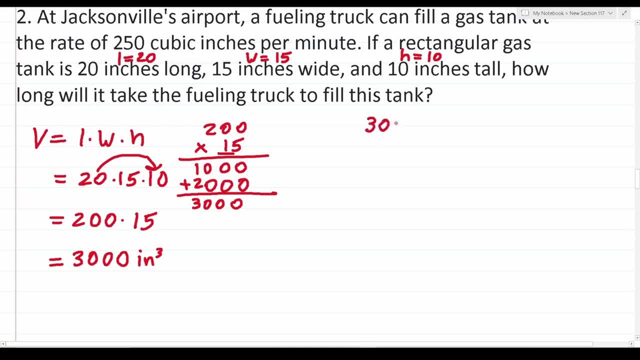 we're going to take the volume of our tank, Which is three thousand, and we're going to divide that by how much volume of gas this fueling truck puts into the tank per minute, which is going to be two fifty, All right. 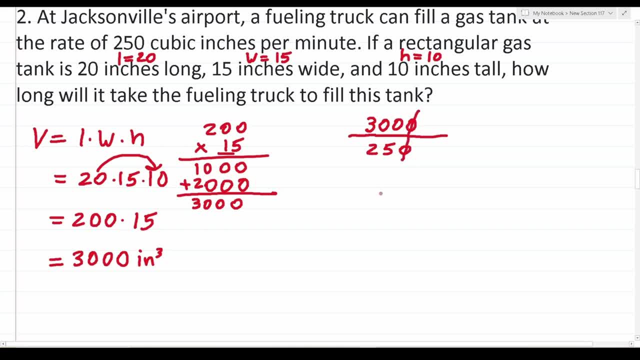 So let's cross out these corresponding zeros to make this math a little bit easier. And you should be able to do this mentally, But if you couldn't, you could always read this as three hundred divided by twenty five, And when you do long division, you start by asking yourself this: 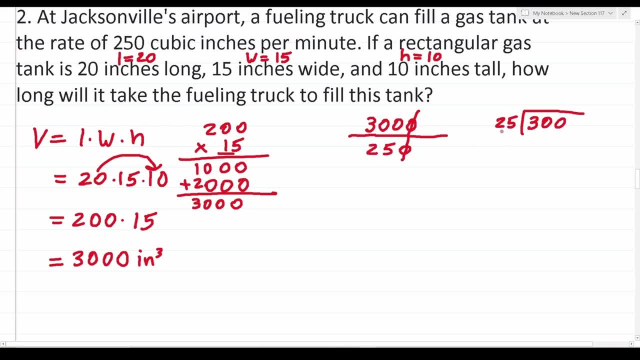 How many times does twenty five go into three Doesn't. How many times does twenty five go into thirty without going over? Well, that's going to be one time. Twenty five times one is twenty five. Thirty minus twenty five is going to be five. 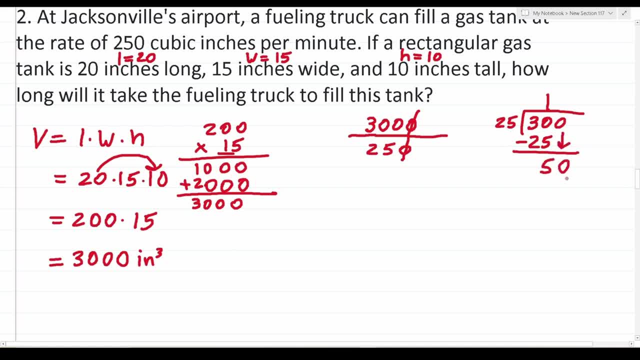 Drop down this zero. Now the question is: how many times does twenty five go into fifty without going over? That's going to be two times. Given that, two times twenty five is fifty. Fifty minus fifty is zero. So three hundred divided by twenty five is twelve. 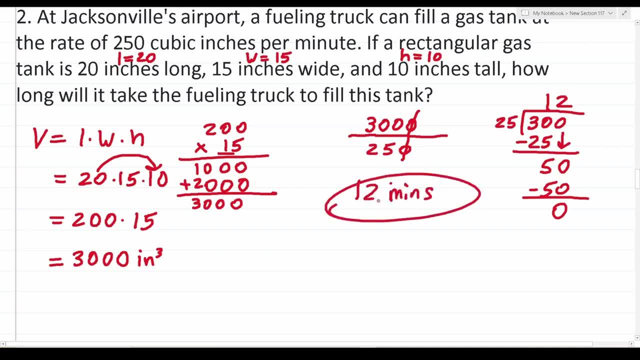 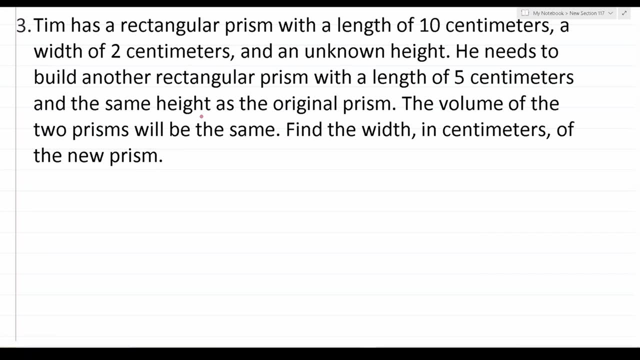 In other words, it takes twelve minutes for this fueling truck to fill up our rectangular gas tank. So that is that one, All right. So number three says Tim has a rectangular prism with a length of ten centimeters, a width of two centimeters and an unknown height. 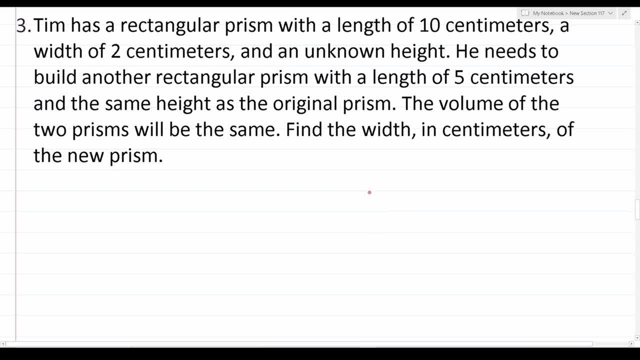 He needs to build another rectangular prism with a length of five centimeters and the same height as the original prism. The volume of the two prisms will be the same. Find a width in centimeters of the new prism, All right, So there's quite a bit going on in this problem. 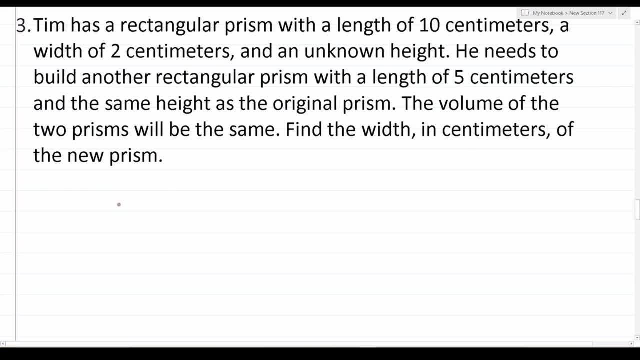 And let's take it step by step. First of all, let's talk about finding the volume of this first prism. So I'm going to call that volume prism one. Well, we know how to find the volume of rectangular prisms, That's length times width times height. 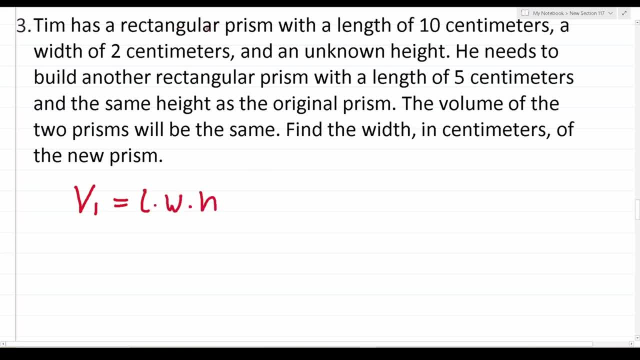 And let's see what was given. according to this problem Has a rectangular prism with a length of ten. so we know L is ten and a width of ten A width of two, So W is two. Height is unknown according to the problem. 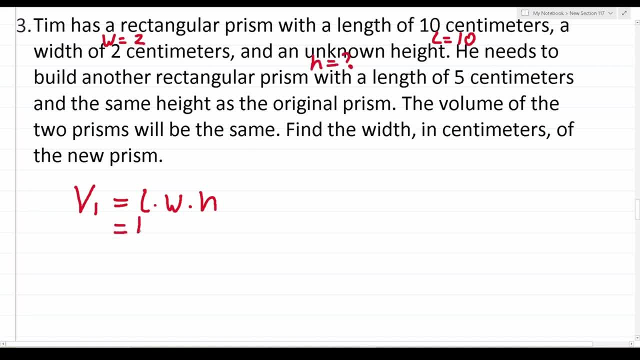 So let's plug those values in. We have a length of ten, So this is ten. a width of two, So that's two, And the height is unknown, So we'll leave that as H Ten times two is going to be twenty. 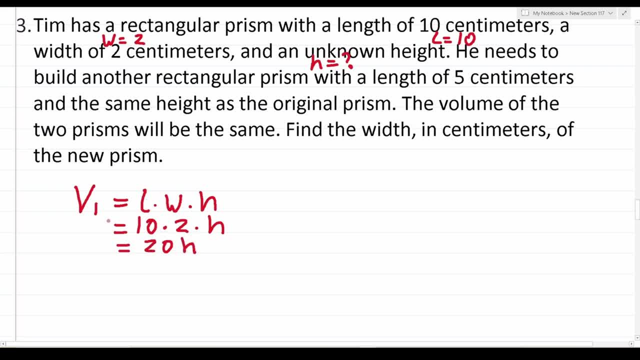 So this is twenty H. The volume of our first prism is twenty H. All right, And that's all we can get from that, And let's go ahead and take a look at the second part of this problem. He wants to build another rectangular prism. 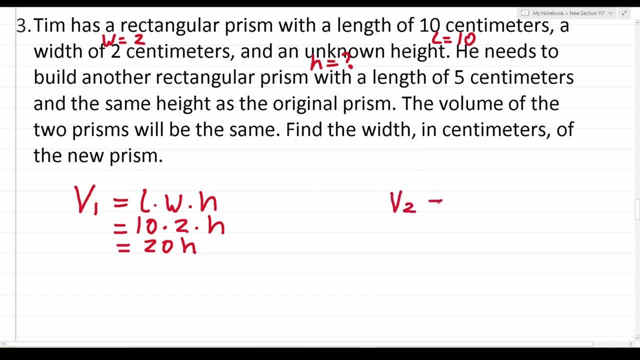 So we're going to be finding the volume of a second rectangular prism, which I'm going to call V2.. And we know how to find the volume of rectangular prisms: It's length times width, times height, With a length of five. 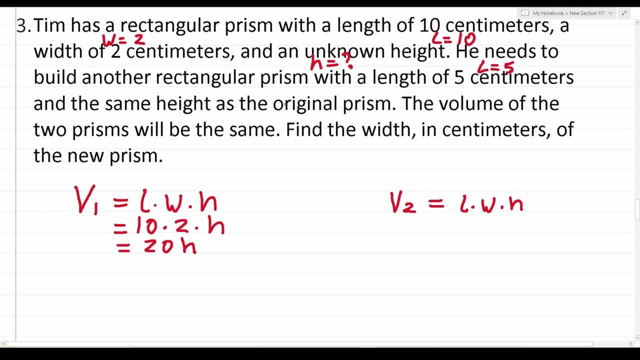 So L is five and the same height as the original prism. The volume of the two prisms will be the same. So let's try to express that mathematically: The volume of this first prism has to equal the volume of this second prism. 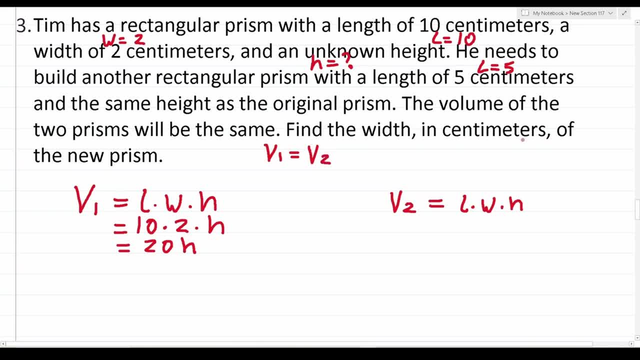 Find the width in centimeters of the new prism. All right, So let's go ahead and fill this in. We know that the length of our new prism is five. We're trying to figure out what its width is, And we're told that its height is the same as this height. 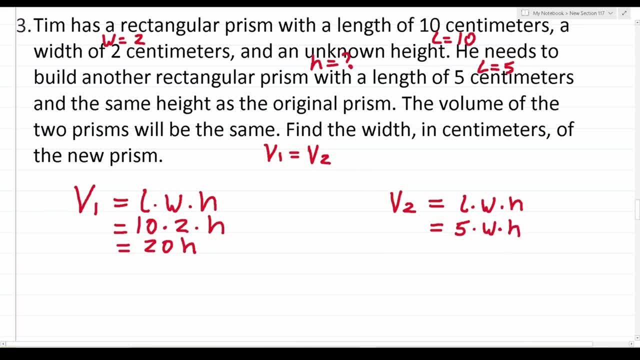 So we're going to have to leave that as H for the time being. That said, we know the volumes of these two prisms are the same. So the volume of prism one was 20H. That means the volume of prism two is also going to be 20H. 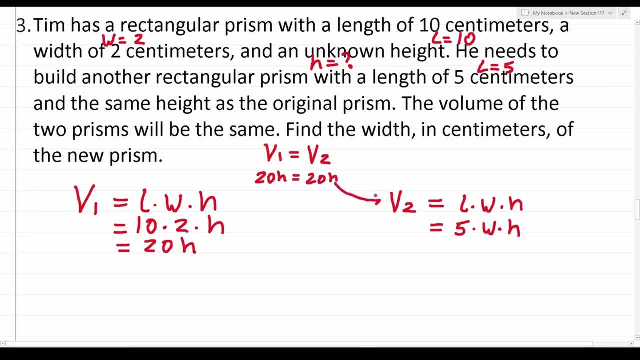 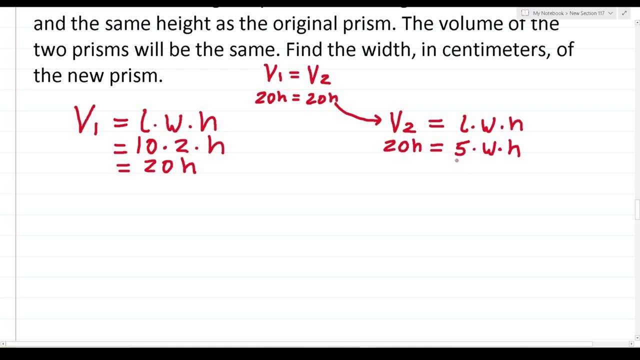 So in place of V2 here, I can go ahead and plug in 20H, So this becomes 20H equals five times width, times height, And it should be pretty clear now that we're going to be solving for W. And if we divide both sides by five, H. 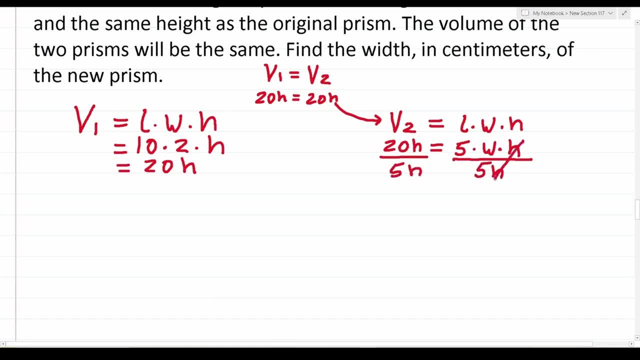 Let's see what happens. Well, this H crosses out here and these fives cross out here, leaving you with W on this side. These H's cross out here, and 20 divided by five is four, So the width of the second rectangular prism is going to be four centimeters. 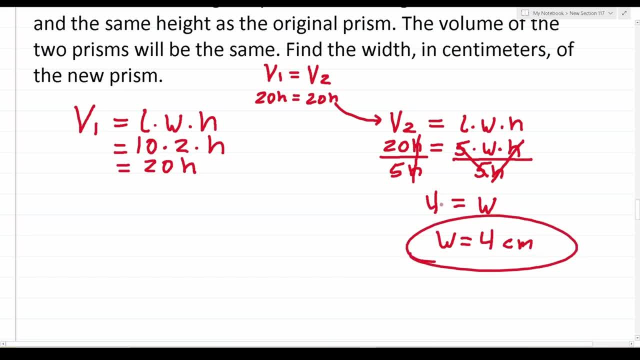 All right, That is that one pretty challenging. But that said, if you understand how to find the volume of a rectangular prism and you follow the instructions in the word problem, it's not that difficult at the end of the day. All right. 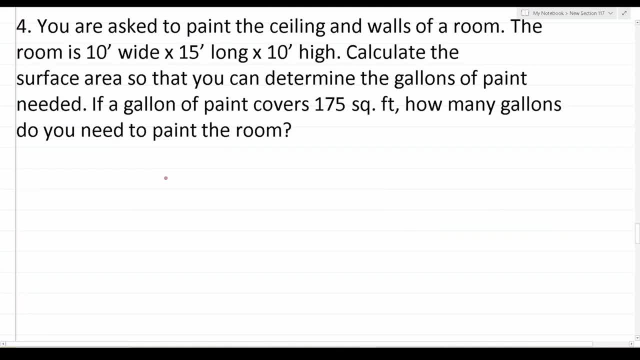 So number four says you are asked to paint the ceiling and walls of a room. The room is 10 feet wide, 15 feet long and 10 feet high. Calculate the surface area so that you can determine the gallons of paint needed If a gallon of paint covers one hundred and seventy five square feet. 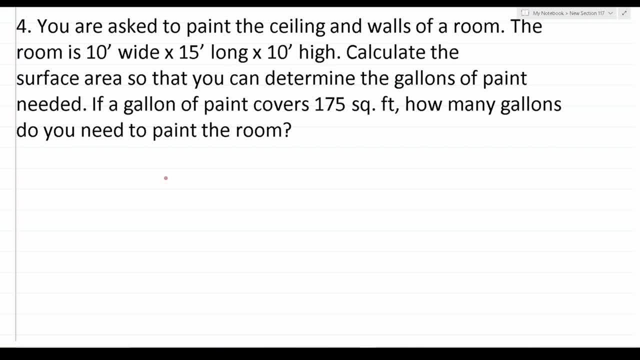 how many gallons do you need to paint the room? All right, So clearly we're going to be finding surface area of this room. So to find the surface area of a rectangular prism, you may recall that surface area equals two length times width plus two width. 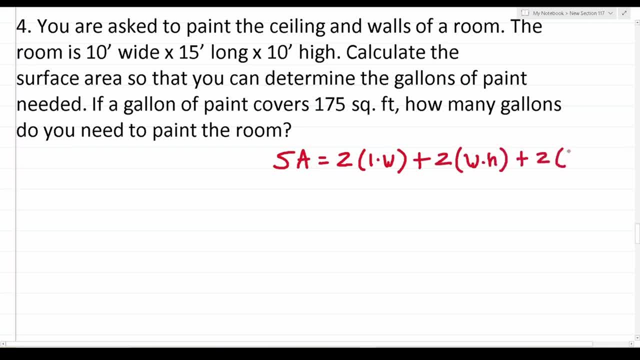 times height plus two height times length, And again, each of these is the area of the six faces of our rectangular prism. Now let me go ahead and take a rectangular prism and unfold it for you, because we're going to have to pay close attention. 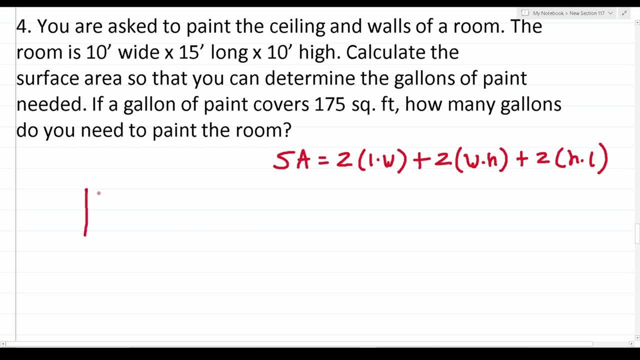 to the wording of this problem, to get it correctly. So here is our floor of our rectangular prism. That means that this is the back wall, This is our front wall, This is our side wall, This is our side wall And this is our ceiling. 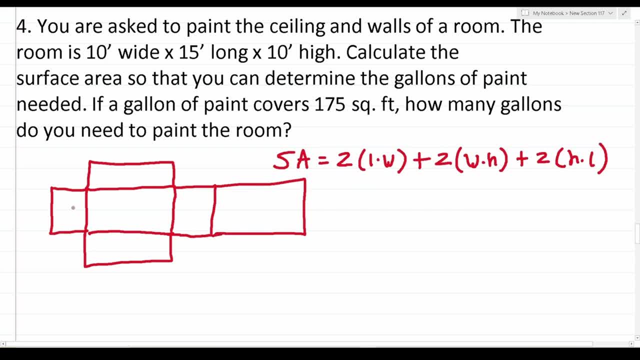 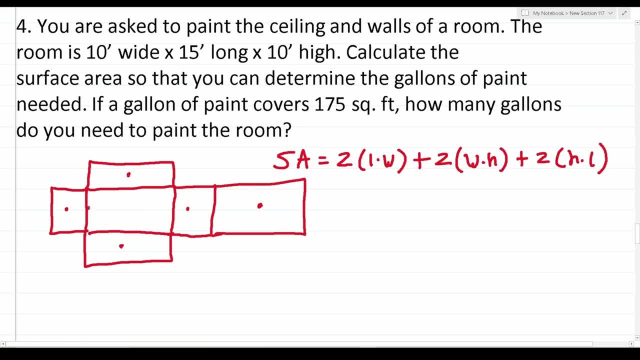 And what is the area of this floor? Well, we have a width here And a length here, So the area of this floor is length times width. So here's the modification we're going to make: This is going to become surface area. 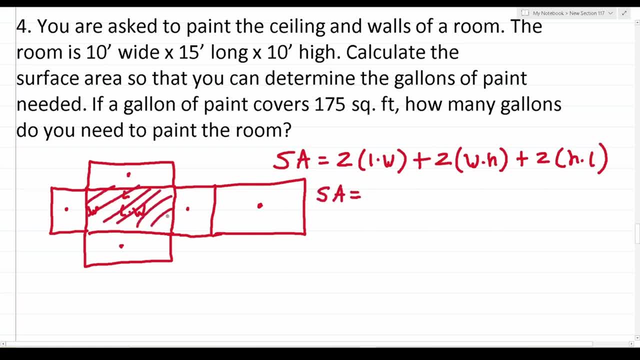 Again, we're excluding the floor, which is one of these lengths times widths. This ceiling is also length times width, So we need one of those. So this is going to become length times width plus two width times height plus two height times length. 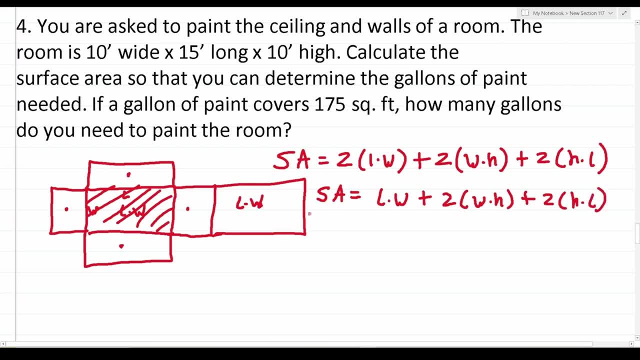 All right. So that's why I unfolded that rectangular prism. So you can see that we have to exclude the floor which we are not painting, which means we have to remove this two here and just leave it as length times width. All right. 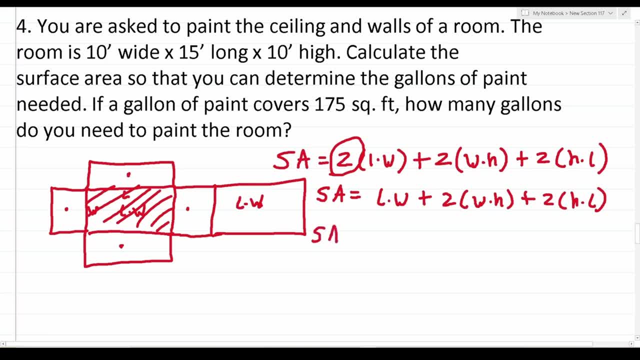 So, with that done, let's go ahead and plug in values accordingly. We know what they all are. W is 10, L is 15 and H is 10.. So W is 15.. So this becomes 15 times. width is 10 plus two. 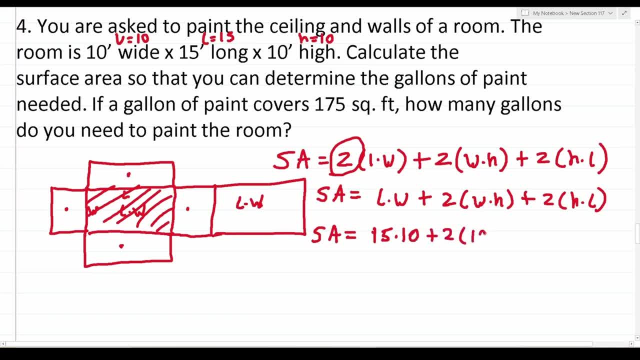 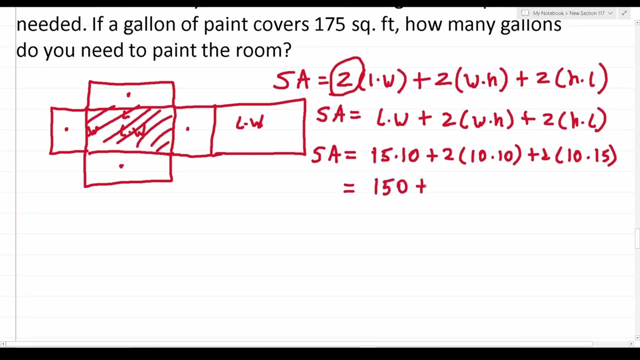 Width is 10.. Height is 10 plus two. Height is 10 and length is 15.. All right, Let's go ahead and work this out. This is going to be pretty easy to do. mentally: 10 times 15 is going to be 150. 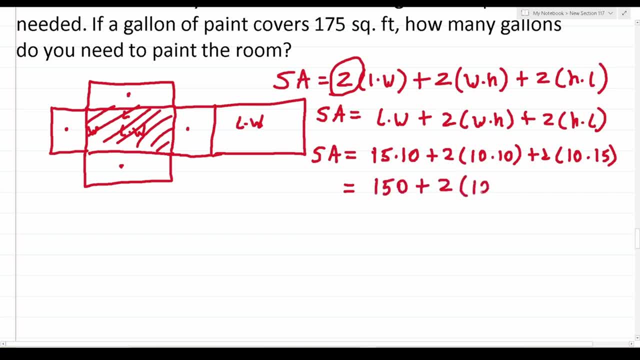 This is going to become two times 10 times 10 is 100.. And 10 times 15 is going to be 150.. So this is two times 150.. Let's go ahead and keep working this out. This is 150 plus two times. 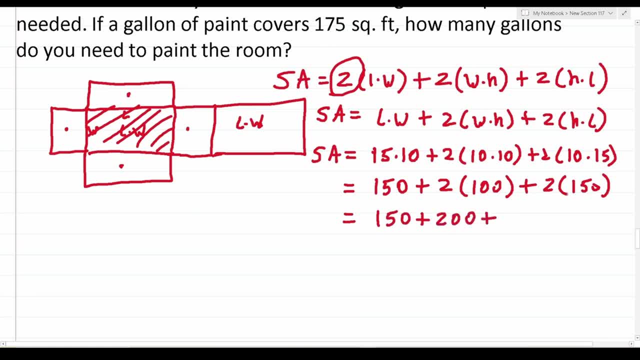 100 is going to be 200.. Two times 150 is going to be 300.. 150 plus 150 is 300.. Let's keep working this out. This is 200 plus 300, which is 500.. So this is 500 plus 150.. 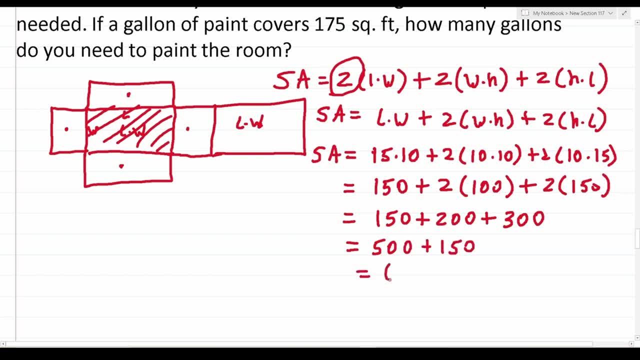 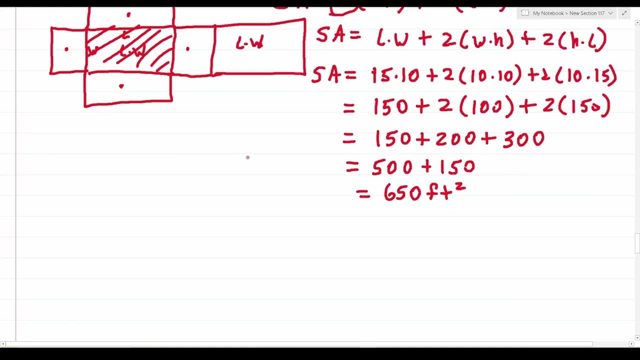 So this is going to be 500 plus 150, which is 650.. All right, So the total surface area that we're going to be painting is 650 square feet. All right, So we know that we're painting 650 square feet of wall and ceiling space. 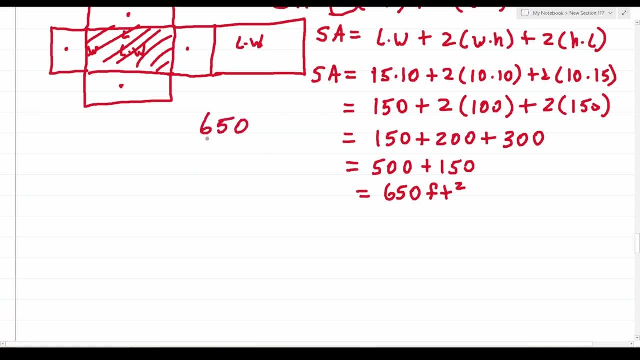 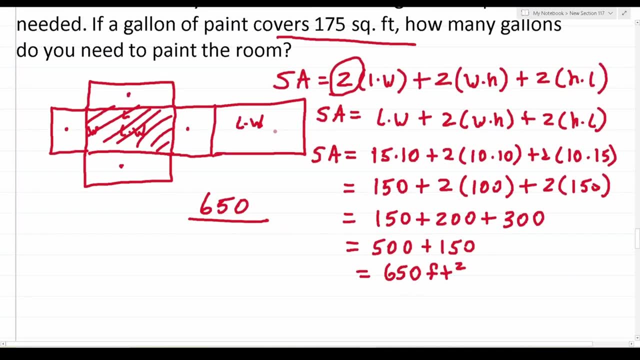 So this is going to be 650.. And we're going to divide that by how many square feet each gallon of paint covers. According to the problem, each gallon of paint covers 175 square feet. So by doing 650 divided by 175, we'll. 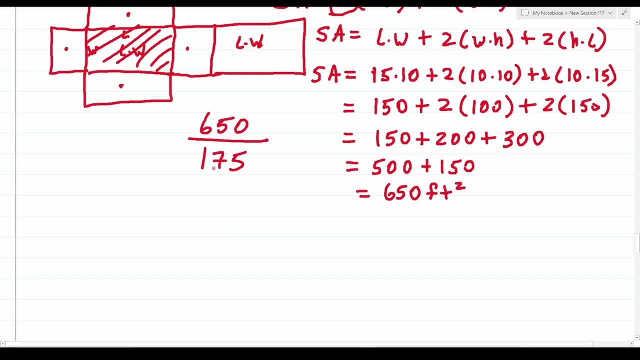 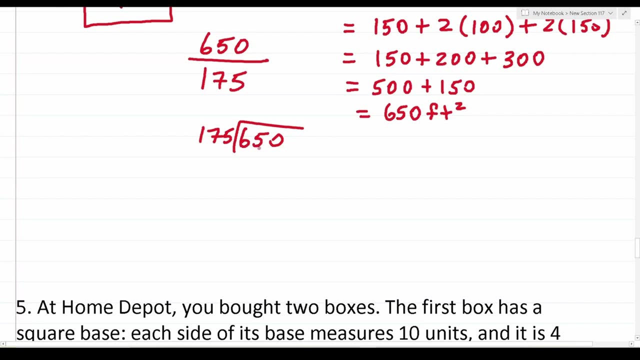 know how many gallons of paint we need, And we could read this as long division like this: 650 divided by 175.. And we start by asking ourselves: how many times does 175 go into six? It doesn't. How many times does 175 go into 65?? 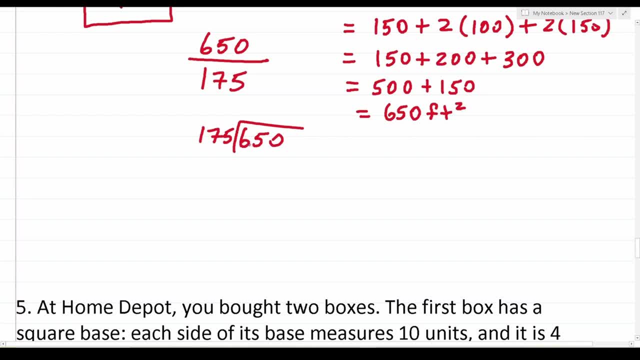 It doesn't. How many times does 175 go into 650 without going over? Well, it's going to either be three or four times, So I'm going to say It's three, But I'm also going to work out 175 times three and 175 times four. 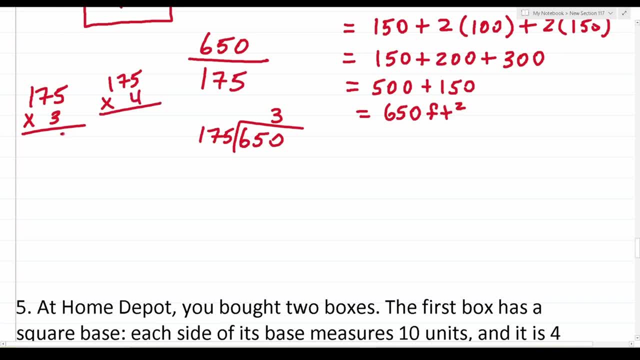 Just to confirm that Five times three, of course, is 15.. So drop down a five, carry a one. Seven times three is 21 plus two is 22.. Drop down a two, carry a two. Three times one is three plus two is five. 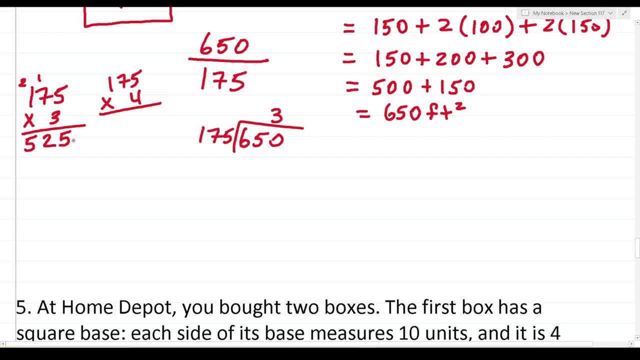 So three gallons of paint covers 525.. Square feet: What about four? Five times four is 20.. So bring down a zero, carry a two. Seven times four is 28,, 29,, 30. Bring down a zero, carry a three. 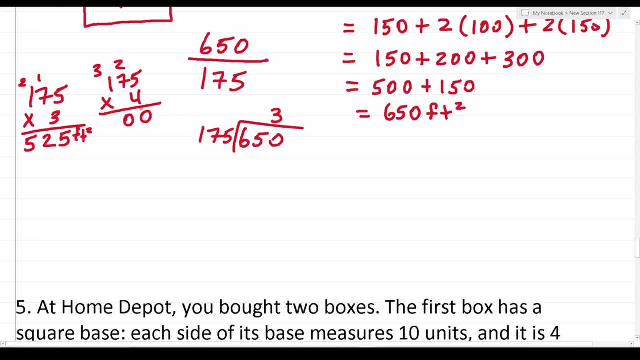 Four times one is four plus three is seven. So four gallons of paint covers 700 square feet of area. So clearly, if I were to do this long division here, this would be 3.7 something, and so on and so forth. 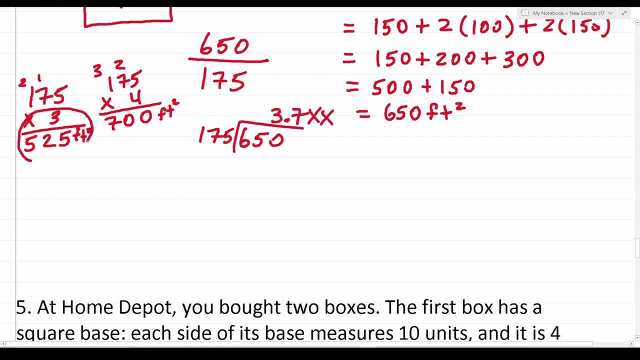 But it should be pretty obvious that if you get three gallons of paint, you're only going to be able to cover 525 square feet, which is not enough to cover our 650 square feet. So that means you're going to have to buy four gallons of paint. 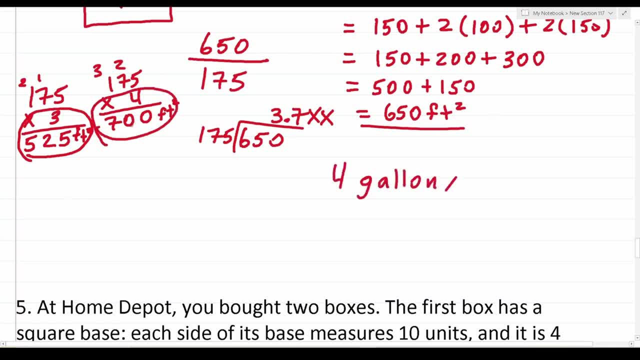 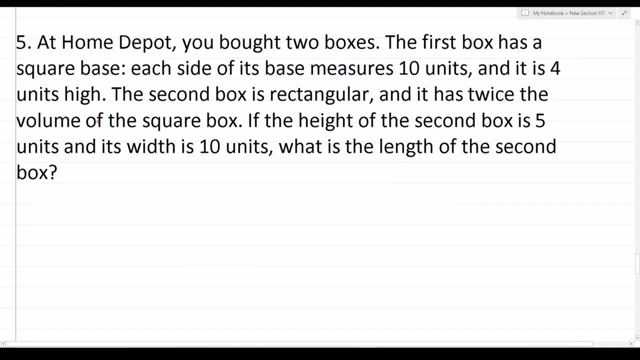 which will cover 700 square feet, And that's going to be enough to cover our 600 square feet for our walls and our ceiling. So the answer to this one is four gallons, All right. So number five says: at Home Depot you bought two boxes. 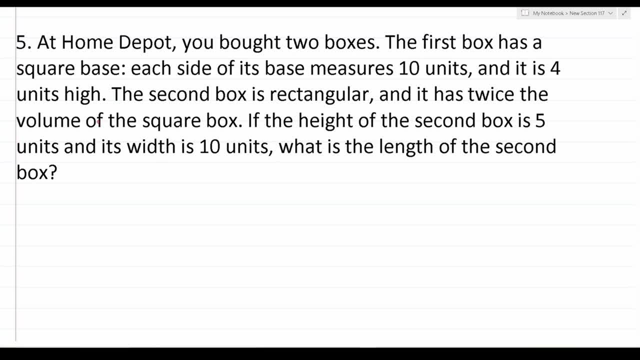 The first box has a square base. Each side of its base measures ten units and it is four units high. The second box is rectangular and it has twice the volume of the square box. If the height of the second box is five units and its width is ten units, 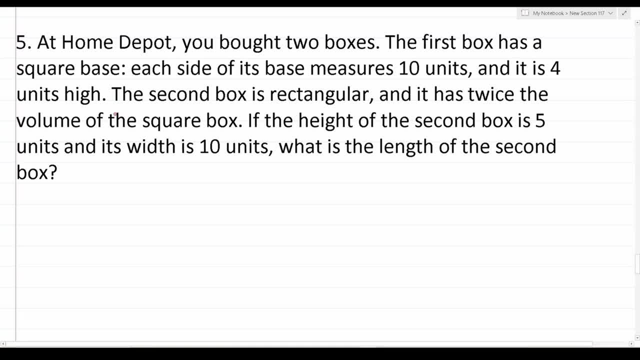 what is the length of the second box? All right, So I know we're talking about boxes And when people hear the word box they automatically think of cubes, But in this case we're actually working with two rectangular prisms And, more specifically, we're working with the volume of two rectangular prisms. 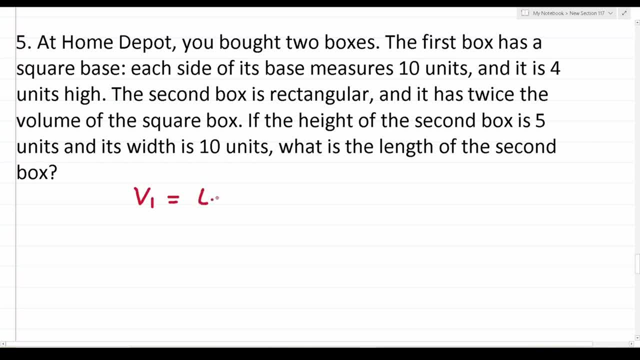 So the volume of one of our rectangular prisms is going to be length times width times height, And the volume of our other rectangular prism is going to be length times width times height. And let's see what information we're given about these rectangular prisms. 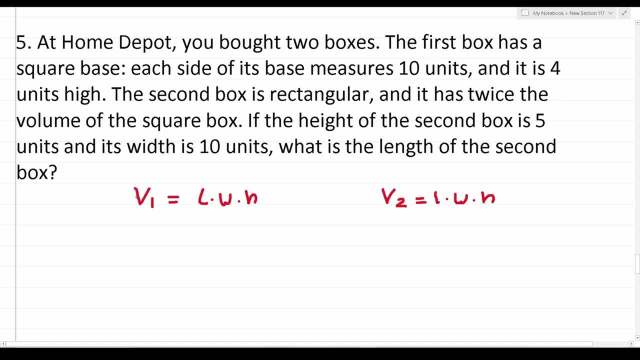 This first rectangular prism which is over here- This is the volume of the first box- has a square base. Each of its, each side of its base, measures ten units. So the length and the width of the base of this box is going to be ten. 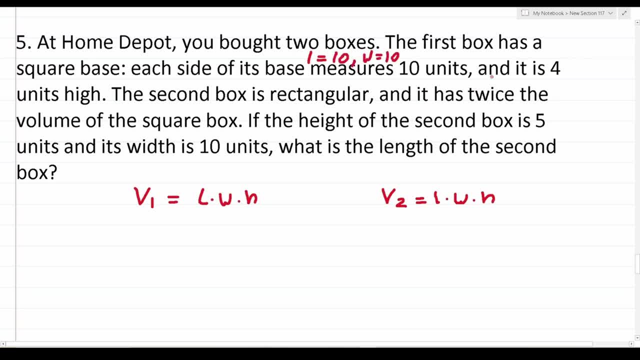 So length and width is ten, And it is four units High, So H is four. Let's go ahead and plug that in. accordingly. This becomes ten times ten times four. Ten times ten is one hundred. One hundred times four is four hundred. 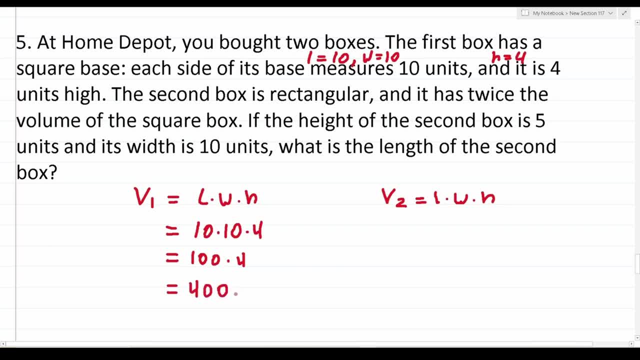 So the volume of this first box is four hundred and it just says units. So this is units cubed. All right, So we found the volume of our first box. It has twice the volume. Our second box is rectangular and it has twice the volume of the square box. 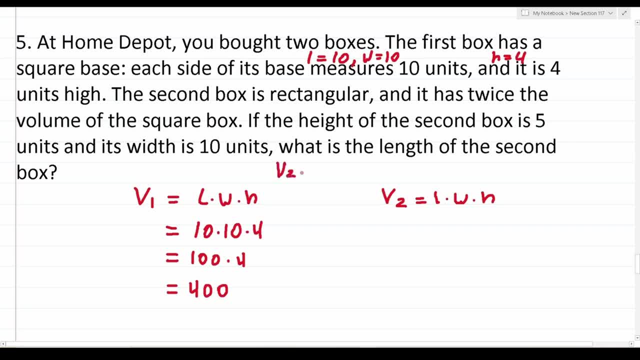 So volume two is going to be twice the volume of the first box. All right, Well, we can actually figure that out. What is the volume of the first box? It's right here It's four hundred. So this becomes two times four hundred. 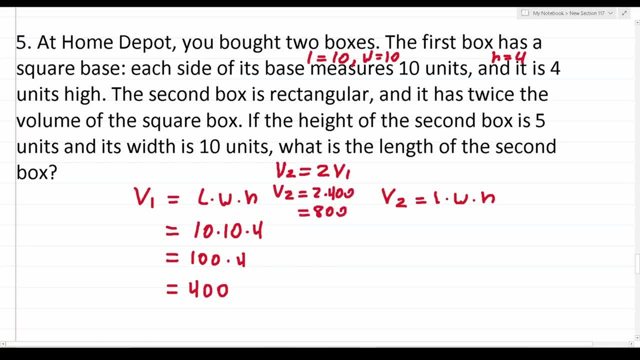 Two times four hundred is eight hundred, So the volume of our second box is going to be eight hundred. It has a height. If the height of the second box is five units, So H is five, and its width is ten units, So W is ten. 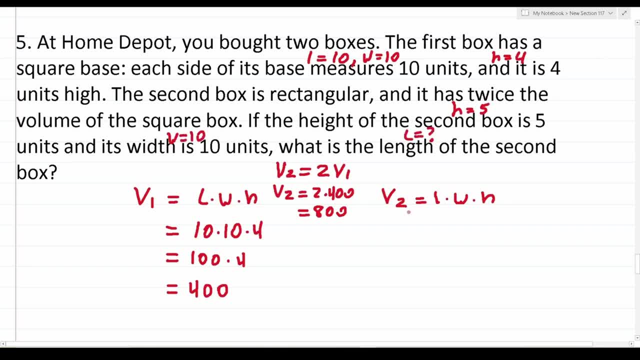 What is its length? So that's unknown. So let's go ahead and plug these things in. We know the volume of our rectangular box is going to be eight hundred. We know its length is what we're trying to figure out. Its width is ten and its height is. 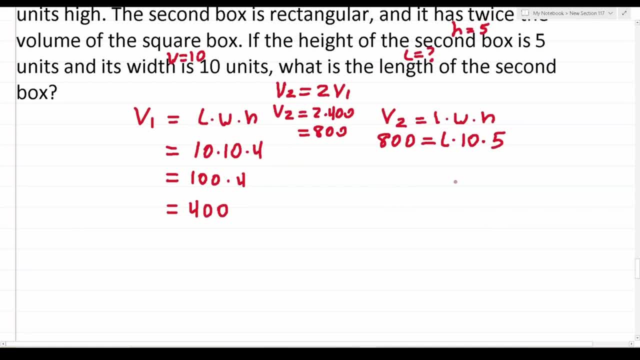 five. So clearly we're going to be solving for L in this case, And that's actually pretty easy to do. This becomes ten times five, which is fifty. So this is fifty. L equals eight hundred. Let's divide both sides by fifty to get L by itself. 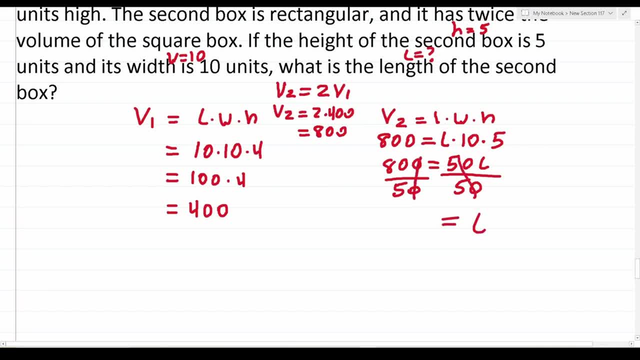 This crosses out here, leaving you with just L. We can cross out these corresponding zeros And now we're left with eighty divided by five, which I know many of you can do in your head. but let's go ahead and work it out. 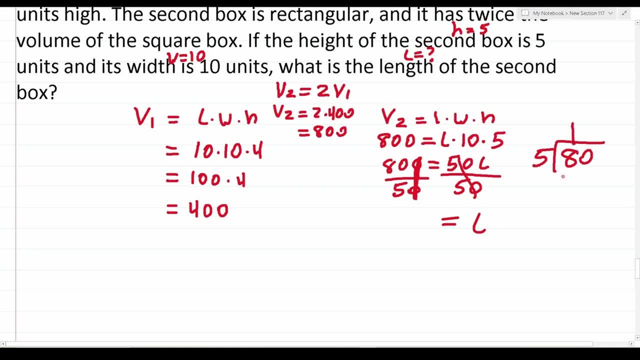 Five goes into eight. one time Five times one is five. Eight minus five is three. Drop down this zero Five times six is thirty. Thirty minus thirty is zero. So the length of this rectangular box is sixteen And of course that's sixteen units. 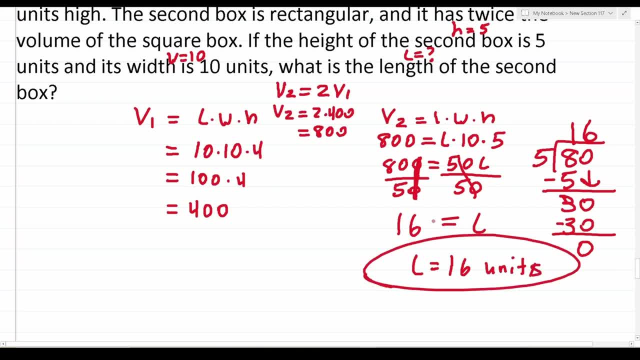 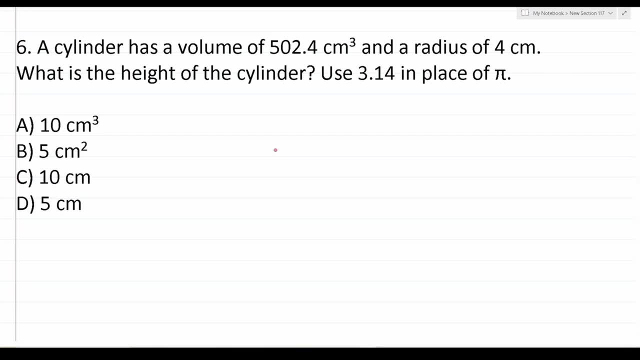 Given a unit of measurement. So the answer to this one is sixteen. All right, So number six says a cylinder has a volume of five hundred two point four centimeters cubed and a radius of four centimeters. What is the height of the cylinder? 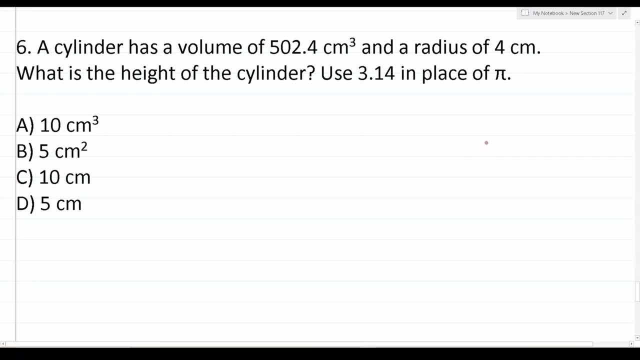 Use three point one, four in place of pi. All right, So we are working with a cylinder here. So if it's helpful and you can't visualize what we're doing, you can quickly make a sketch of a cylinder here. Let me draw that line a little bit better for you. 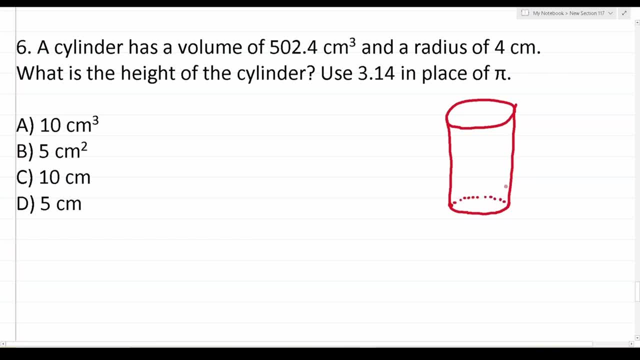 More specifically, we're finding the volume of a cylinder, and you should recall my definition of volume: Volume is the area of the base, times the height of the figure. Well, a cylinder has a base that's in the shape of a circle. 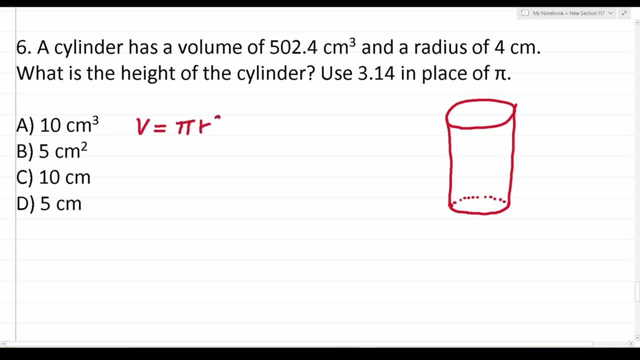 So the area of a circle is pi r squared And of course I just said you multiply the area of the base times the height. So that's the formula to find the volume of a cylinder. We can label the rest of this if we want, but it's not really necessary. 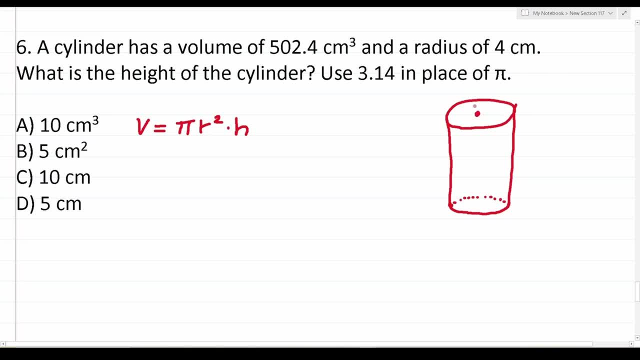 We know this cylinder has a radius of Radius of four and a height That is Unknown, So we'll leave that as H. So let's get back to the problem, now that we've derived our formula. just by looking at our figure, we know this cylinder has a volume of 502.4.. 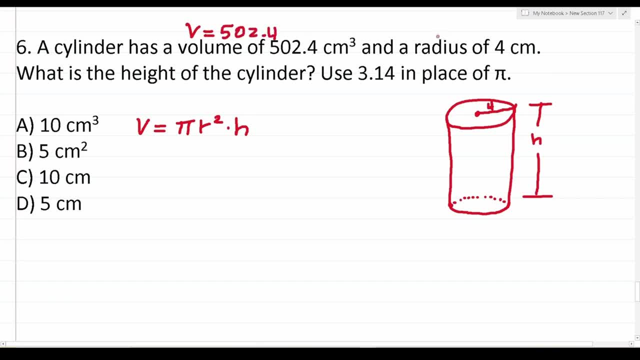 So our V is 502.4.. Our radius, or R, is four, and we don't know what its height is. So we're ultimately going to be solving for H. So let's start plugging those things in. We're told our volume is 502.4. 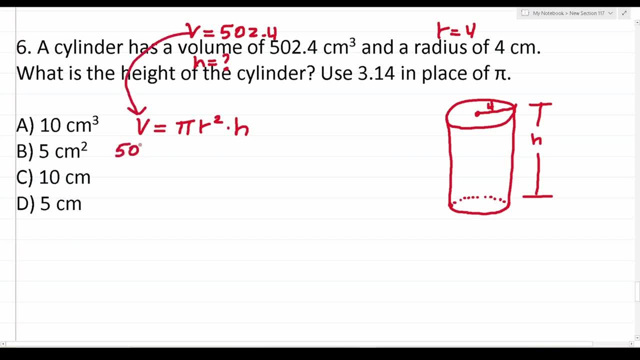 So in place of V, we'll go ahead and put 502.4.. We were told to let pi be 3.14.. So this is going to become 3.14.. Our radius is right here It's four. This is four squared and our height's unknown. 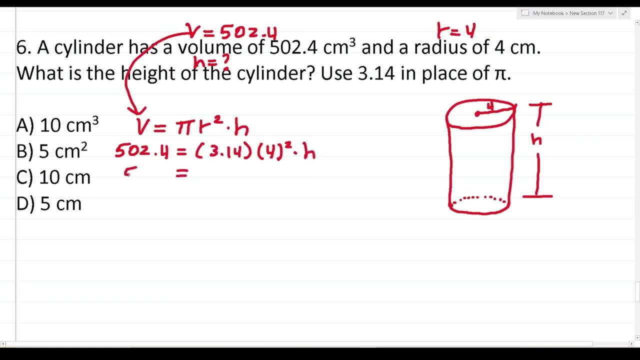 So we'll leave that as H. Let's keep working this out. This is 502.4.. Four squared is 16.. So this becomes 16 times 3.14 times H, And I'm going to work this out off to the side so as not to make any mistakes there. 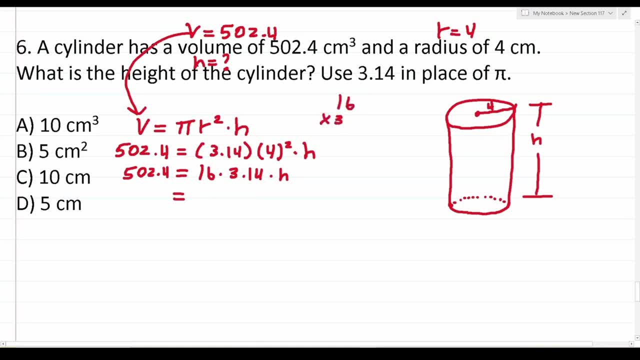 We have 16 times 3.14.. Well, as you can see, we're multiplying a whole number, notably 16, by a decimal, notably 3.14.. So what you want to do is take your decimal and shift it one, two times to the right. 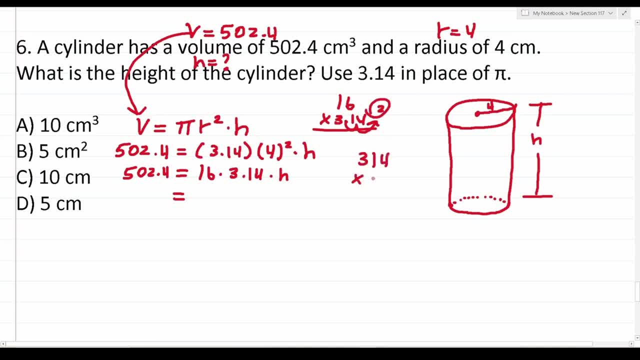 Rewrite this as 314 times 16,, albeit with no decimals, And once we do this, we're going to take the two decimals that we shifted to the right here and we'll shift them to the left in our answer. So let's work this out. 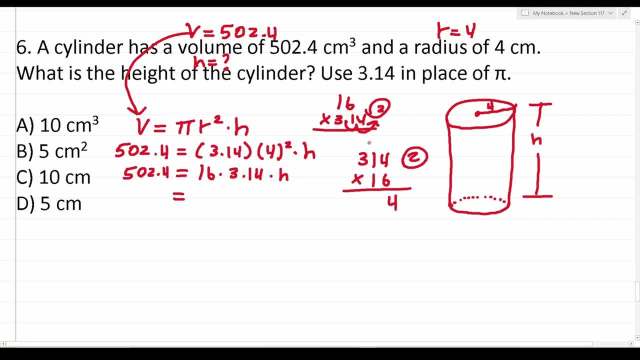 Six times four is 24.. So drop down a four, carry a two. Six times one is six plus two is eight. Six times three is 18.. Before we start the multiplication with this one, we have to bring in a zero placeholder. 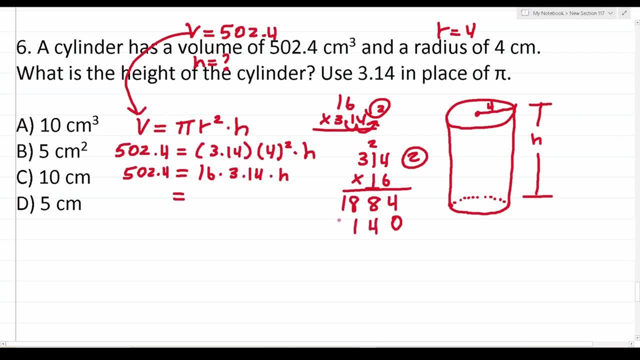 One times four is four, One times one is one, One times three is three. Let's add these together now. Four plus zero is four. Eight plus four is eight, nine, ten, eleven, twelve. So bring down a two, carry a one. 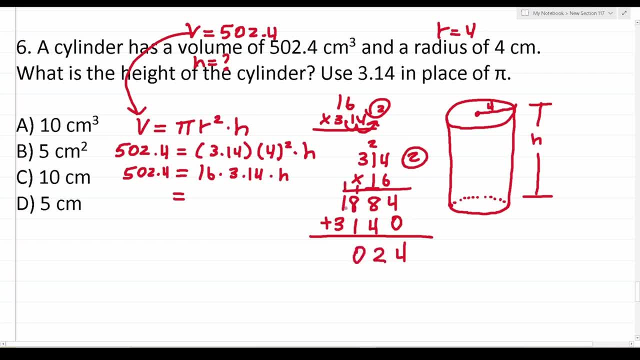 Eight plus one is nine, plus one is ten. So bring down a zero, carry a one. Three plus two is five. Bring our two decimals back into the left, One, two, So this becomes fifty point twenty four. H equals five. 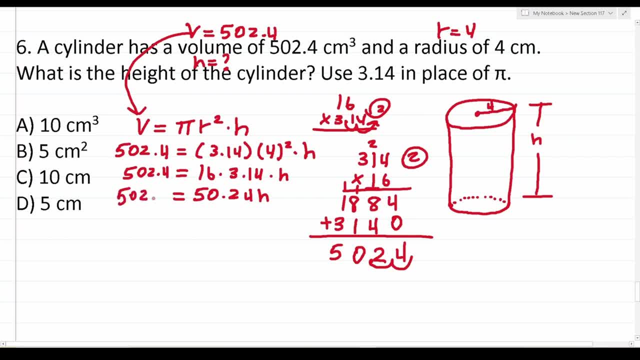 My pen will let me write it Five, oh two, point four. And now we're just going to divide both sides by fifty. point twenty four, To get H by itself. This crosses out here, leaving you with H on this side. And now we got to work this out. 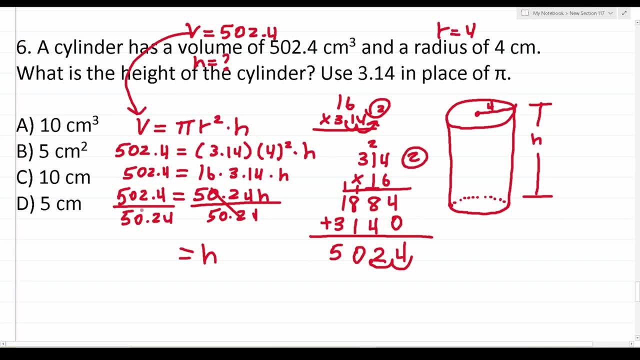 And this one should be pretty easy to do: Five, oh two point four divided by fifty point twenty four. Well, you should know that that's going to be ten, So H in this case is ten. All right, So that is that one. 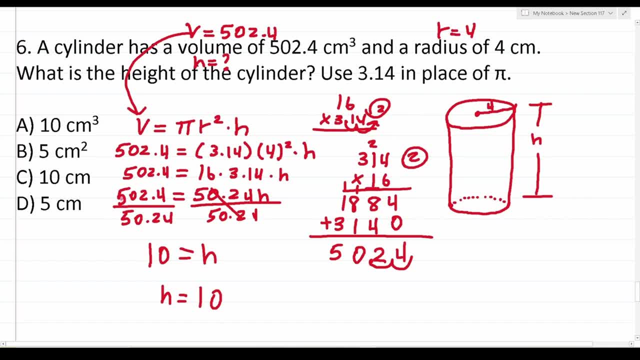 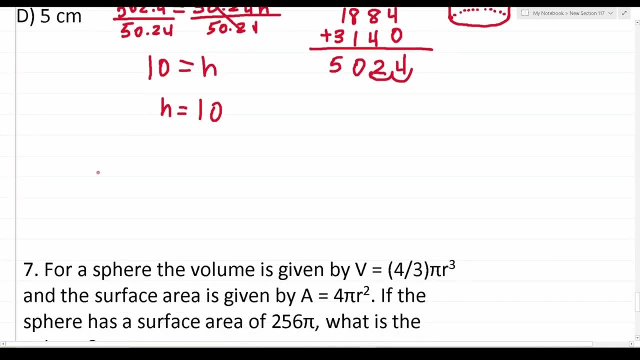 I would work this out for you, but you should see: five oh two point four divided by fifty point two, four is just ten. if you multiply fifty point two, four by ten, You'll get five oh two point four. All right, So the correct answer to this one is C, ten centimeters. 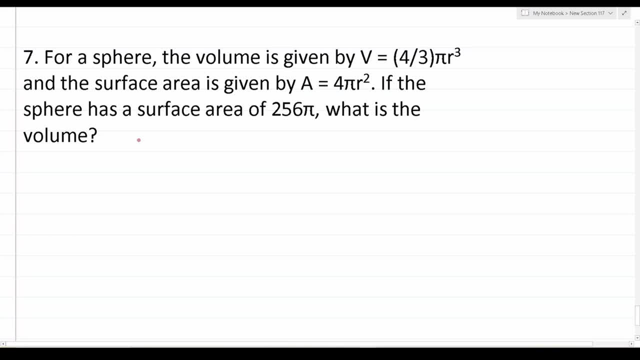 All right. number seven says for a sphere the volume is given by volume equals four thirds pi r cubed, And the surface area is given by area equals four pi r squared. If the sphere has a surface area of two hundred fifty six pi, what is the volume? 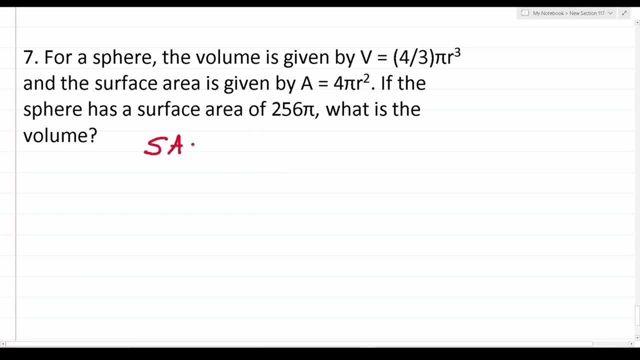 All right. So we're going to start with surface area, And we know that formula. The formula, because it was given to us in the problem, is four pi r squared. What's more, we were told that the surface area, our SA, was two hundred and fifty six pi. 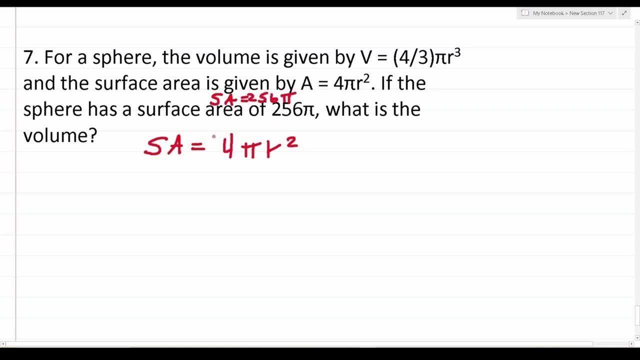 All right, So let's go ahead and think about what we're going to have to do to solve this one. We want to know the volume of this sphere, So that's going to be. volume equals four thirds pi r cubed. What are we missing to find the volume of this sphere? 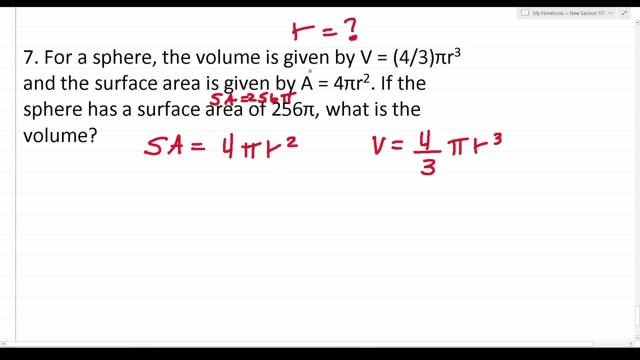 Well, we're missing r. We don't know what r is, And that is the only thing that we have to plug in here to find the volume of this sphere. That said, we're going to use this information given about surface area to figure out what r is, and then, ultimately, we'll be able to find. 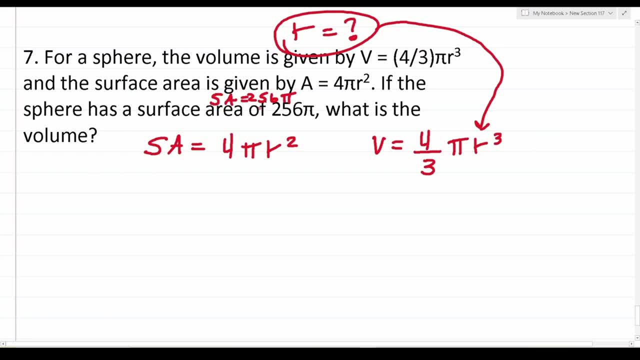 its volume. So again, SA is two hundred and fifty six pi. So in place of SA over here I'm going to put two fifty six pi equals four pi r squared. All right, So we're going to be solving for r here. 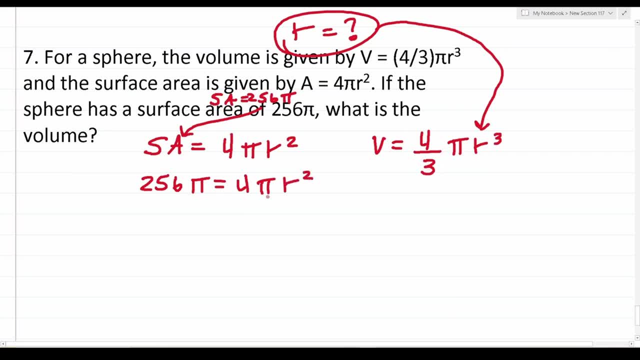 which is going to enable us to find the volume of this sphere. So let's go ahead and divide both sides by four pi to get r squared. by itself, This crosses out here, leaving you with r squared over there. And what happens here? 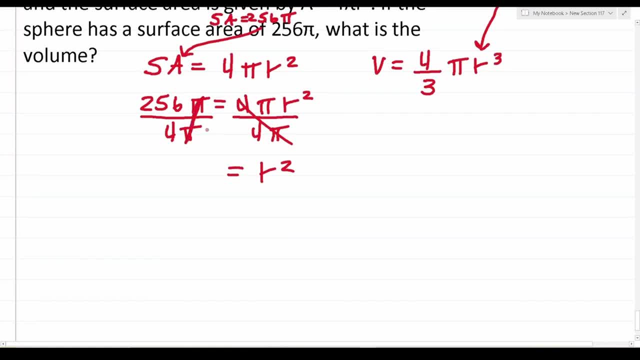 This pi crosses out right here And now. we can do this. Two, fifty six divided by four. We ask ourselves: how many times does four go into two? It doesn't. How many times does four go into twenty five without going over? 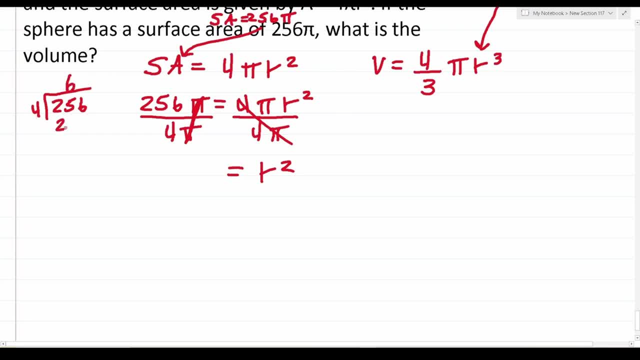 It's going to be six times Six times four is twenty four. Twenty five minus twenty four is one Drop down to six. How many times does four go into sixteen? That's going to be four times Four times four is sixteen. 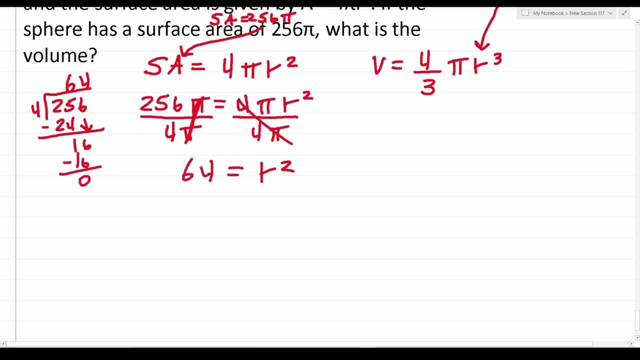 So there is no remainder. So this becomes sixty four equals r squared. We just want r, So we're going to take the square root of both sides, get r. by itself, This becomes r equals the square root of sixty four, which is eight. 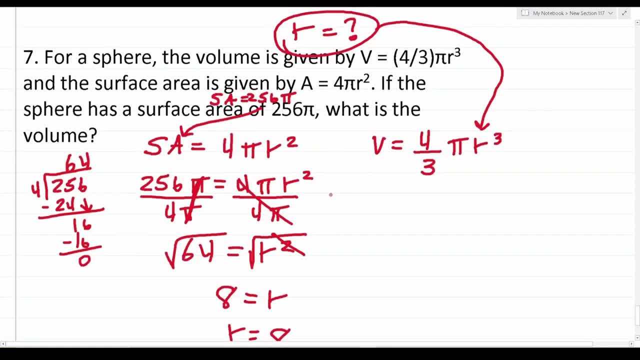 So r is eight. Now that we know r is eight, we can go ahead and plug it in here and figure out what the volume of this sphere is. So this becomes: volume equals four thirds pi, And that's going to be eight cubed. 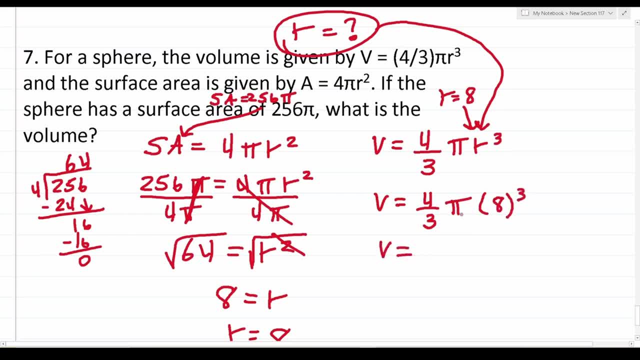 All right. So volume equals four thirds times pi times eight cubed. Eight cubed is the same thing as this. It's eight cubed is eight times eight times eight. Eight times eight is sixty four. What is sixty four times eight. 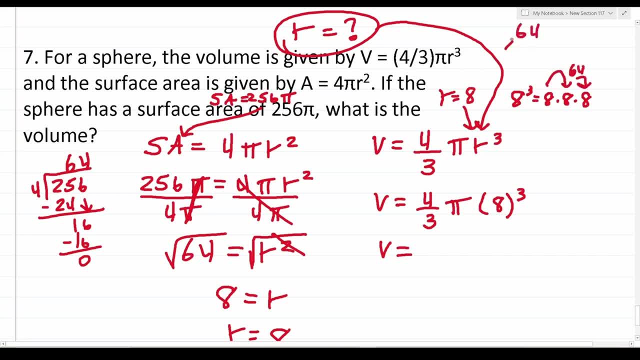 So it's not to make a mistake, I'm going to do that. off to the side, We have sixty four times eight. Four times eight is thirty two. So drop down a two, carry a three. Six times eight is forty eight, forty nine, fifty, fifty one. 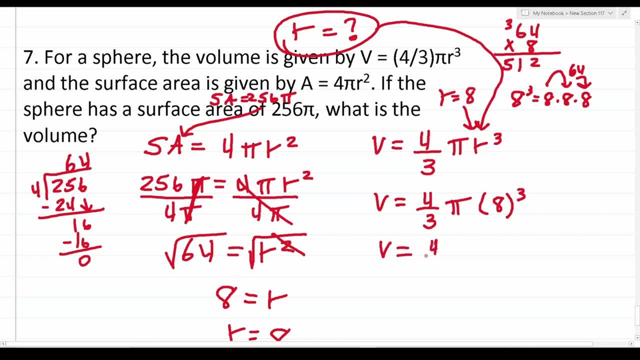 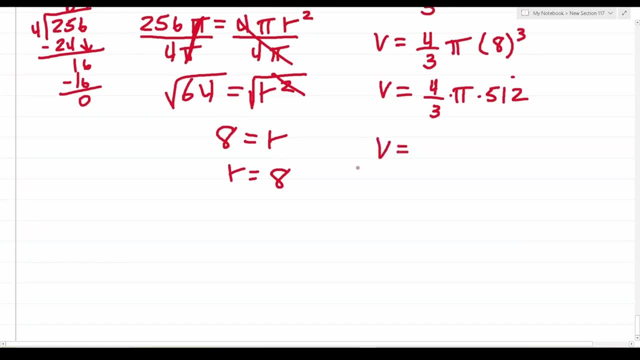 So this is five hundred and twelve. This becomes four thirds times pi, times five hundred and twelve. So let's go ahead and work on simplifying this. So we're going to do this off to the side. We can do four thirds times five hundred and twelve off to the side, like this: 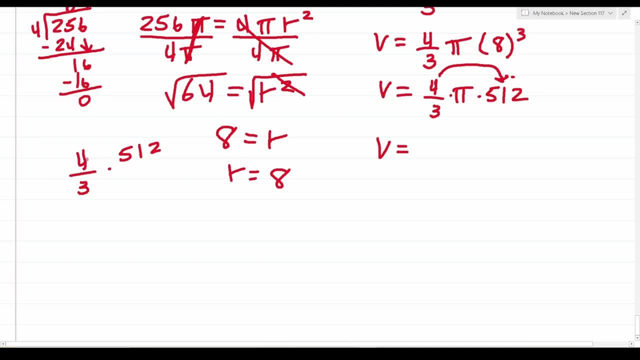 And again we can regard this like this: Four over three times five hundred and twelve over one. You can write any whole number as a fraction by placing it over one, which means we're going to do this, we're going to multiply straight. 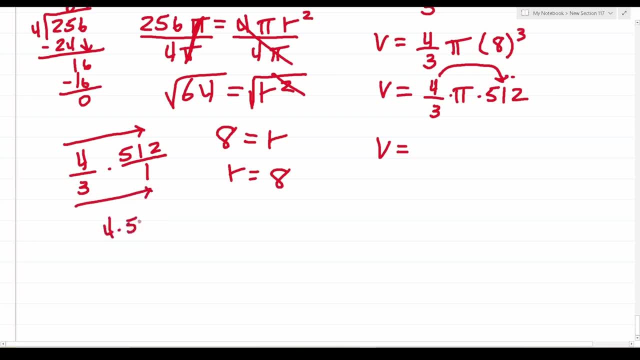 Across, such that this becomes four times five hundred and twelve, over three times one. Three times one is just three. So we can go ahead and work that out very quickly. Let's do five hundred and twelve times four. Now, two times four is eight.